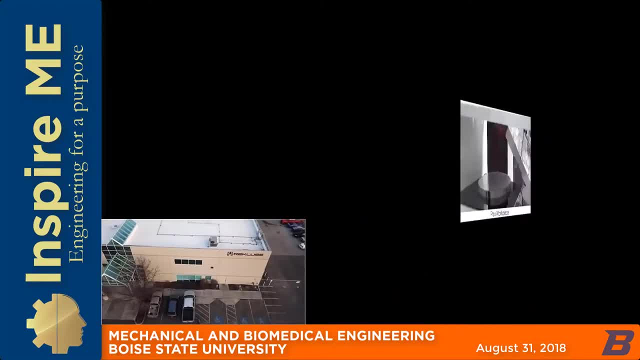 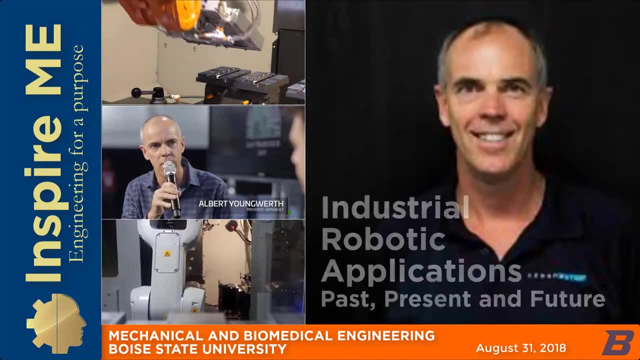 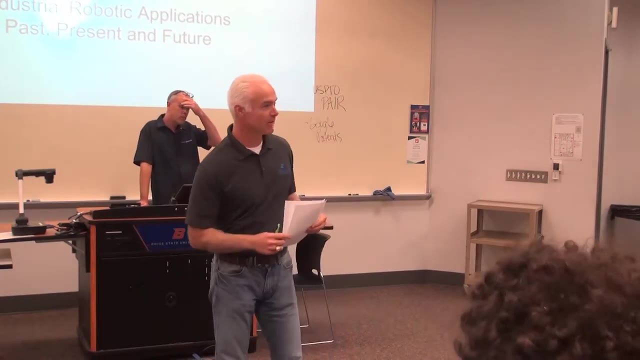 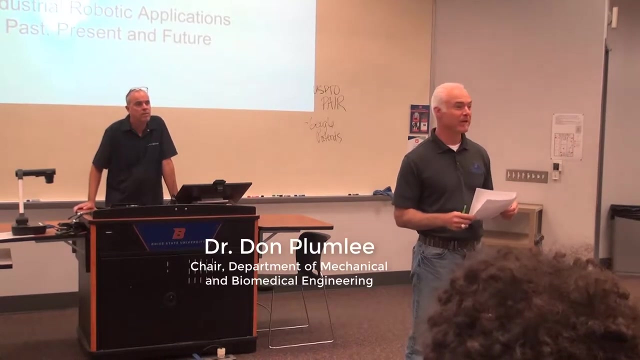 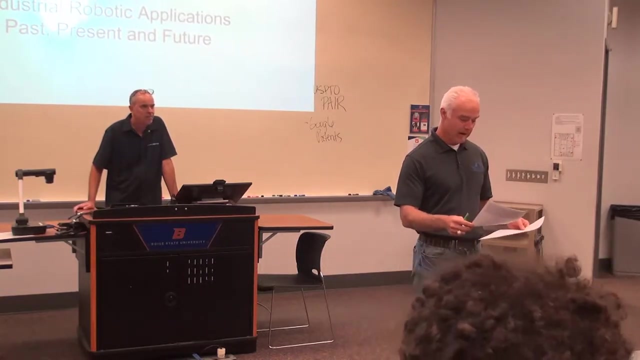 Welcome to our Friday seminar. Inspire Me- our mechanical engineering seminar. Again, I'm Don Plumlee, Glad for everyone to be here. I'm really excited for our topic today. Before we get started, I had a couple of announcements. We do have a sign-up sheet that some of you have already signed. 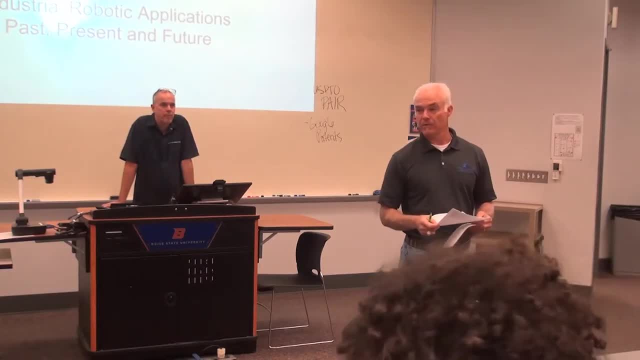 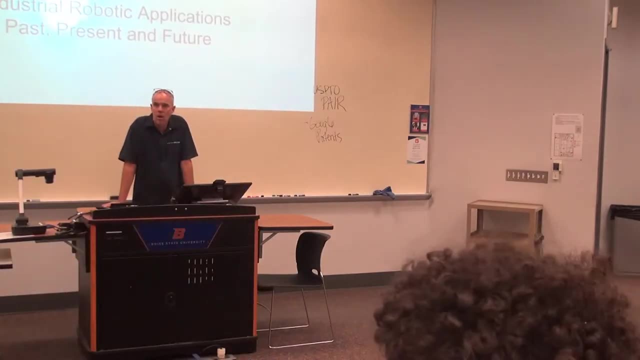 and we want to make sure everybody gets on here, so I'm going to pass it around. Make sure that you get your name on that. Have you signed yet? Okay, I'll get you. First of all, make sure you get on there and keep the pin, if you would. 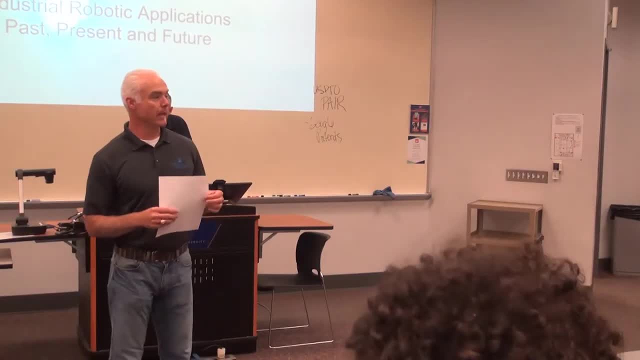 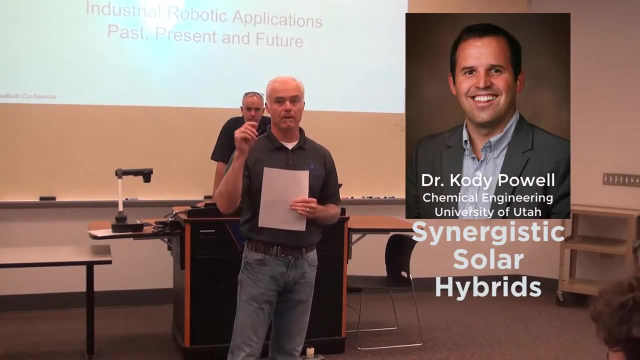 And then pass it around, Make sure everybody gets a chance to get on it. And then the next week- this time next week- we're also going to have a speaker from the University of Utah. He's going to talk about synergistic heat systems. 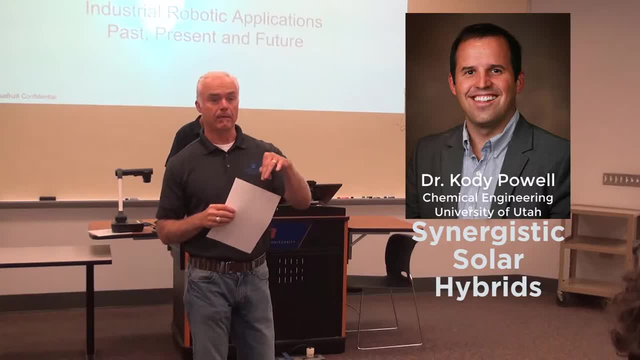 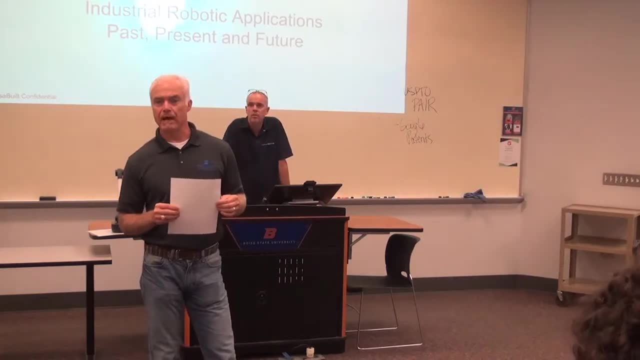 So this person worked with Dean Leidy, who's now our dean here, back whenever she was at Utah, So it should be an interesting topic as well. I believe he's a faculty member in chemical engineering, Chemical engineering, Chemical engineering- Yeah, I'm there, So that'll be a good one. 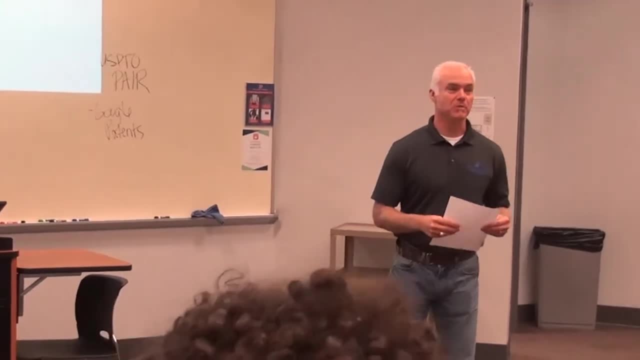 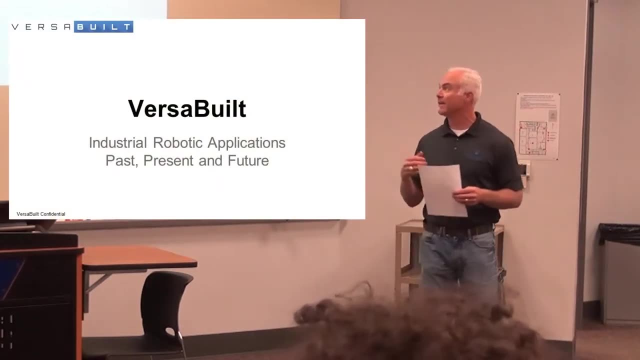 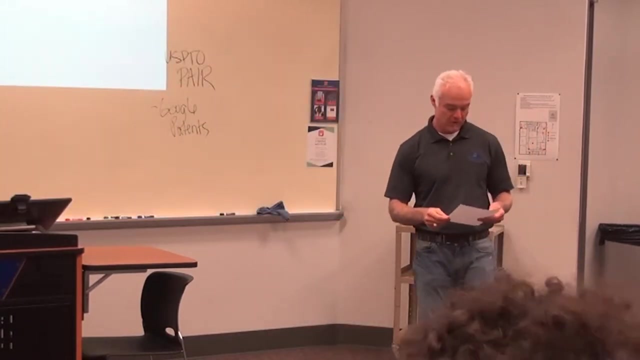 Okay, so today we have a special speaker here from locally in Boise We have Al Youngworth, who's the CEO of VersaBuild Robotics And, as you can see there, he has a master's degree from the Cal State University, Chico, in computer science. 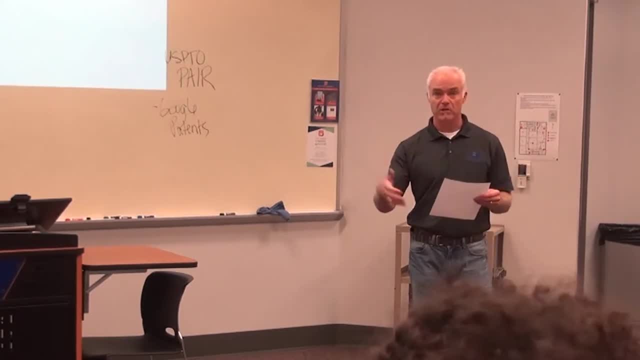 And he's done some work establishing different startups here in Boise See. he founded the Recluse Motorsports and VersaBuild, And he's also held senior level positions at Apex Technology and Extended Systems. So he's got a lot of a wide range of experience, but also very focused. 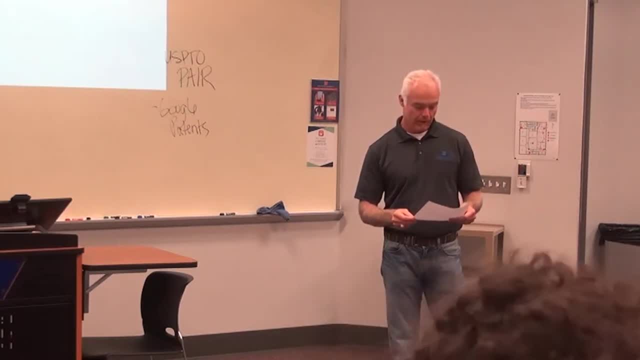 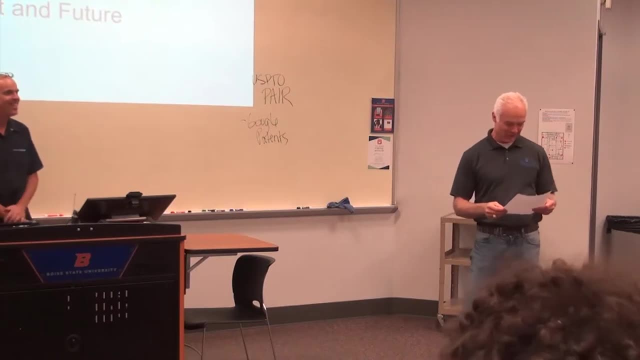 in the Boise area around robotics, So we're excited to have him here Also. just interestingly, I always like to see the. what else is he interested in? So yeah, so when he's not tinkering with robotics or new business opportunities, he likes to fly airplanes. 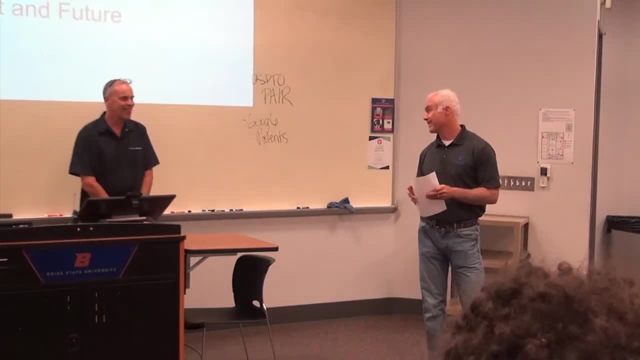 And he's got a newly acquired pilot slot A little over a year. A little over a year, Yeah, Okay. So so he can talk about maybe his robotic or not, so his, his aerobatics- Okay, All right. 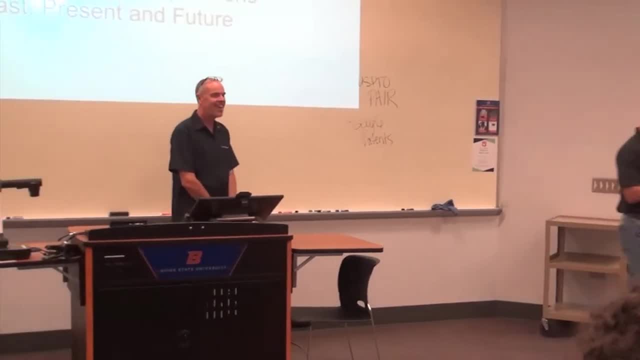 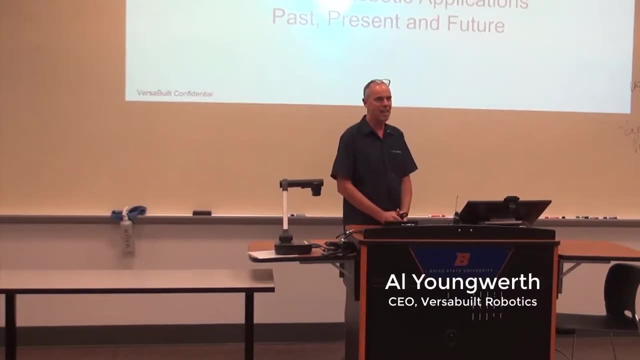 So let's welcome Al Youngworth, please. Well, you know, as I was coming in here, I was thinking about gosh, how long have I been here? When was I last in college? So 30 years ago. I was starting my final semester of college. 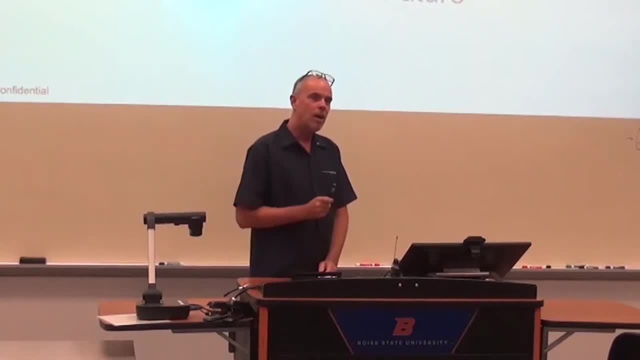 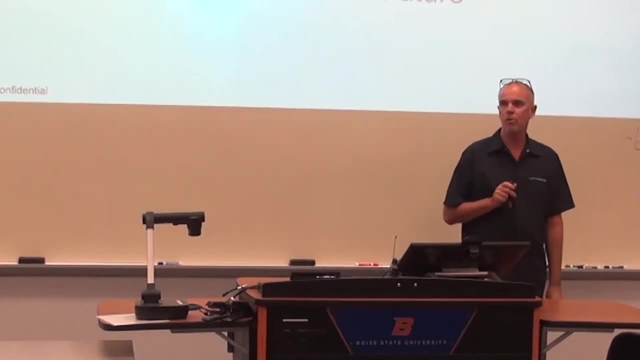 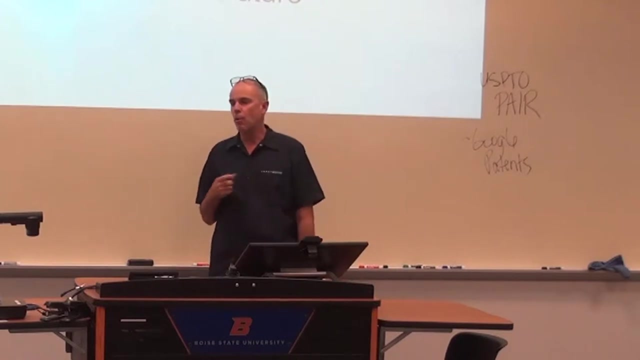 So hard to believe. So I started in the Boise area at a little company called Extended Systems. Most of you probably have not heard of that. That was a company that was a spin-off from Hewlett Packard that made network connectivity devices. 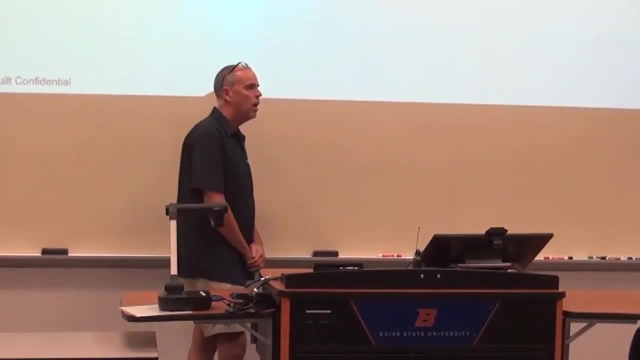 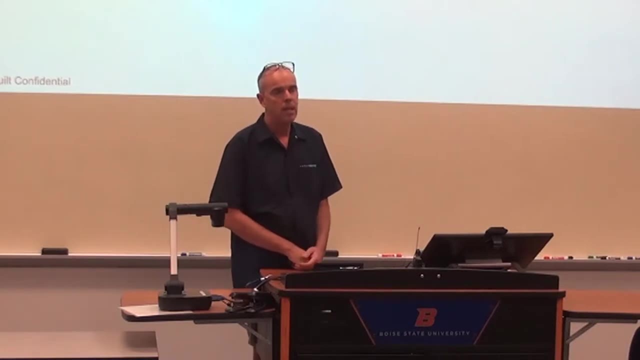 primarily for printers, then moved on to Bluetooth things like that. Then, about 1996, I moved to a start-up company called Apex Technology And we made one of the very- actually very first Linux-based devices. It was a small box that connected a small office to the Internet and provided an Internet connection. 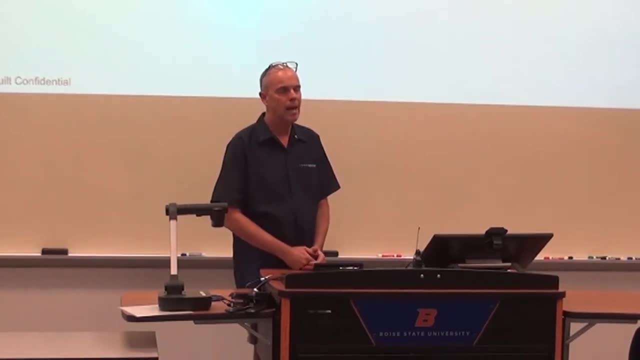 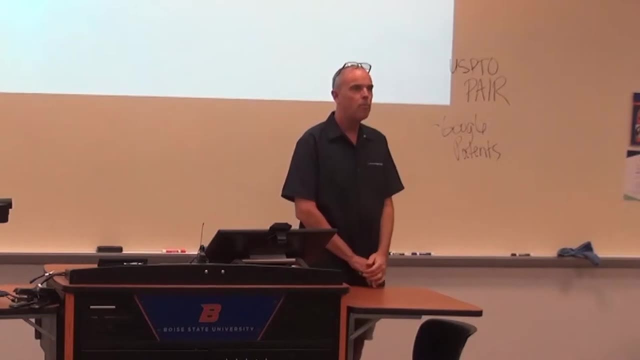 that could be shared- a firewall, a mail server and things like that- And then in 2002, after I'd exited that company- to have a couple of years of consulting. one of the reasons I wanted to come to Idaho was because I really enjoyed dirt biking growing up. 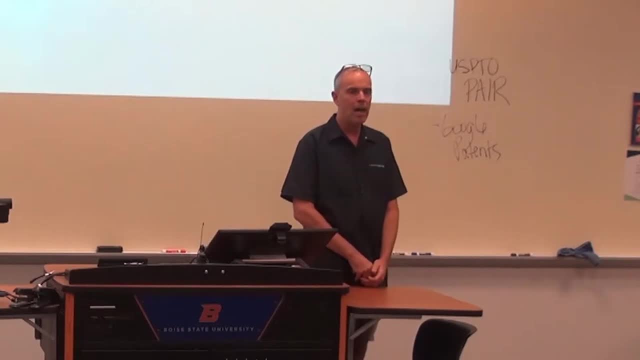 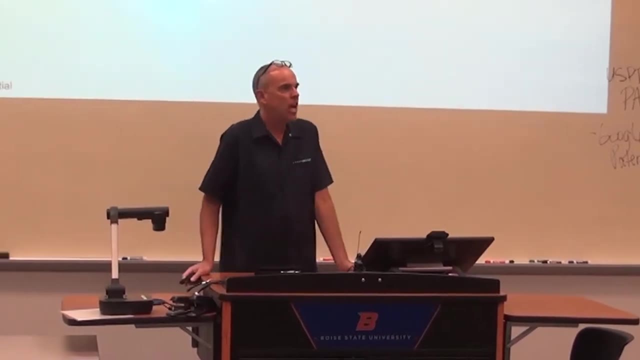 And I heard Idaho was a great place to do that- And I came up with an idea of a new type of motorcycle clutch which was a little bit outside. you know what my educational background was, But I was pretty passionate about motorcycling. 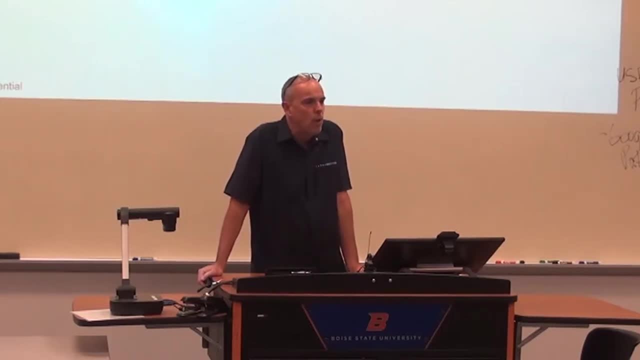 I wanted to try something new So I designed a clutch. I worked with tech help here at VSU- a senior mechanical engineering student, a guy by the name of Sean Brown, back in 2002.. He's now the CEO for his motor sports and built that from starting in my garage to a company. 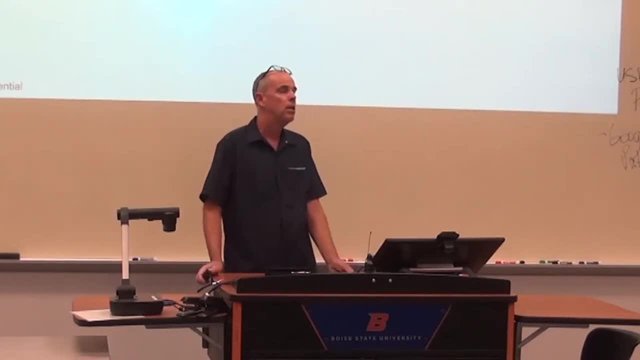 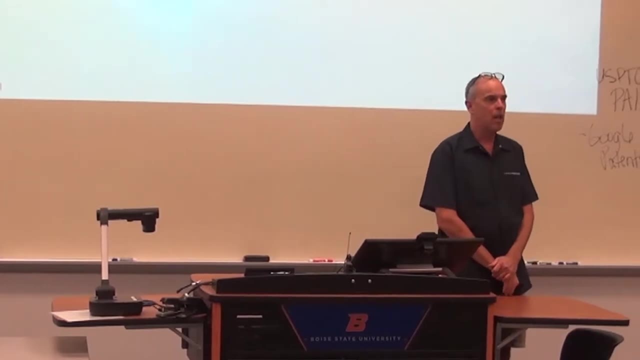 that I think today employs about 70 people, $10 million in revenue, And that was a great experience, So I'm very proud of it. Thank you, I spent a lot of time. you know. one of the things I like to tell people is: you know, 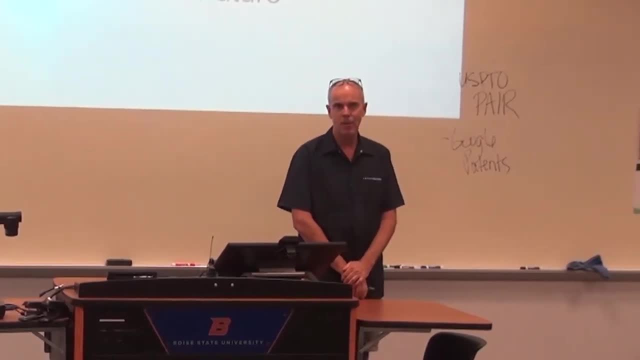 what you're doing here. you're going to learn a lot, But this is just the tip of the iceberg. you know, Learning really begins when you get out of the world, And it's a lot of. it's based on what interests you and what you allow yourself to explore. 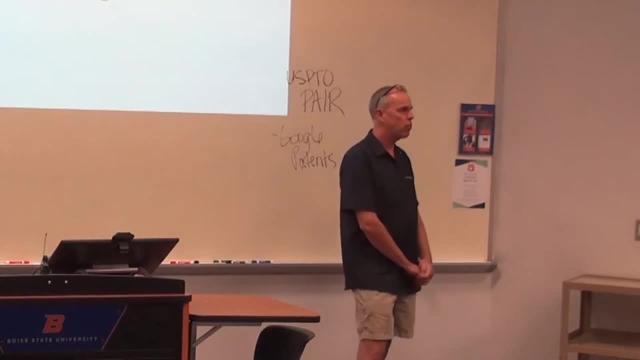 You know, for me, I went from no experience in mechanical engineering, process engineering or robotics and I learned that stuff because I wanted to and I had to be successful. The other thing I think is really important, and you don't necessarily get a whole lot: 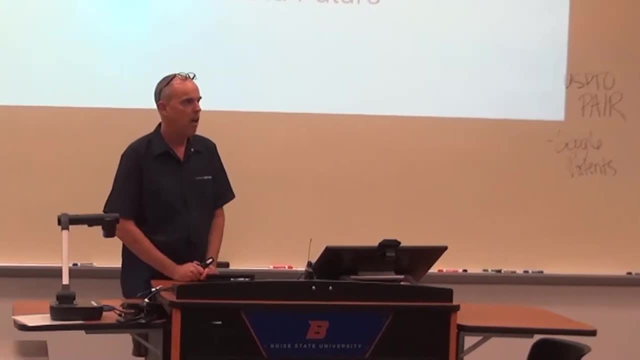 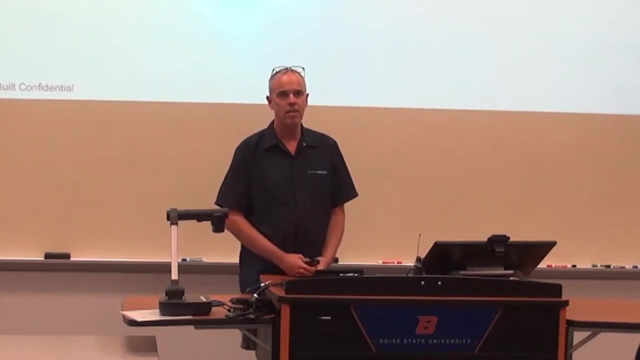 of as an engineering student, is the business side of designing things, the business side of engineering, because that's oftentimes just as important or even more important than the actual engineering. So this isn't going to be a terribly technical discussion about robots. 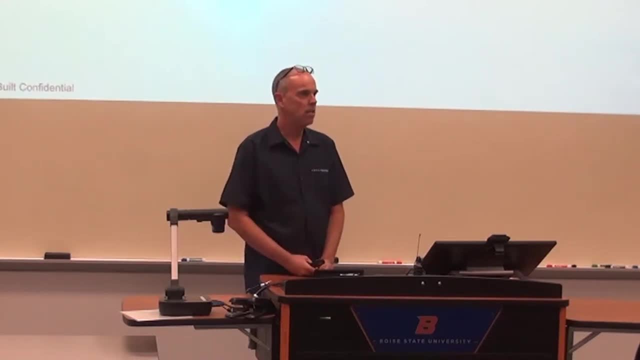 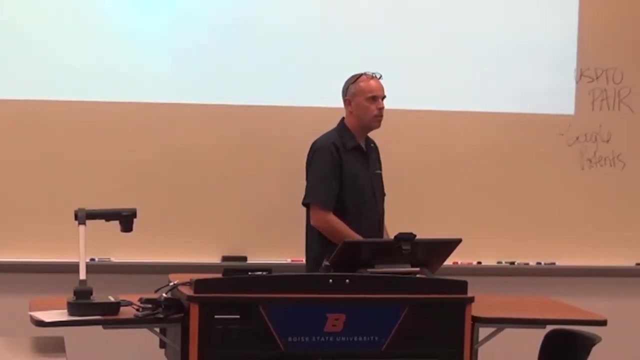 It's going to be more of a market assessment view of robots and kind of how robots, how robots have evolved, where they stand today and where they're going in the future. Now, robots mean a lot of things. I'm sure you guys have all seen the Boston Dynamics Boston. is it Boston Boston something? 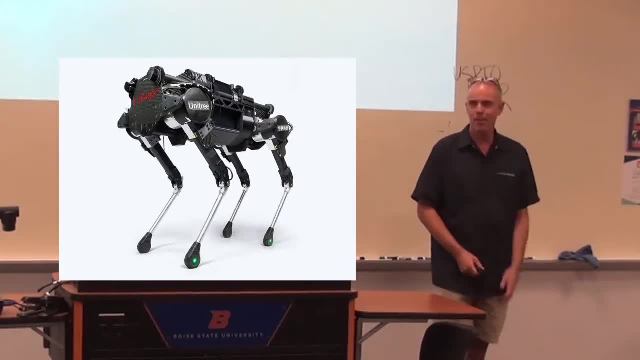 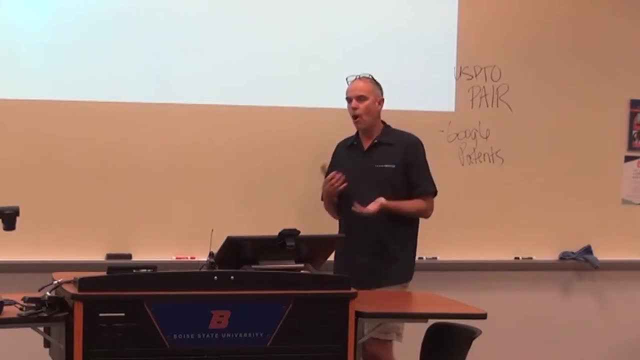 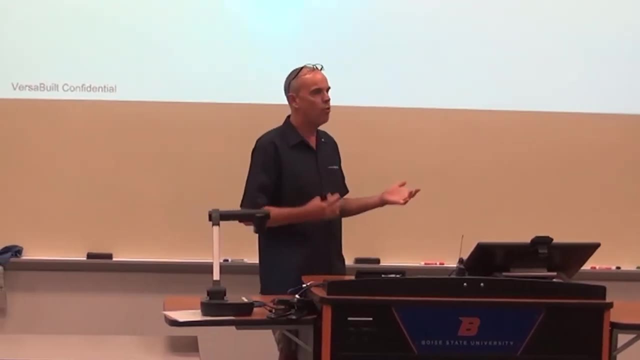 Can anyone help me with that? Yeah, Boston Dynamics. okay, with the robots that look like sheep and things like that. You know those are still R&D projects. They don't yet have a lot of industrial applications. You know, you have your humanoid robots- again same thing. 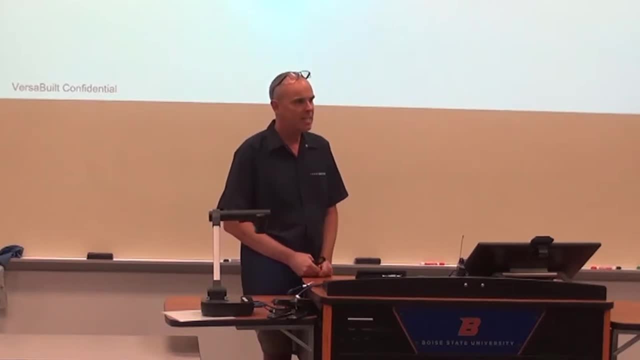 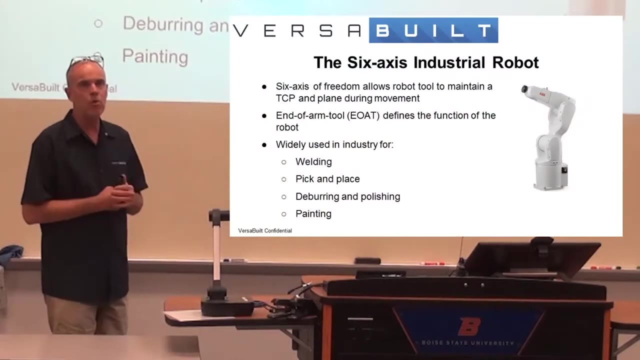 So these are very interesting studies, but that's not what's in the market today. What's in the market today is the six axis industrial robot is the mainstay of industrial automation. Now there's a lot of other different types of robots. 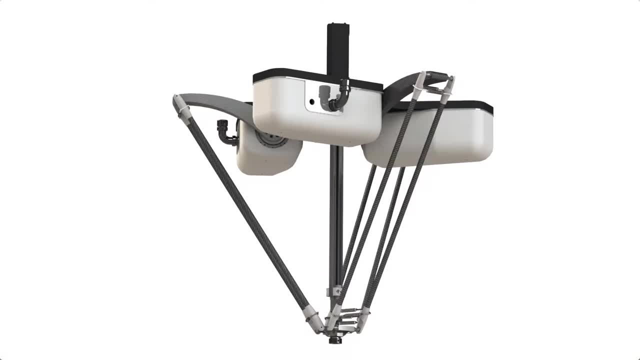 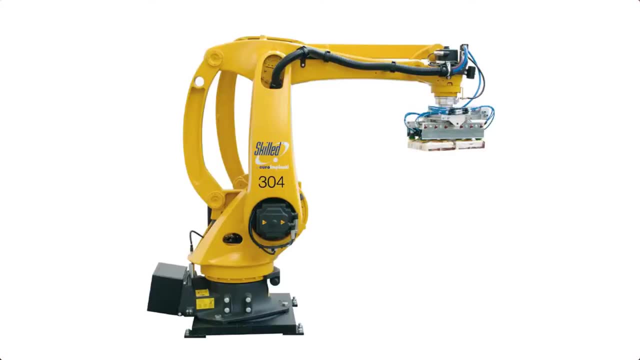 There's delta robots and they kind of look like these spider things. They've got these arms that control and they're generally used for taking place. They're very, very fast. There's four axis robots which look a lot like this, but they have four axes instead of six axes. 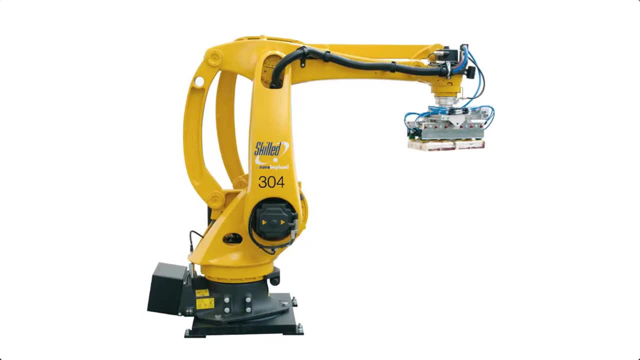 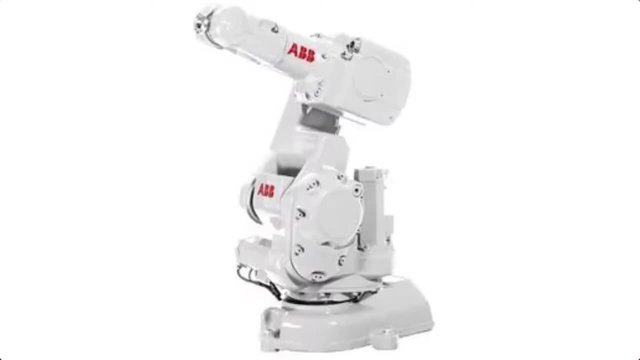 And they can generally rotate. They maintain a single plane for their tool and they can pick up a box and then move it to another location. The six axis industrial robot allows you to find what's called a tool center point. Every robot into that arm is going to have some sort of a tool, and that tool could be a. 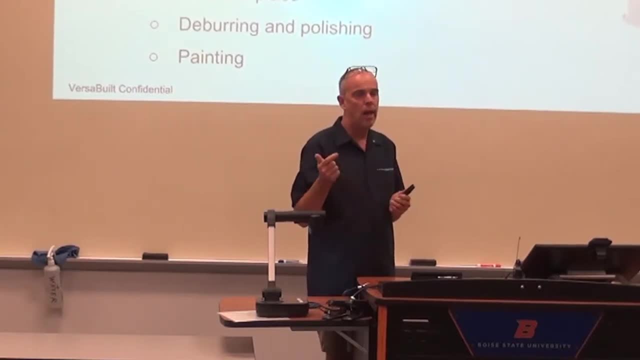 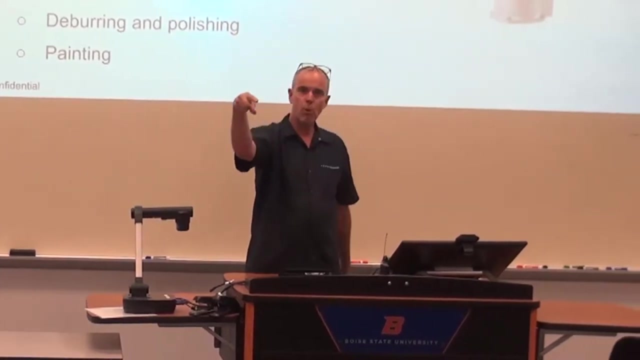 welding torch. it could be a caulking dispenser, it could be a paint gun, it could be some sort of a gripper to pick and place things. But what six axis allows you to do is to find the tool center point and say this is my robot arm and this is the end of my torch, The robot. 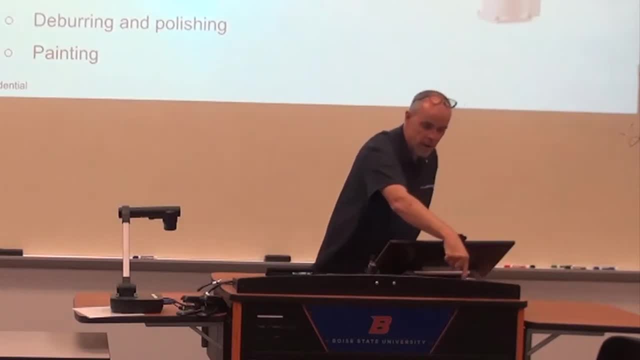 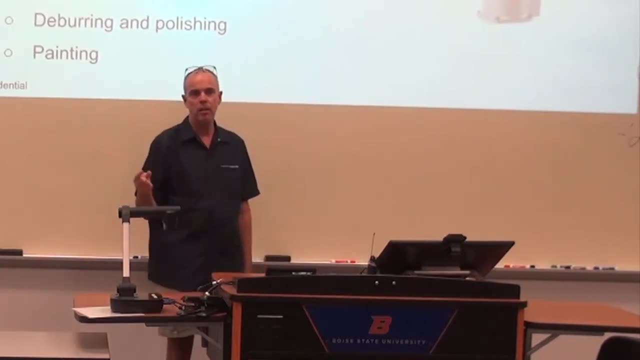 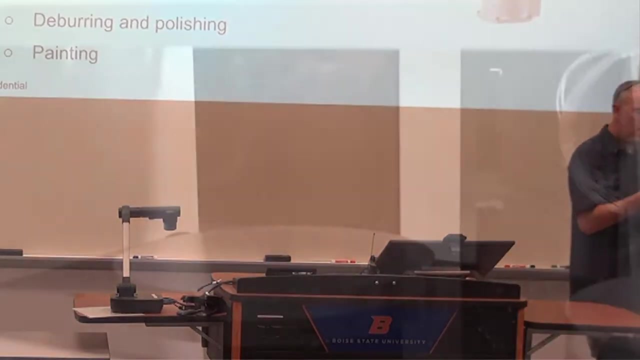 knows where it is and you can program it so it can follow a very, very specific path and maintain that path around different objects. The other thing a robot can do is it can maintain a plane with the tool center point. So imagine the tool center point is the bottom of this. 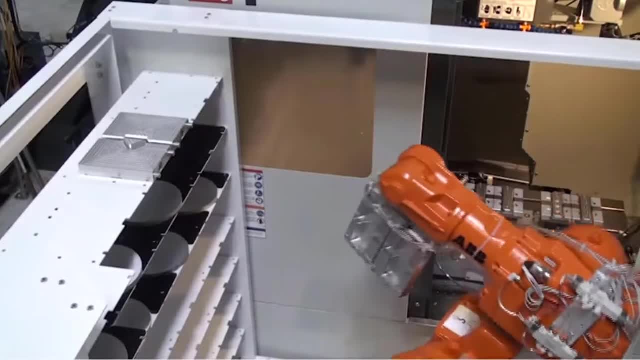 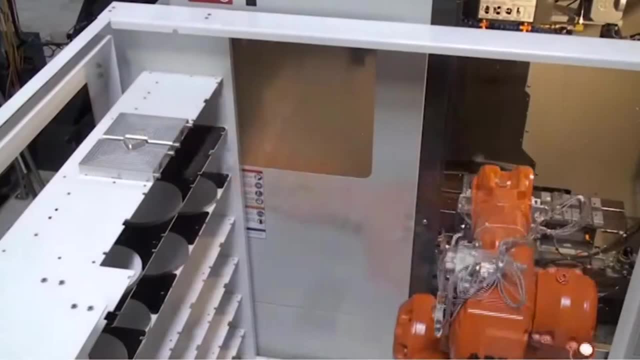 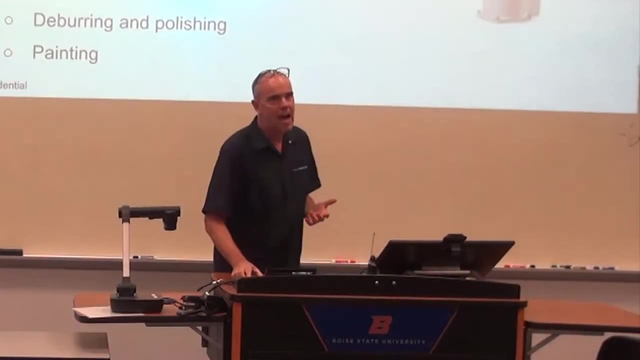 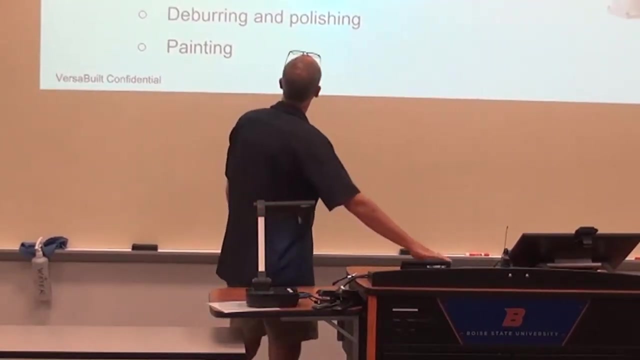 phone. With the six axis industrial robot I can move this around and maintain that plane and that's something my company uses a lot in pick and place applications. So six axes are kind of the minimum number of axes, Six axes necessary to do kind of all the most common types of functions And the most common. 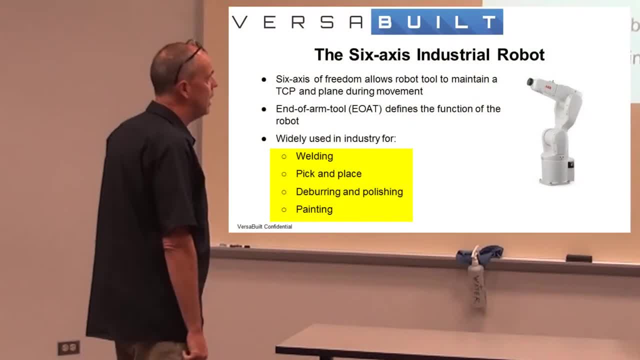 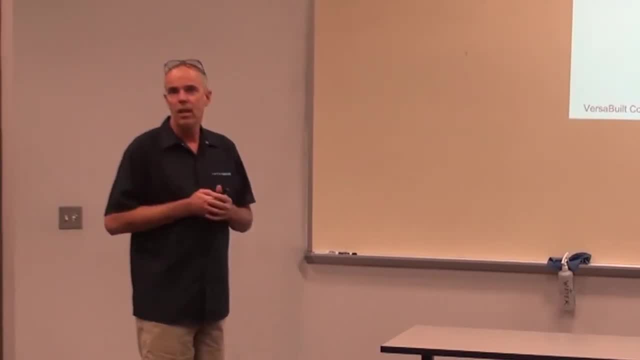 functions in industry today are welding, pick and place, deburring, polishing and painting. Pick and place- that's really, really broad right. It can be picking and placing fruit, it can be stacking boxes or it can be picking up raw material to feed a machine. 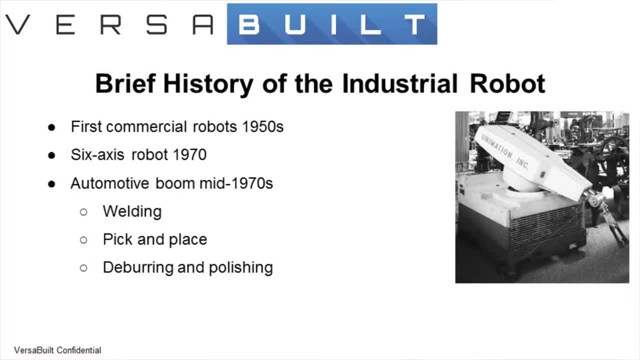 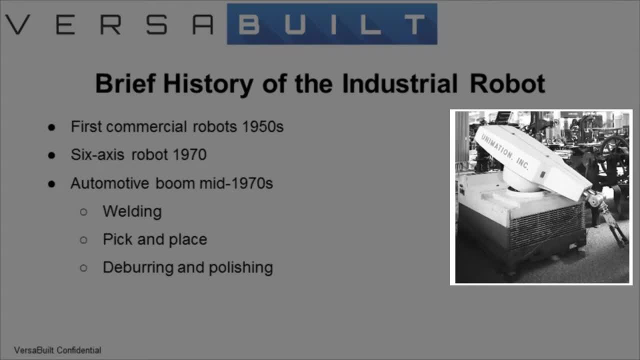 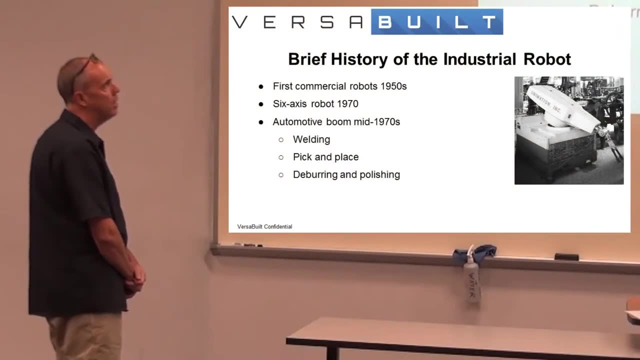 So a brief history. The first commercial robots came out in the 1950s- That's a picture of the Unimation robot- and they actually were used a fair amount in industry in the 50s and 60s. The first real robots, the modern industrial robot ideas, came out in the late 1930s. but the 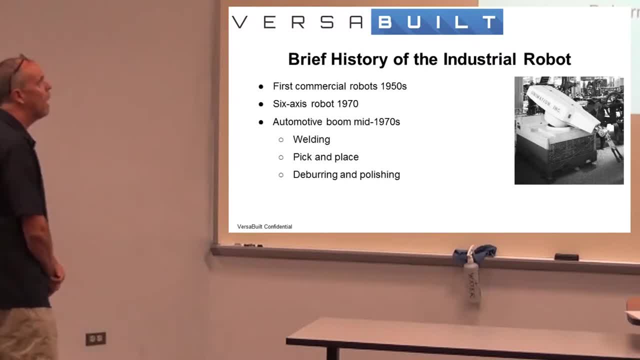 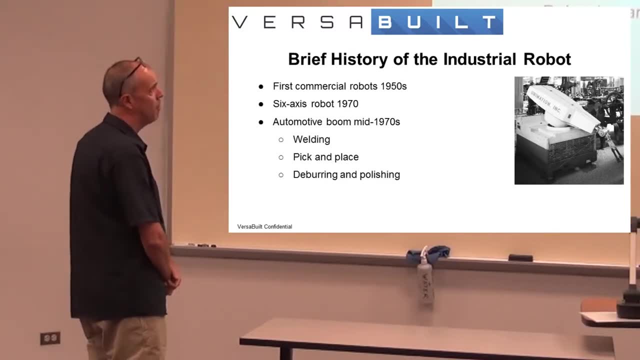 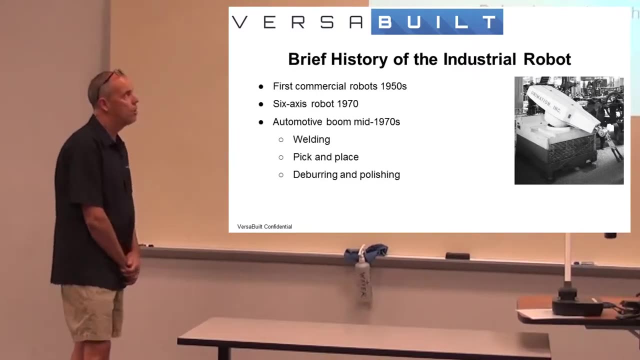 Unimation was really the first commercially one successful robot. The six axis robot, I believe, was invented in 1969. It became commercially viable about 1970. But what really drove robots to where they are today was the automotive market. I'm sure you guys have all seen pictures and videos of robots used. 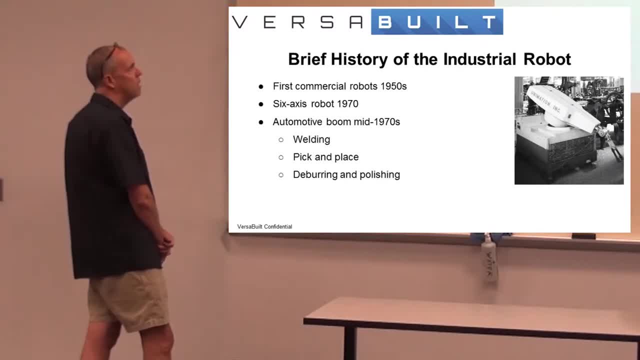 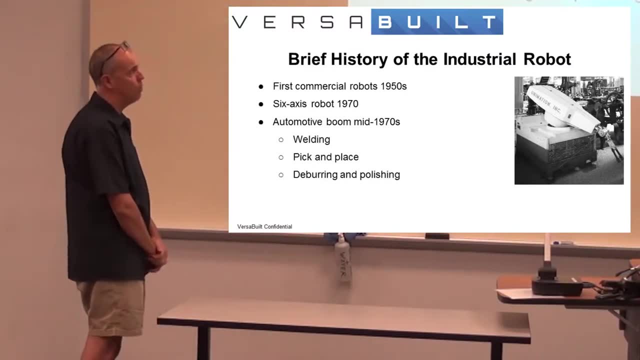 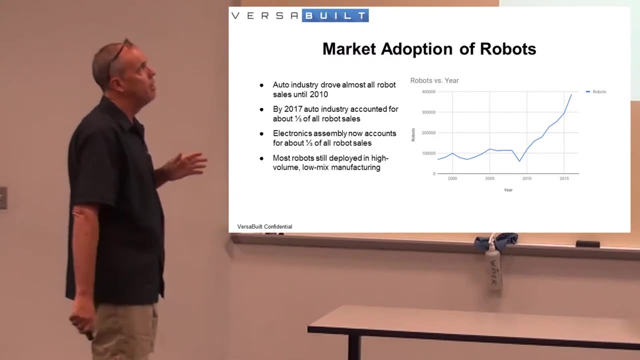 in the automotive market, But they're widely used in welding. making a place to bring in polishing Painting is the other thing that's really big with robots and automotives. So if we look at the market adoption rate of robots over the years and I think this- 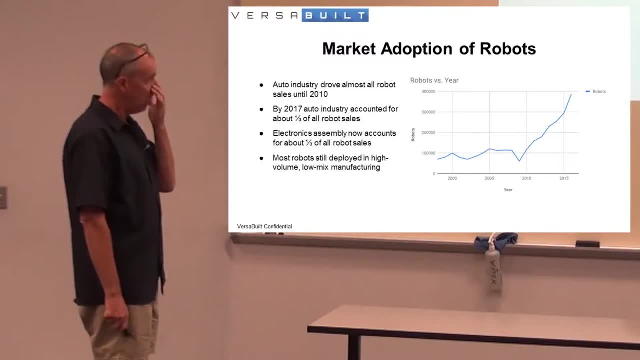 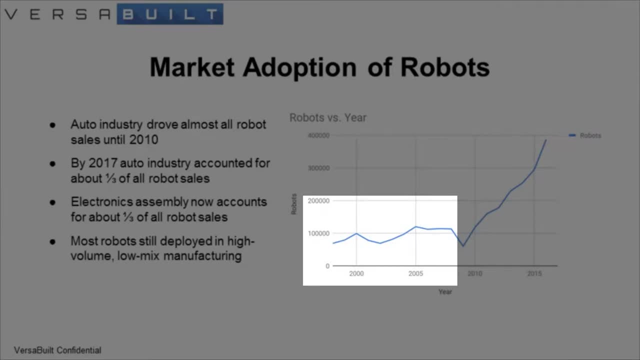 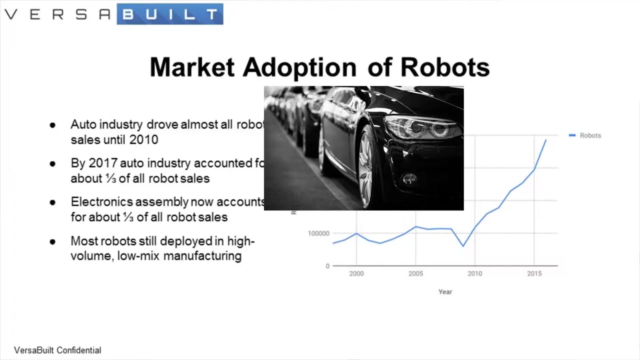 data goes back to about 1996 or so. the curve is pretty flat through this area And really what you're seeing here is kind of the ups and the downs of the automotive cycle. You know, something like 80%, 90% of all industrial robots up until about mid-2000s- like 2007,, 2008,- were going into 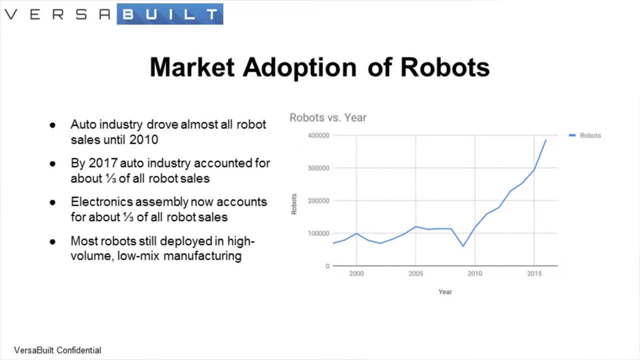 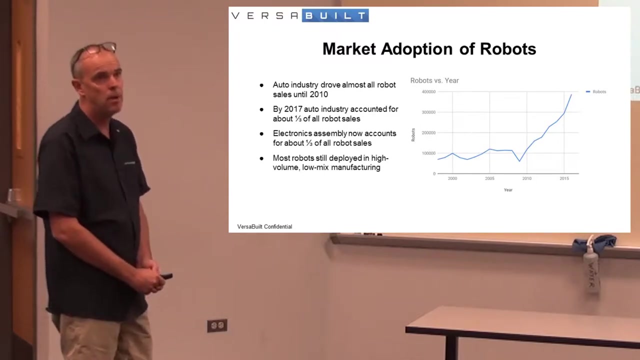 automotive applications. And then you see this big dip here during the recession where the automotive industry really shut down. And then what you see here in this steady- you know, increasingly steep curve here is robots moving into other applications, other industries. The biggest driver there is the electronic assembly. The iPhone has had a big impact. 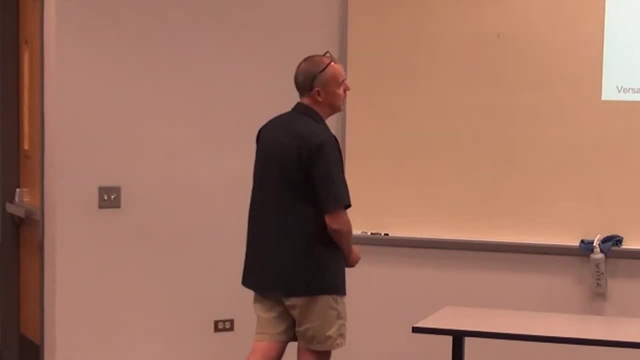 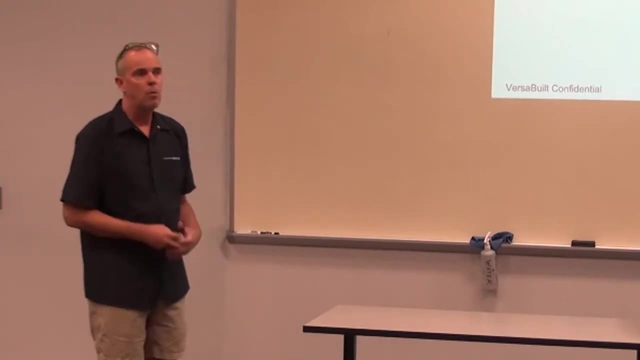 on the use of robots in the industry, And China is by far the largest consumer of robots in the world, And we think of China as being a place where labor is low and that's why all the product manufacturing is going to China, because the labor costs are lower. But 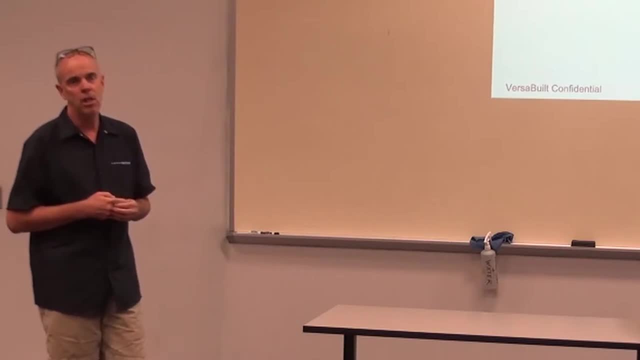 China really is the fastest adopter of robots in the entire world. In fact, we have a lot of companies in the United States that have already been in the market, And so we're seeing a technology in the world. South Korea also very, very big. Most of Europe, really, really. 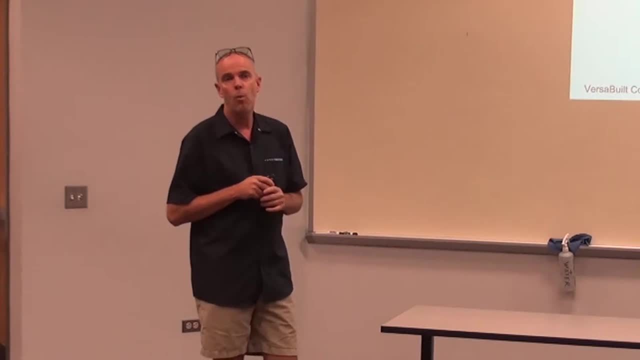 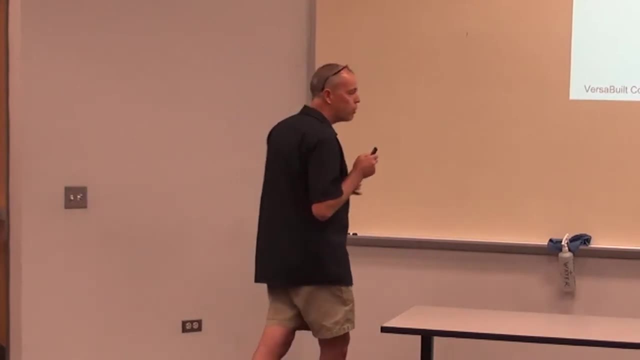 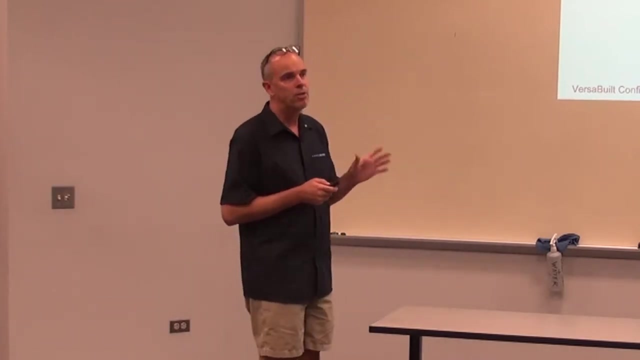 big. The United States is way, way behind the rest of the world, the rest of the industrialized world, In terms of robots per 10,000 workers. I don't have the data for that, but it's kind of interesting to look that data up. but we are way behind, especially if you look outside. 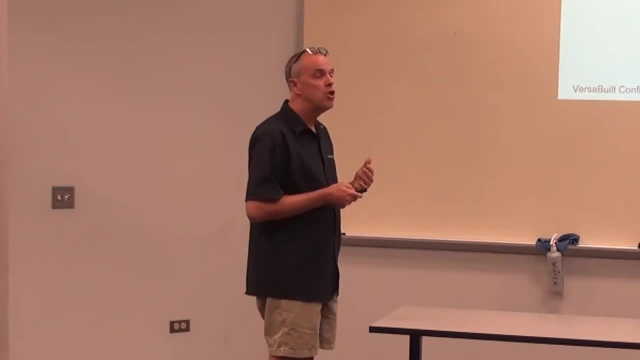 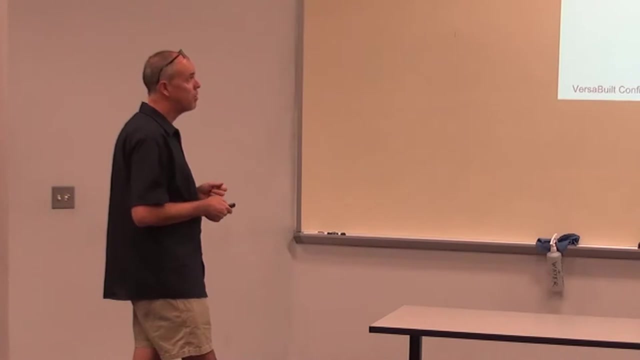 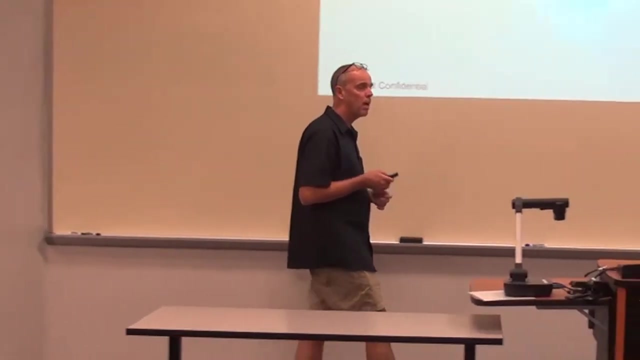 the automotive market. It's just really within the last two or three years that robots are gaining significant traction in the United States outside the automotive market. I think another really important thing to note here is that most robots are still deployed in what I would call high-volume, low-pitched manufacturing. If we're making an iPhone, 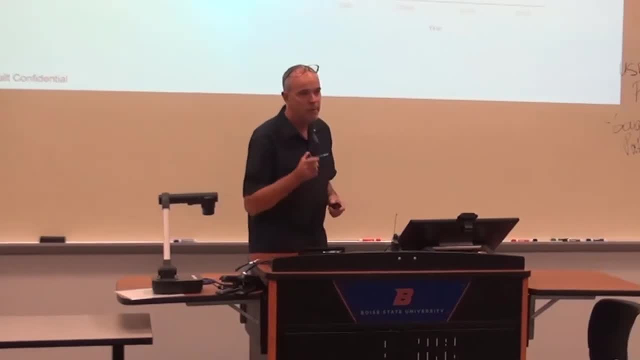 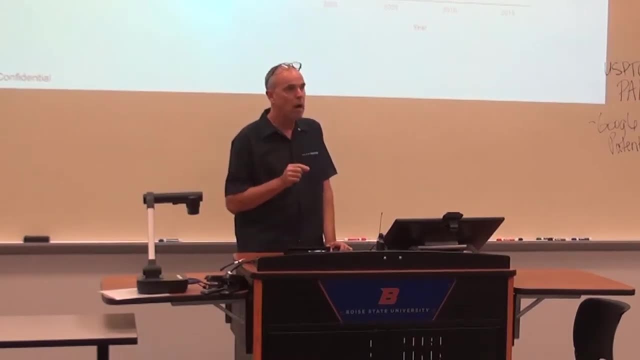 for example- and I'm going to just make the iPhone- If we're making an iPhone X, then there's probably several thousand robots that are out there in the world someplace that are dedicated just to the assembly of the iPhone X: High volume, doing the same thing over and over again and really no mix. They're 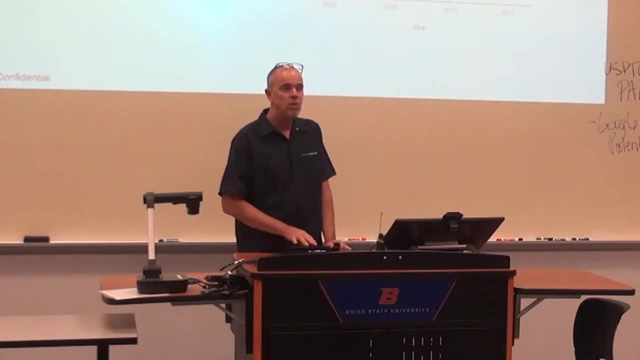 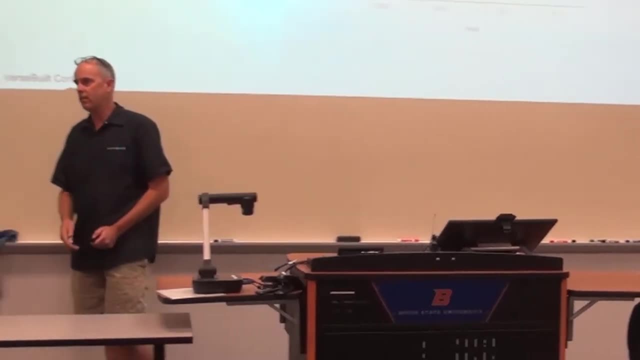 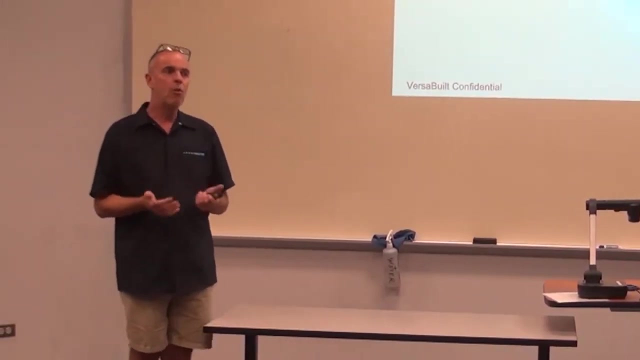 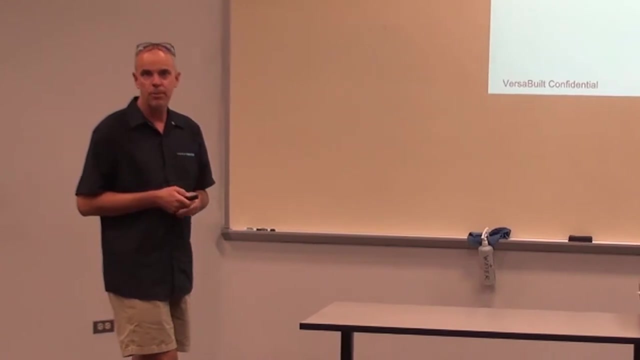 only doing the iPhone X. That's what you see still for most robotic applications. As consumers, we like different things, We like unique things, We like things that change frequently. So the general manufacturing market is moving towards lower volume, higher mix applications because we have more parts that we're building. 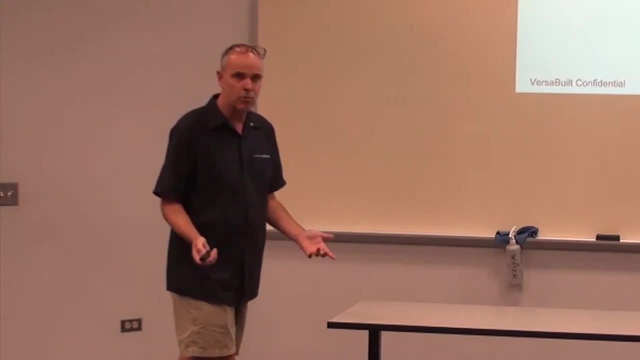 in smaller quantities. Also, you've heard of lean manufacturing principles. I'm sure you guys have been introduced to that somewhere in your school studies. Lean is about building to consumer demand. not trying to build mass production, but building to consumer demand. 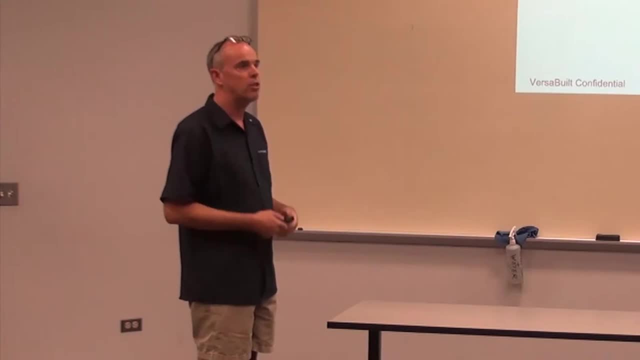 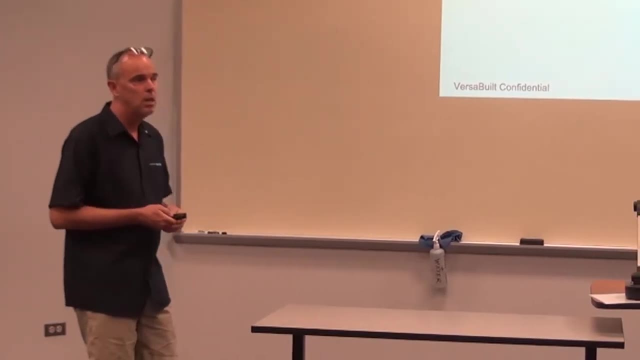 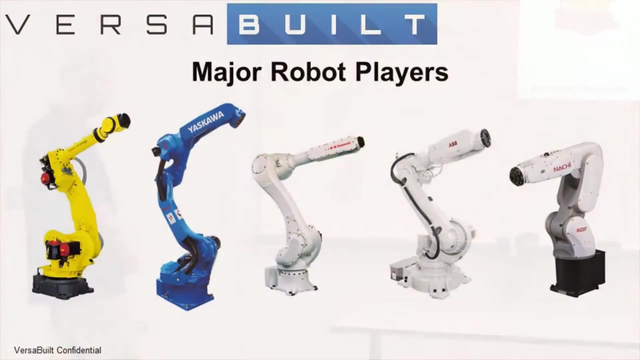 That's a number. I'll mention massive quantities, instead trying to build manufacturing systems that can operate efficient more efficiently with lower volumes and higher apartments. so some of the major robot players in the world- Bannock is number one. they're privately held Japanese company. about fifty. 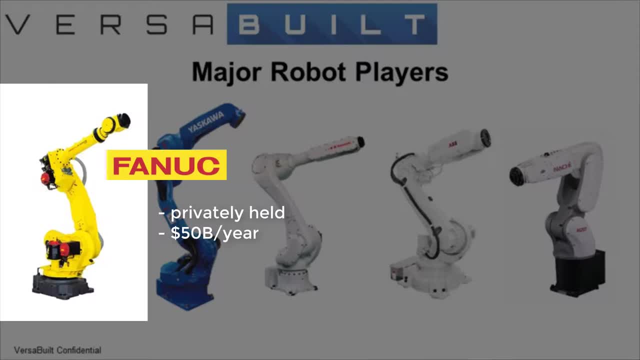 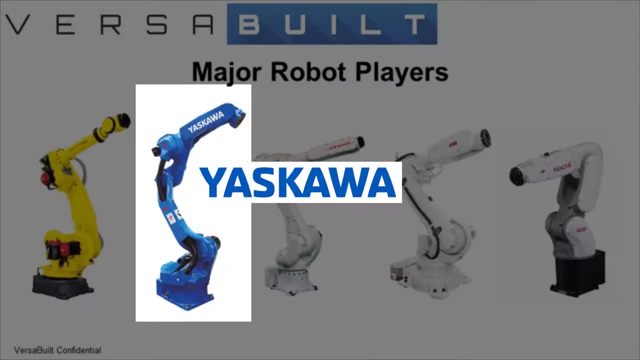 billion dollars a year. they're the also the largest maker in the world of servo motors- the motors that that drive robots, that drive CNC machines, that drive any kind of a motion activity where precision and high torque are required. Yaskawa is another Japanese company. it's very big in Asia. Kawasaki has been a 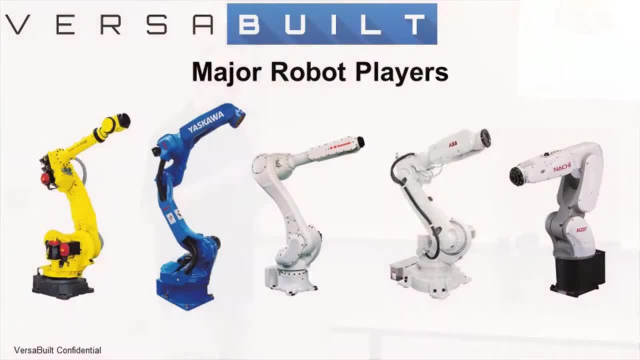 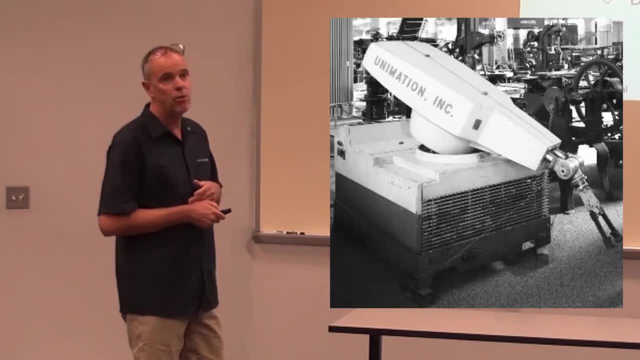 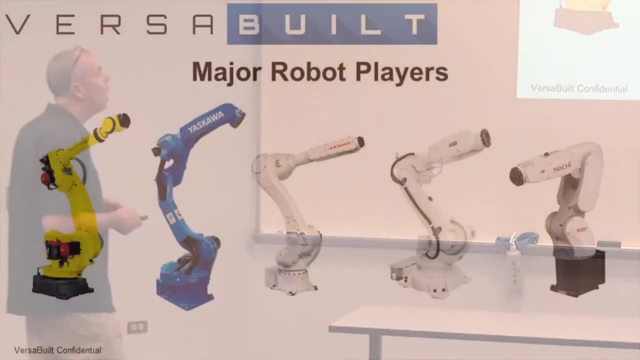 company that's been in the robotics industry longer than anybody else. you saw that picture back here: the unimation robot. well, unimation didn't last too long. Kawasaki licensed that technology and started going to make the building the Kawasaki unimation robot. they're still big, but they're not considered a terribly innovative company anymore. 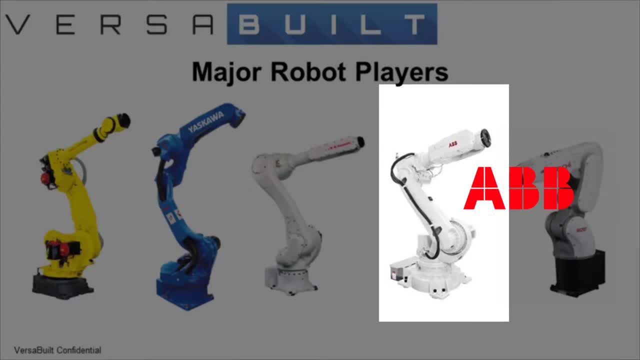 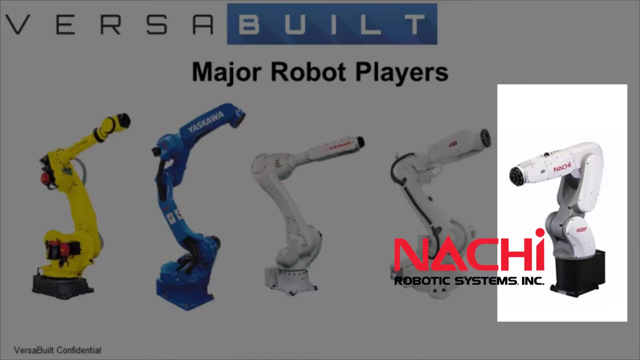 ABB is a robot that we use quite a bit in our business. they're a company that's based out of Switzerland. they're also very big in power distribution systems, windows, things like that, and then Nachi, another Japanese company. so development of industrial robot applications. so how do robots get? 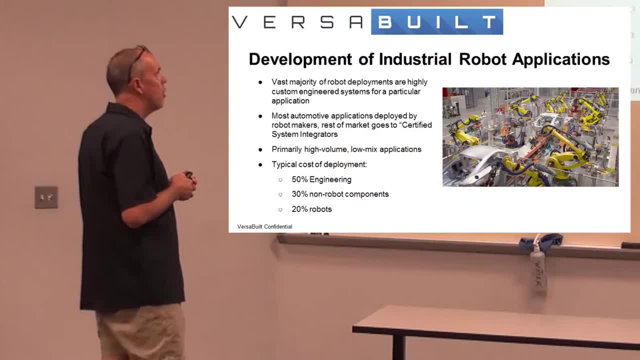 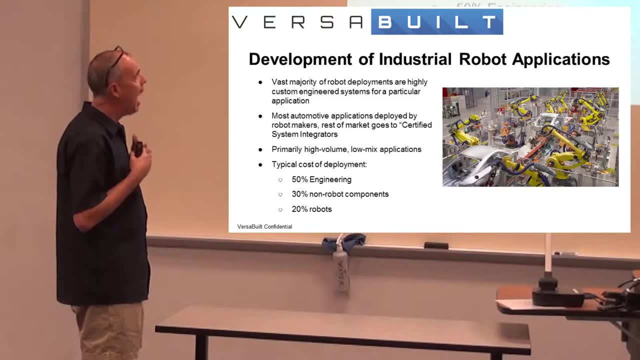 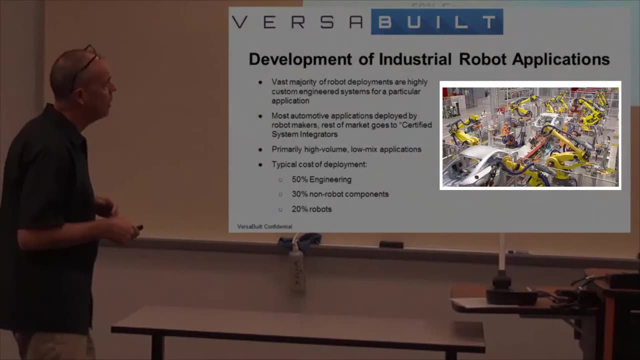 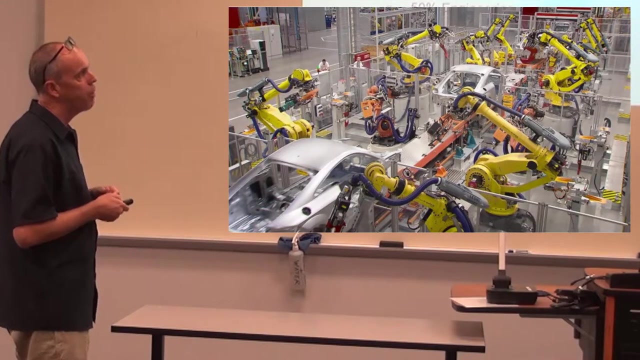 deployed today. so the vast majority of robots that are deployed in the world are deployed in these highly custom engineered systems for a very, very particular purpose. this line here, you see, that's an out ETT. this line was probably built. it will probably last somewhere between three and six years. 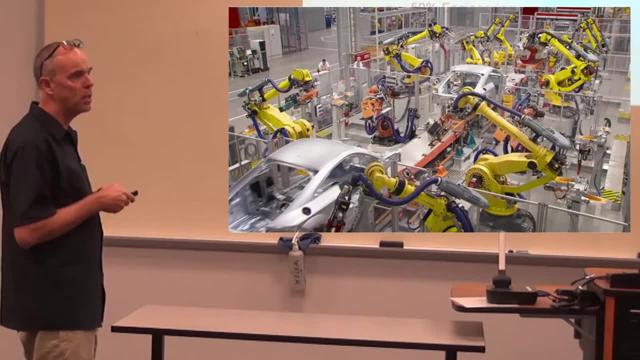 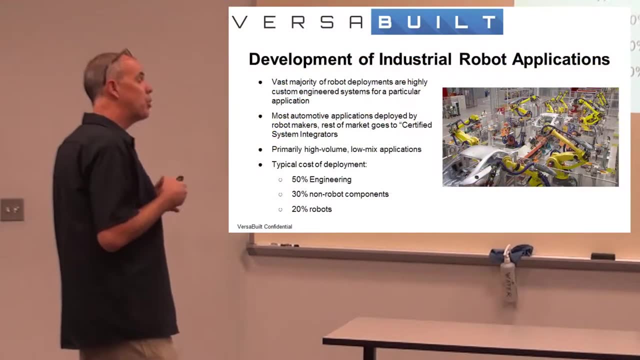 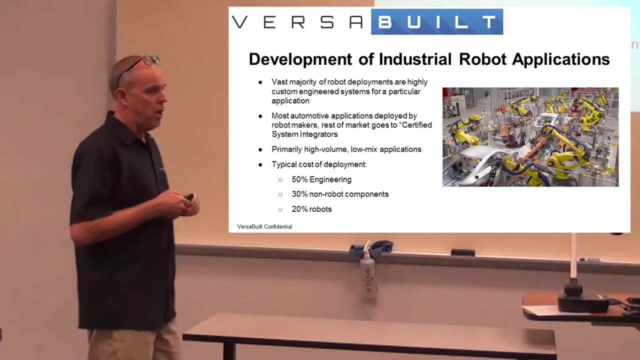 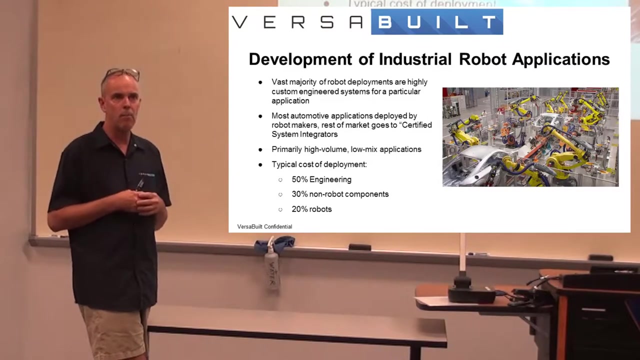 seven years and it will only do these cars. so these robots are doing the same things over and over and over again. if you look at the total robotic market. the other thing I found really interesting is when you go to work with a robot company and you want to buy robots and develop. 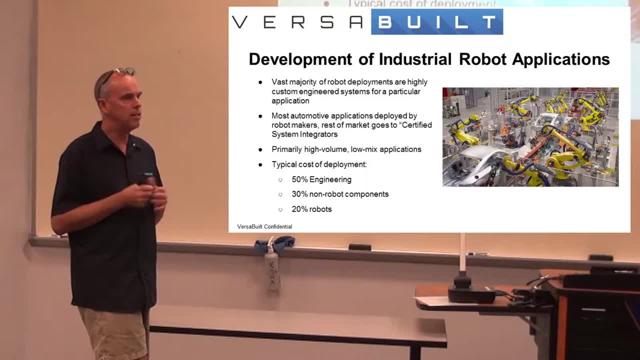 applications for them. then you become what's called like a certified system integrator, but they give you something like this and then you get to work with a robot that's based out of Switzerland training and you agree to do certain things and work with them, and then they give you the ability. 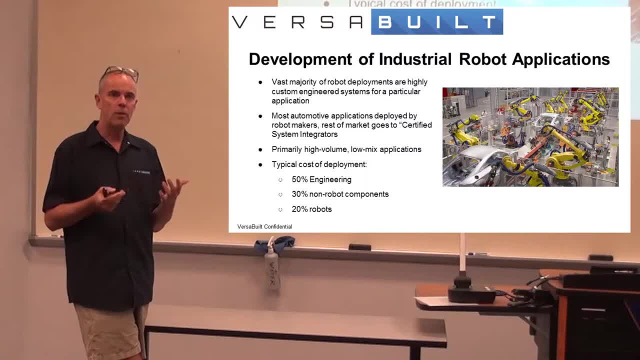 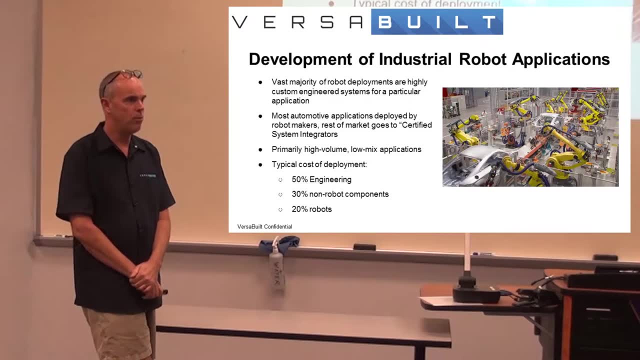 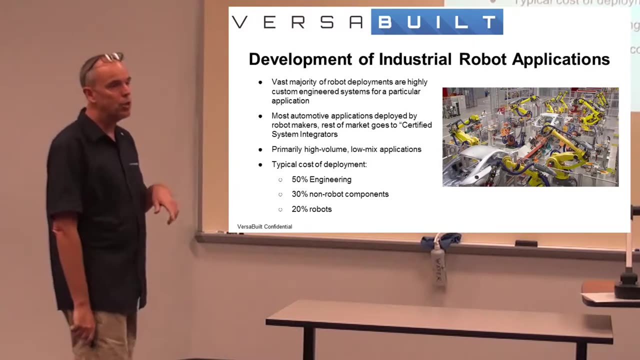 to purchase those robots and resell them, and what they will tell you is: hey, you can do anything in any market you want except automotive. we own automotive. so all these robots that you see in automotive are either those applications are either being developed internally by the automaker. 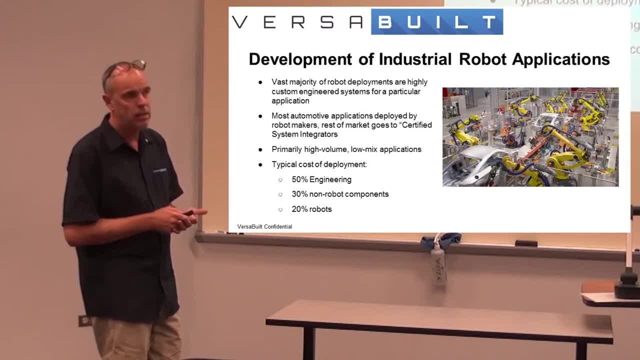 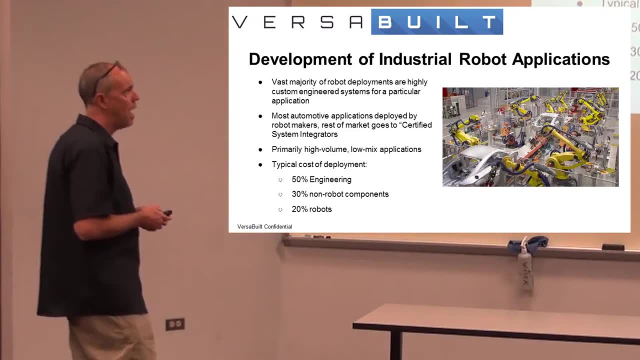 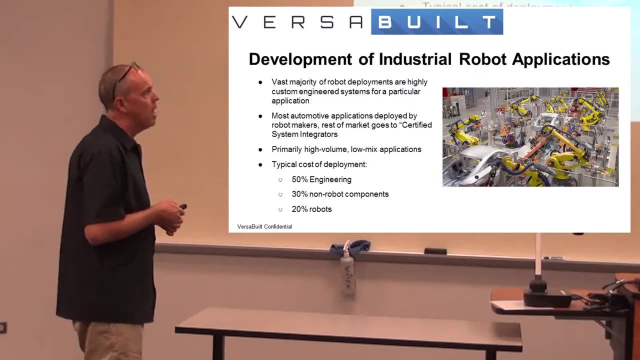 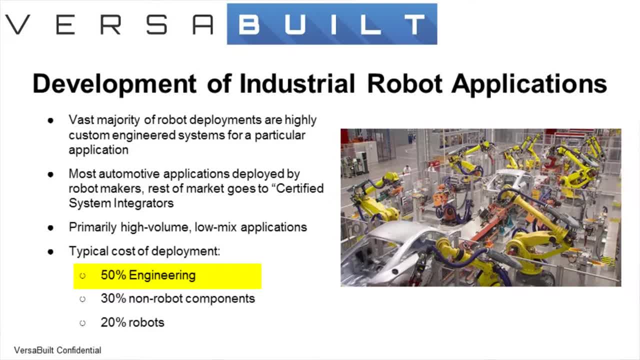 thing work, design it, build it, test it, deploy it. 30 are non-robot components. fencing robots need to have some sort of a safety system around them. robots are extremely fast, they're extremely powerful and they can and do kill people you do not want to get in the way of. 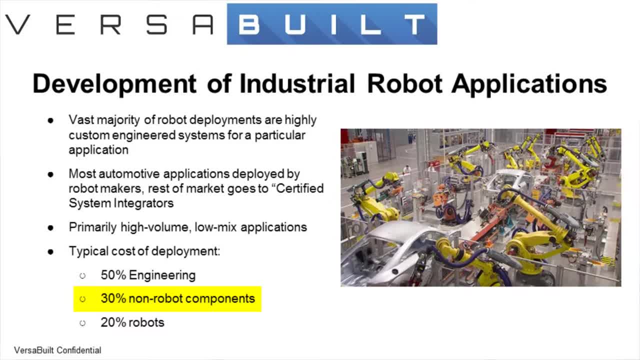 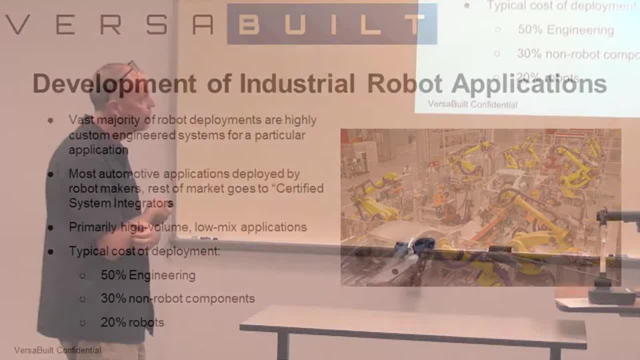 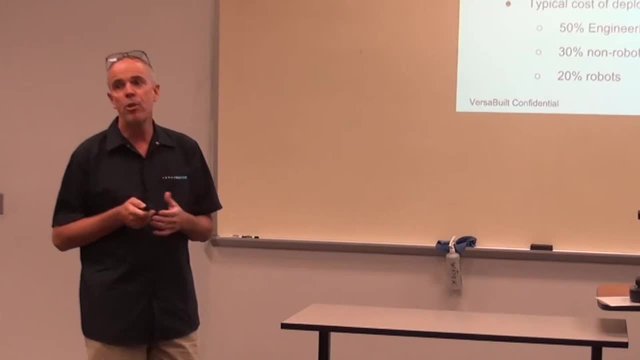 the robot, the end of arm tooling, all the infeed and outfeed- all those things add up to more than the robot itself and that that has played some kind of interesting dynamics and how this overall market has developed and what some of the opportunities are for disruption in this market. 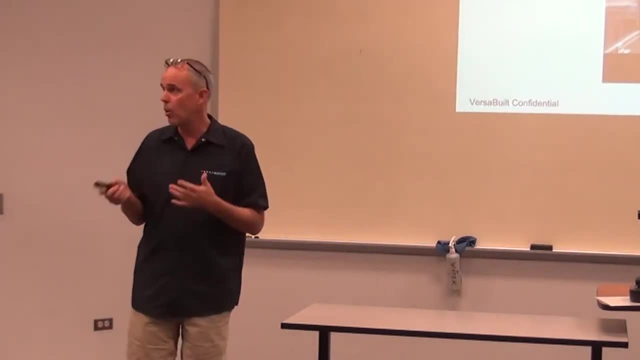 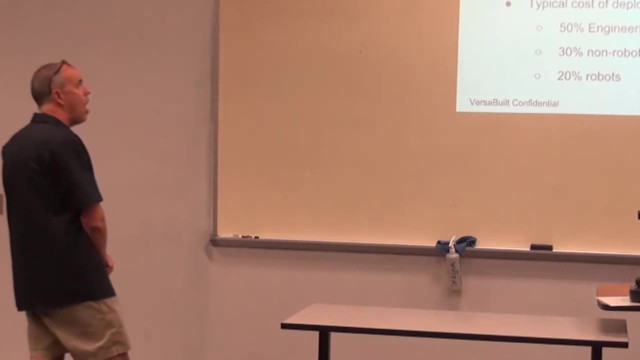 and guys, if you have any questions at all, as i'm going through this, please stop and ask your questions. go ahead. uh, where are the germans? where those dead robots? uh, so the germans play some really important roles. there was a german company making robots called. 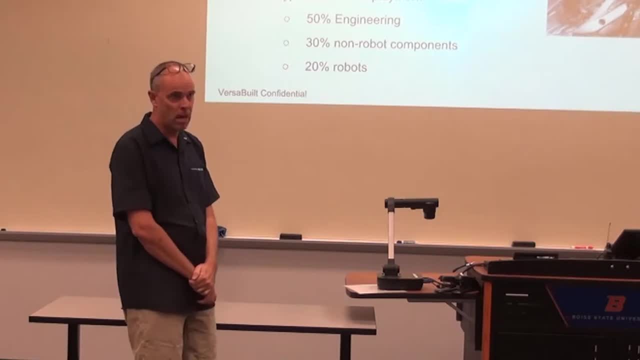 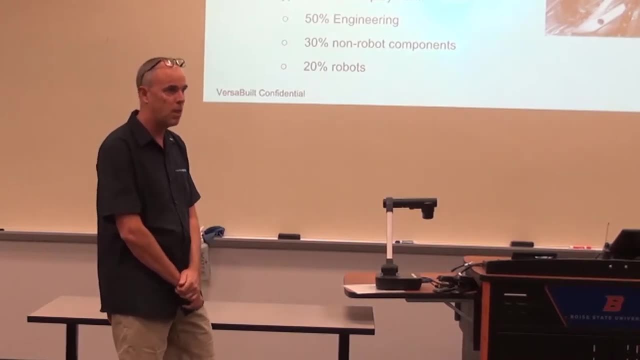 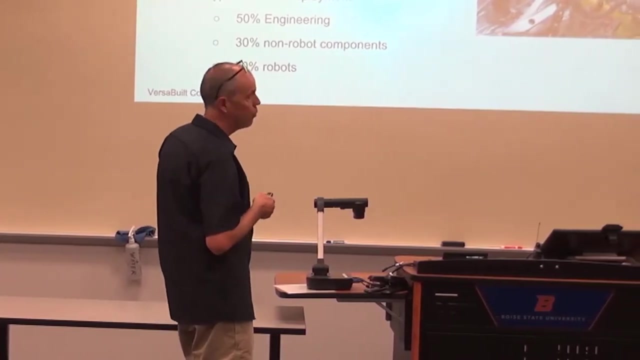 cooka and they were just recently sold to a chinese company, so they're no longer joining uh. the largest maker of the end of arm tooling, uh the grippers and things like that, is a company funny called shunk. they're a german based company, about five billion dollar a year company. 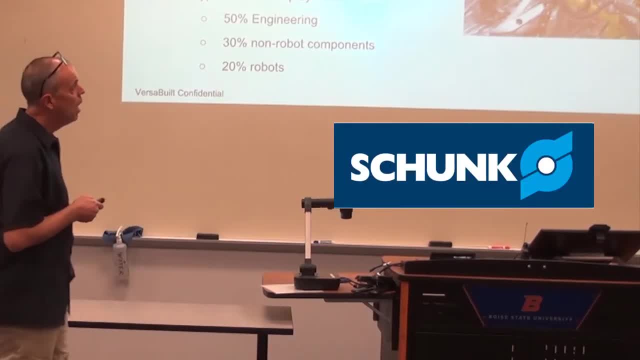 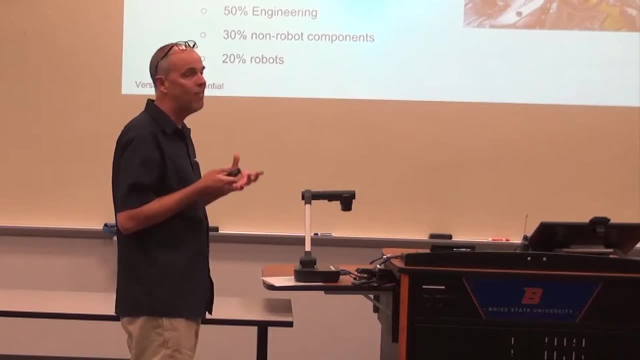 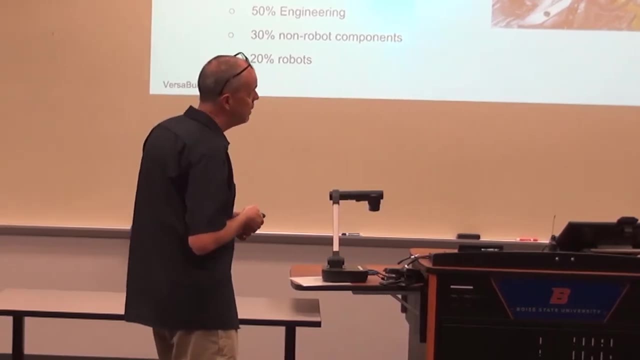 uh, that was a company that had super smart plants, so one of the big ones was radio忽. They make the tooling here and then they also make vices and chucks and things like that. so for machine tools. so they're going to hold parts firmly for processing to be done. 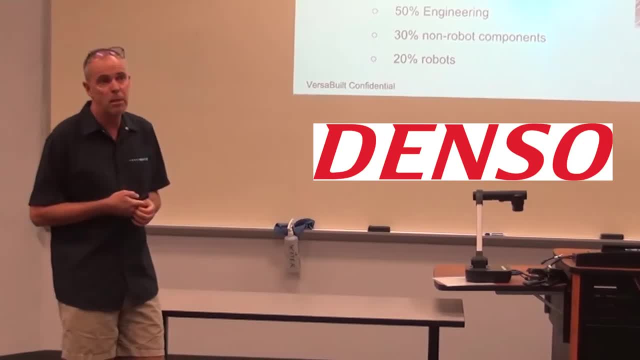 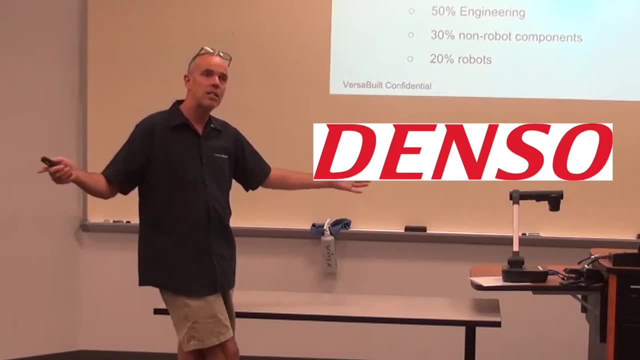 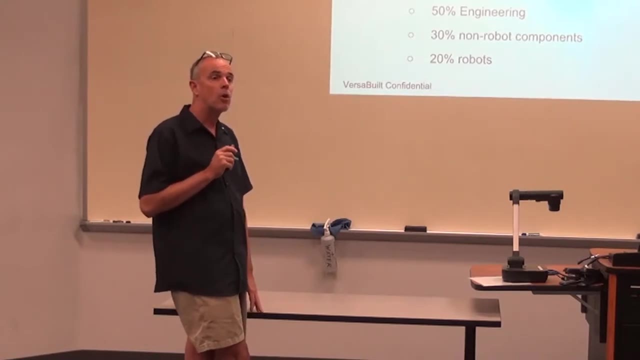 Another company, Festo, is also very big. They're a German-based company, about a $2 billion a year company. They make linear rails, linear actuators, so instead of six axes one axi. They also make rotary axes and things like that. and then they're also very big in what are called programmable logic controllers, PLCs and pneumatic control. 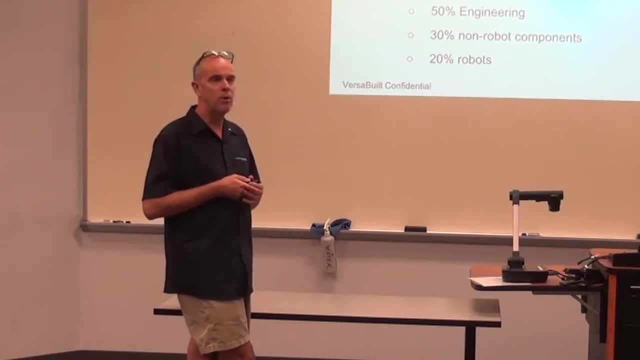 So typically most robots, if they have a gripper or an actuator or something like that, they're typically pneumatically actuated and Festo is very big in that value and the control of the value. Siemens doesn't have a robot. 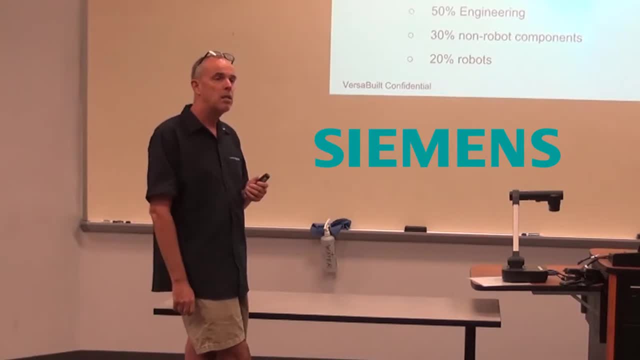 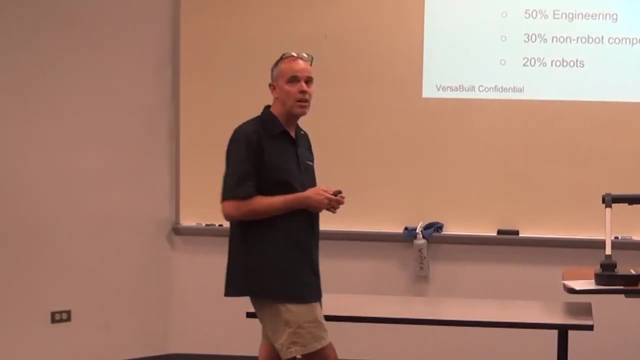 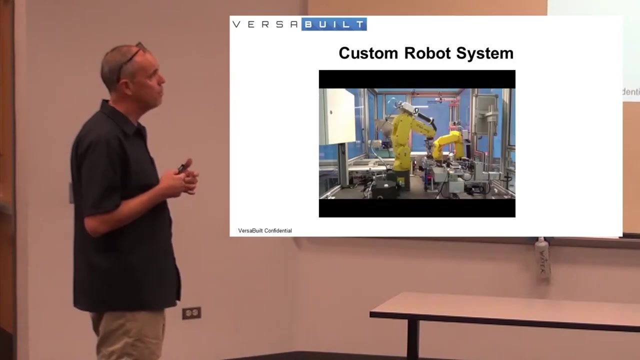 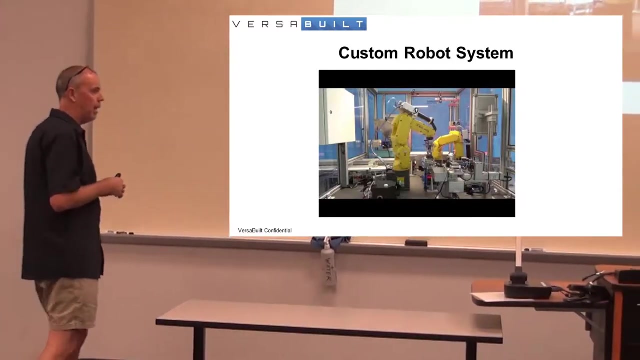 Siemens does not have a robot. but Siemens does make controls, Primarily for CNCs, not so much six-axis robots, Siemens also makes motors, the servo drives. Any other questions? Alright, so this is a short video. This is a really typical type of application that would be developed by a small regional system integration company. 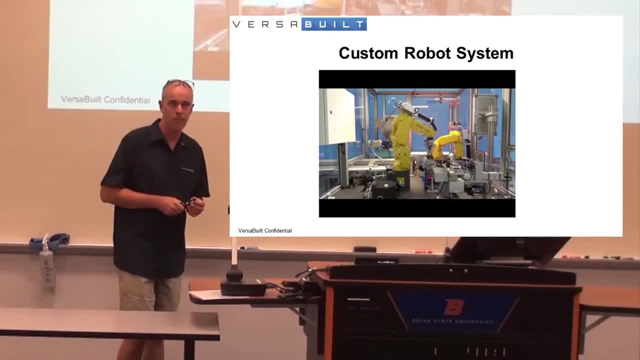 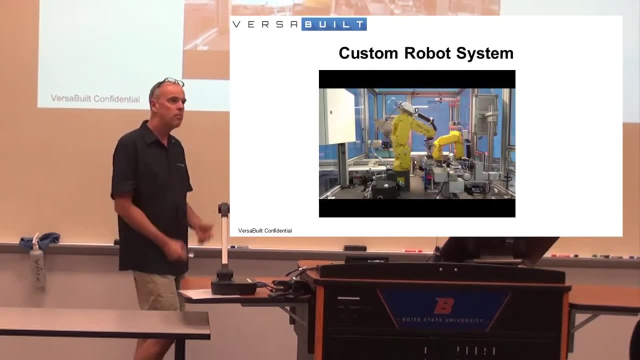 We've edited it. How many of you guys ever heard of a company called House of Design? They're a local ADV system integrator and this is the type of stuff that they do. A customer comes to them and says, hey, I've got to make this thing. 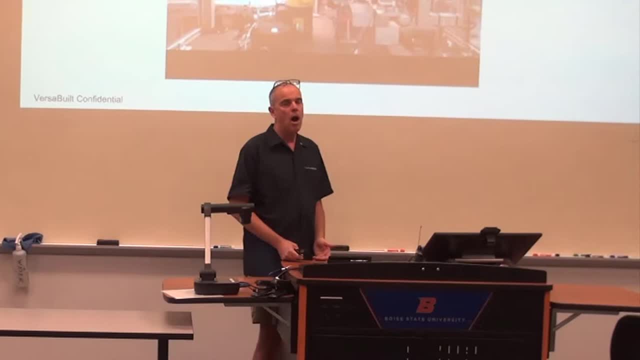 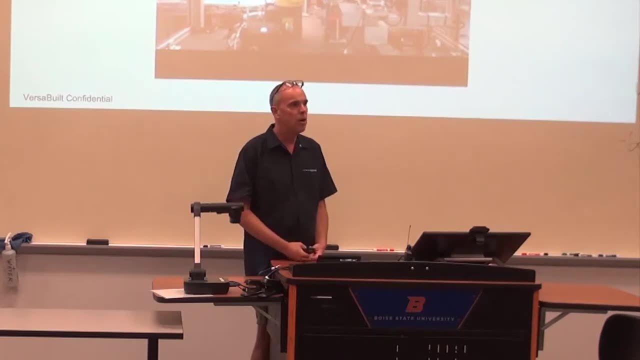 I've got to process this thing this way. And then the system integrator goes in and understands what the customer's problems are, what the needs are, defines the scope of the project and designs a solution and implements it. So this would be pretty typical. 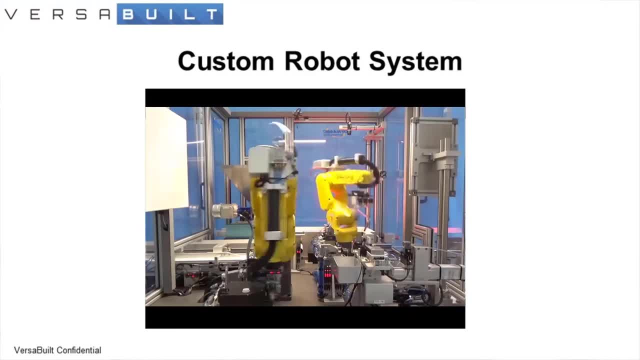 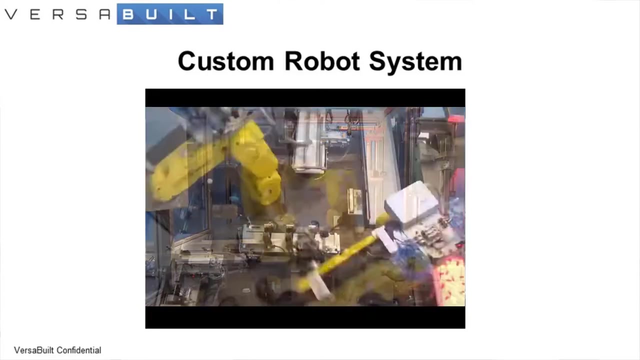 The details of what are happening here aren't that important. What I want to show in this video is how specific this application is. So you're going to see some parts that are being processed here And, as you can see in this video, try to imagine what if you needed to expand this system. so it worked with a part that was twice as big. 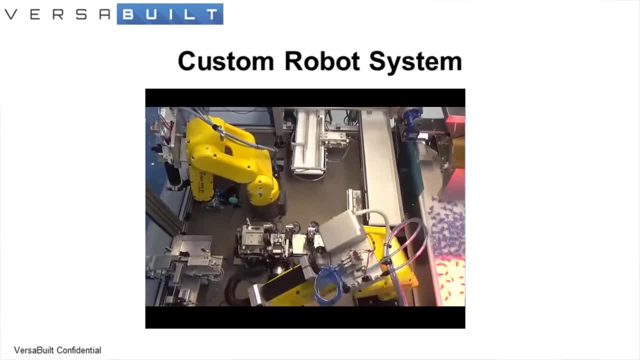 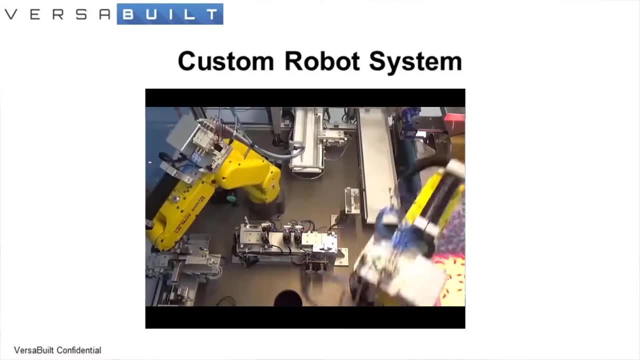 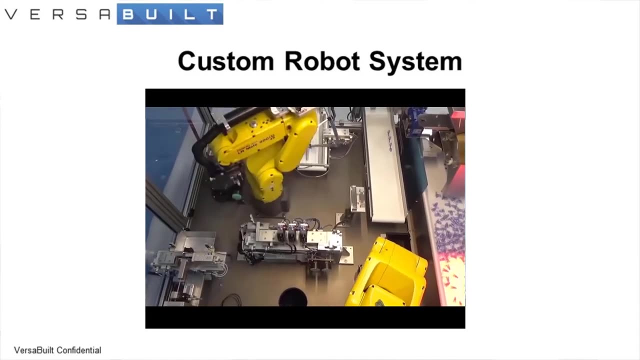 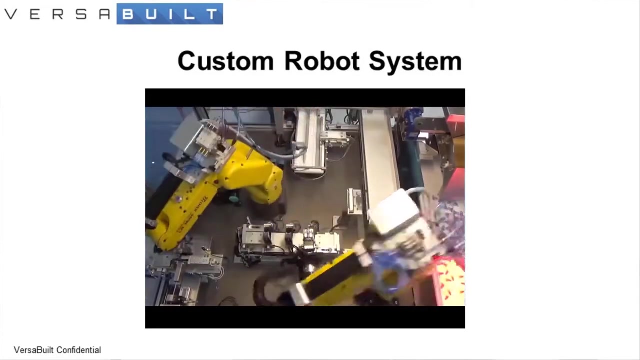 It would be starting almost from scratch. So pretty typical kind of a cell. We have these aluminum extruded frames that are custom built. They're- a company called 8020 is most famous for making those- And then these are small, authentic robots. 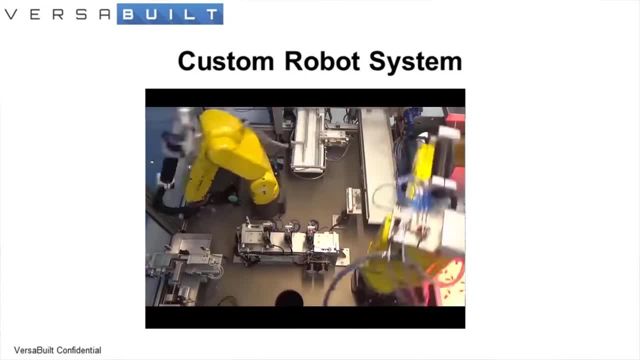 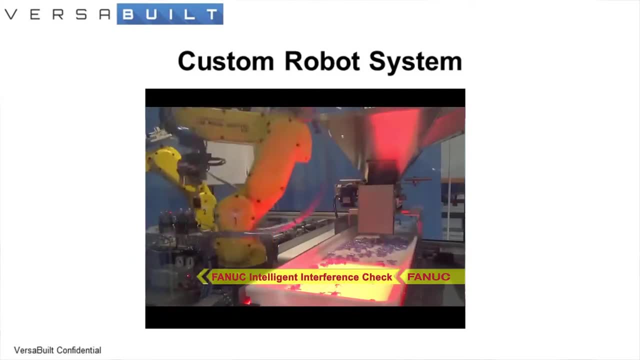 The retail cost of those robots is about $30,000 a piece. As you can see, they move very, very fast. They move very, very quickly. They're very, very fast, very, very accurate. Accuracy is the wrong word. 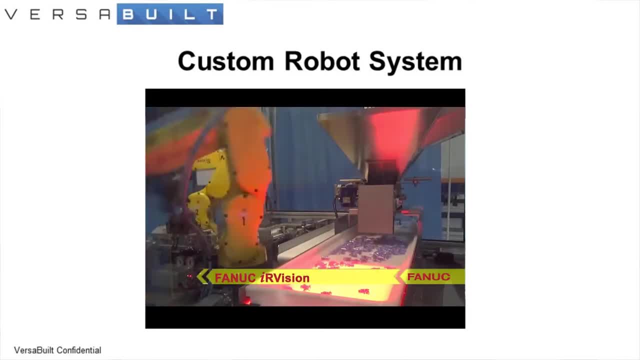 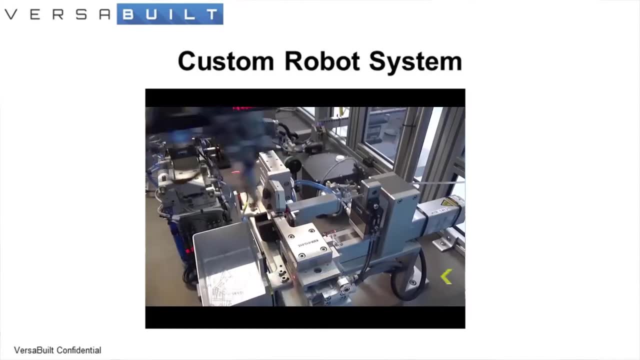 They're very repeatable. Most robots are very good at repeating to the same point that you teach them. They're not as good as hey. I have to top this point. I need to be 12 inches this way and 13 inches that way. 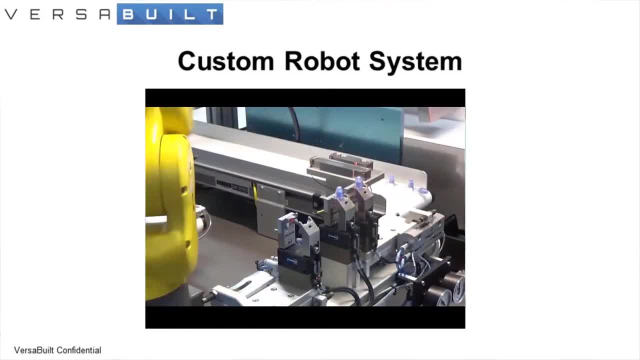 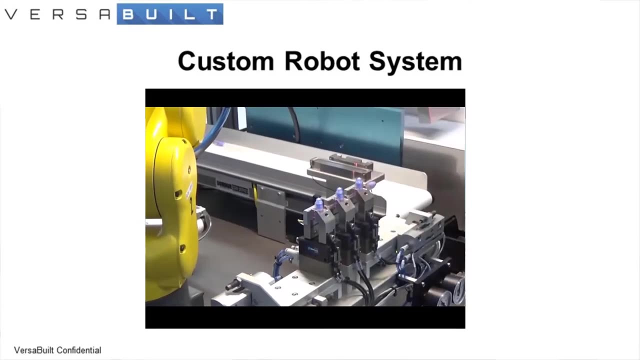 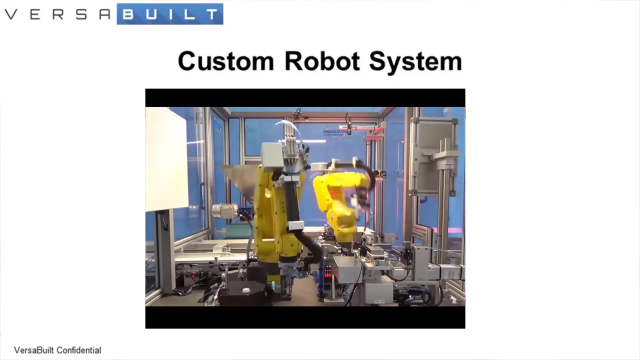 And these robots are picking up from an infeed here little tiny parts and then staging it into little fixtures. here This robot is picking up other parts. The two parts come together And then this is the outfeed here. So infeed, infeed, where the parts get staged to be assembled together, and then outfeed here. 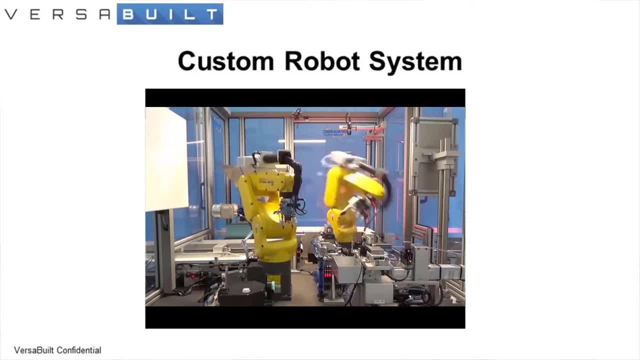 Over here this infeed. you can see the parts are kind of scattered all over the place. Vision is a very important thing in industrial robotics, In industrial robot applications, And the camera will come down and show where the part is to the robot. 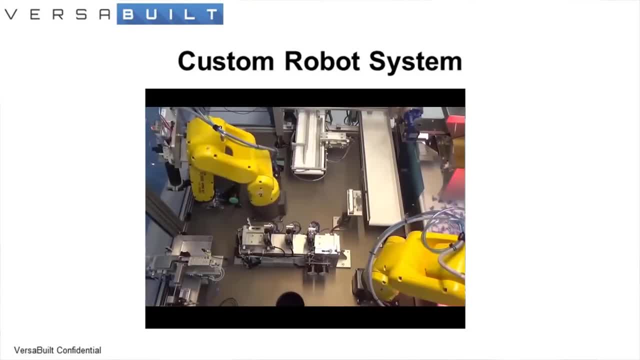 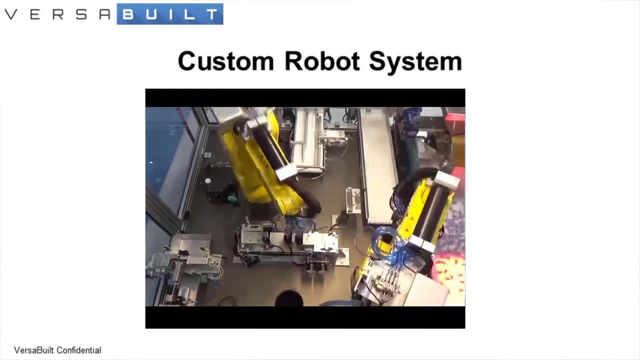 The camera can then understand what the orientation of that part is and give the robot a picture of how it needs to approach that part to pick it up. That right, there is some sort of a quality check where the robot's verifying that it has the part correctly. 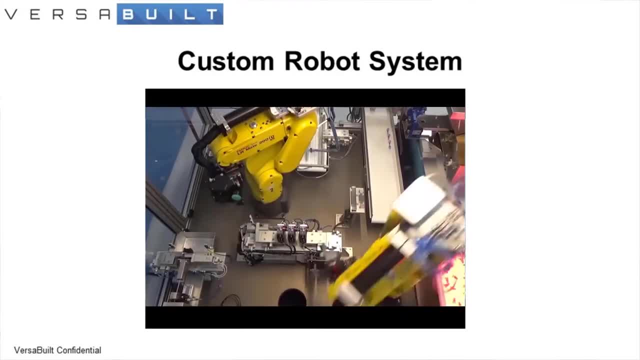 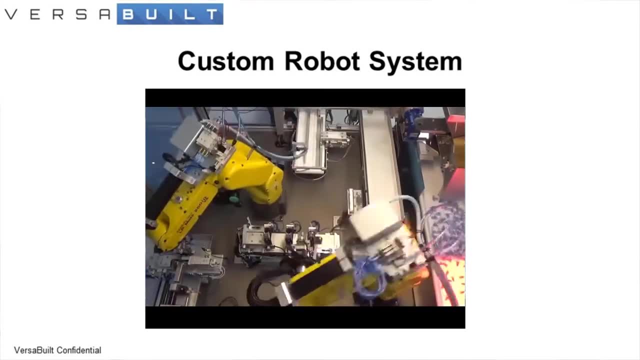 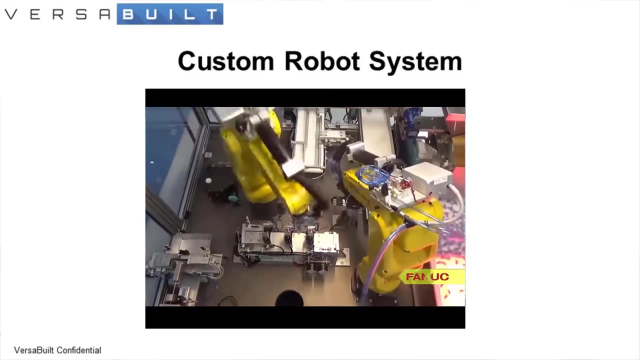 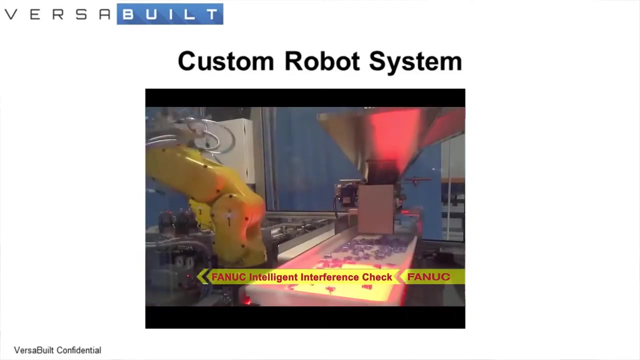 These are the actual parts that are being assembled. That's a shunk gripper right there we talked about. I assume that's real time. This is real time. This is not sped up. A robot. application like this, from start to finish, would typically take between six months and a year to develop. 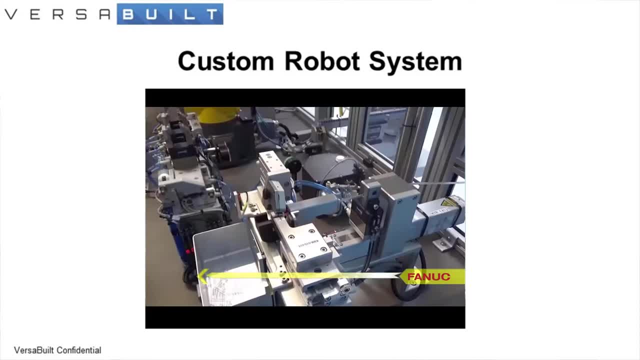 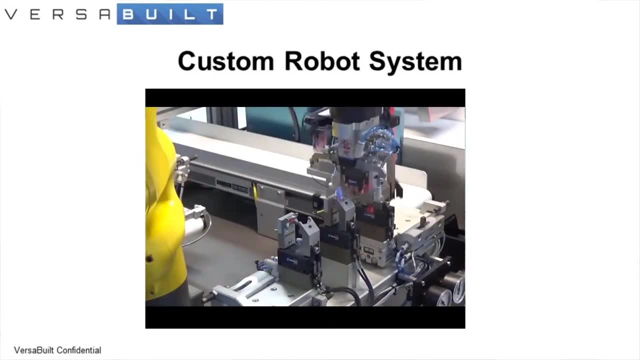 It was probably a team of between Two and five engineers. The hardware cost all the parts and pieces there were probably about $150,000. And then I would estimate the engineering on this to be somewhere between $150,000 to $300,000. 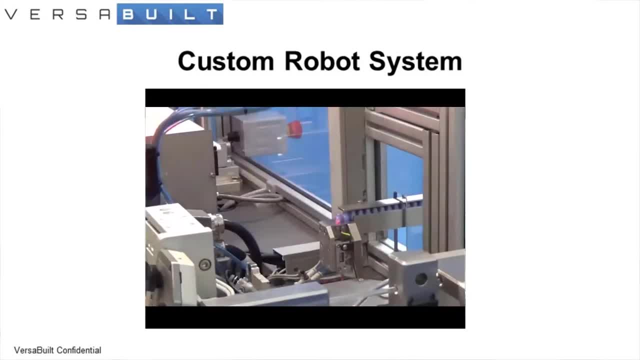 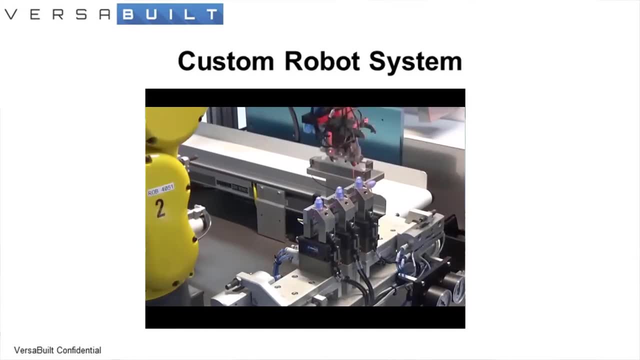 So you're saying that this is not too important, but I am a little curious about the large screen that just turns red. Yeah, Is it like the robot? I mean it's to lift the robots. So you mean that down low? 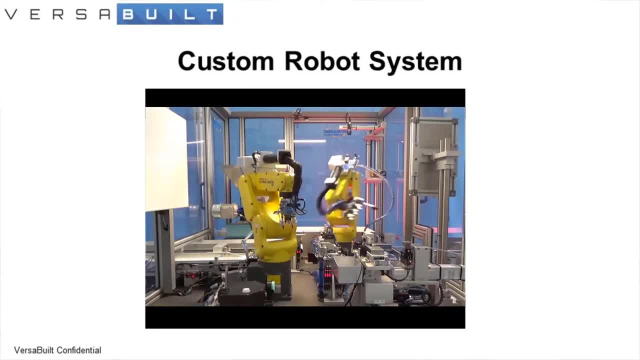 Up there, That thing right there. Yeah, I'm actually not sure what that is, to be honest with you. My guess is it's some sort of a quality, some sort of a vision inspection kind of thing. Anybody have any questions about that? 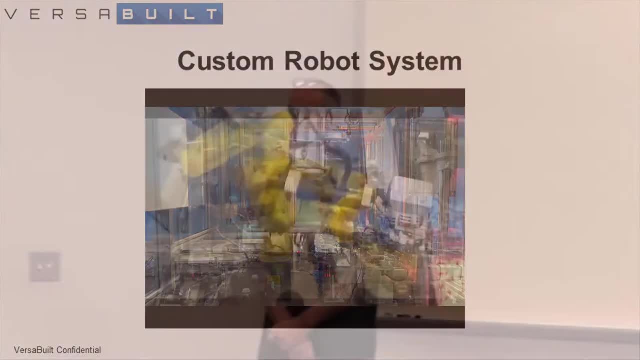 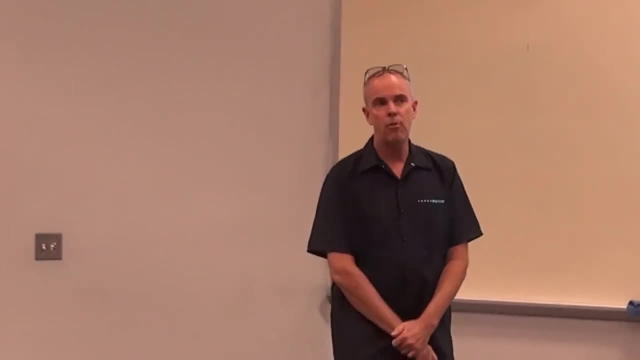 Yes, You said that robots weren't so good about I need to go 12 inches and 3 inches. They're not as good As good, So. So repeatability: state of repeatability. So ABV is a little bit different than most other suppliers. 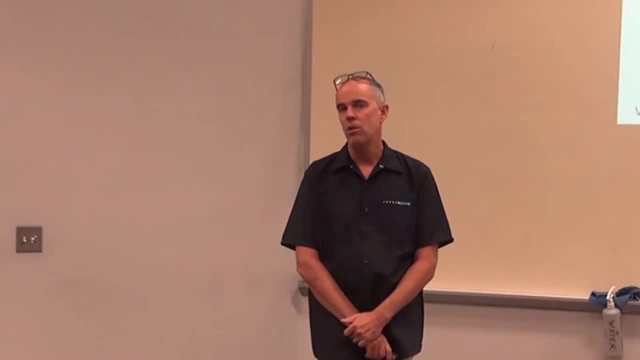 They will state a repeatability and an accuracy. So most robots in that kind of category typically have a repeatability of .1 microns. I believe .007 inch. Most vendors will not give you a stated accuracy, So let's think about this problem for a second. if I could, 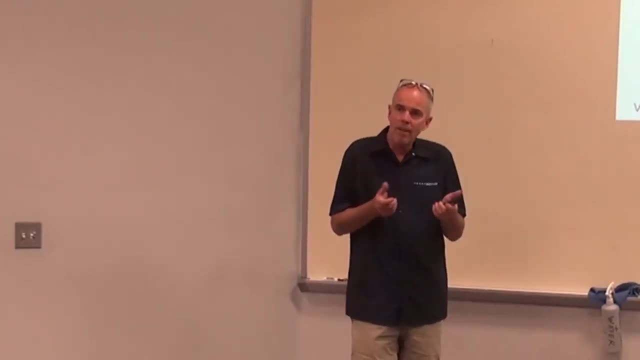 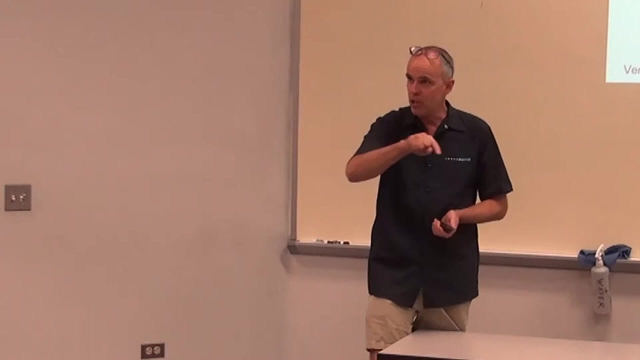 So repeatability. you have a robot and you have a thing called a teach pen and that allows you to jog it around. And you come over and let's say, we want to pick up right from this corner. So you teach it down, down, down and you say, okay, right here. 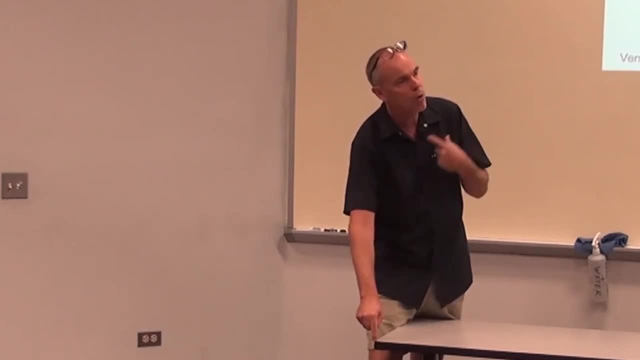 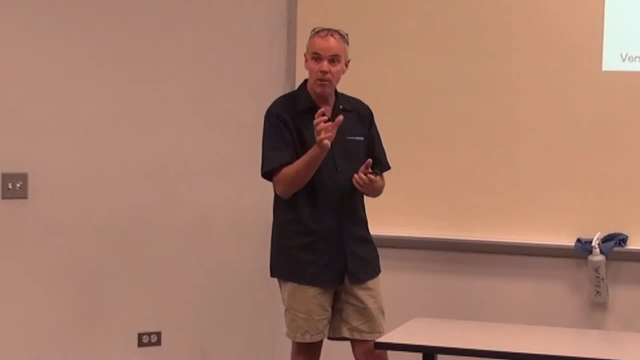 Think about the problem So that the robot can read what all the joint values are. It has encoders or resolvers that count the number of revolutions or micro-revolutions to get to that point, And it knows what all the counts of all those are. 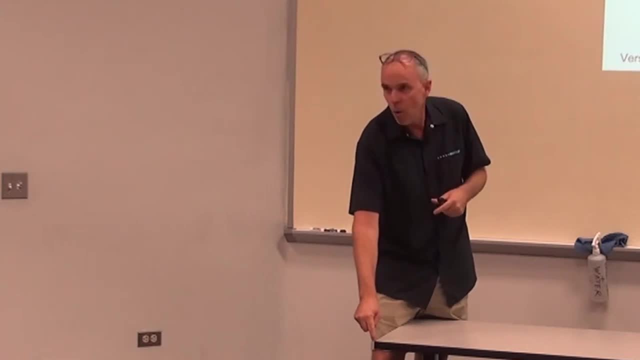 Okay, So that it can go. oh, to get back to that same point, I just have to get all those encoders to those exact same values. But now, if I want to go out here, things get more difficult because I need to know. 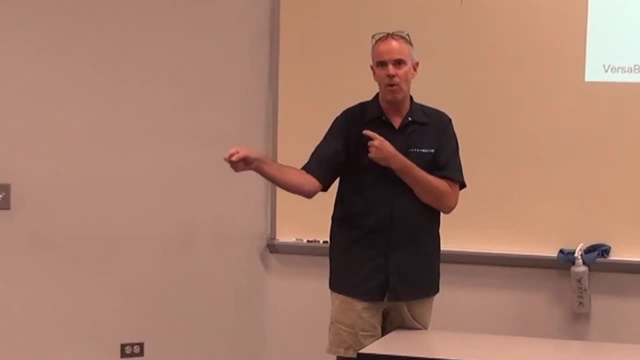 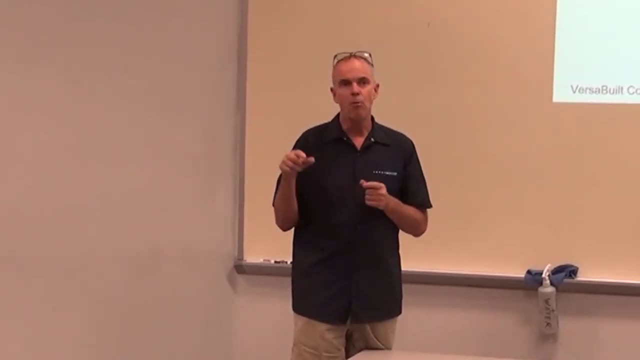 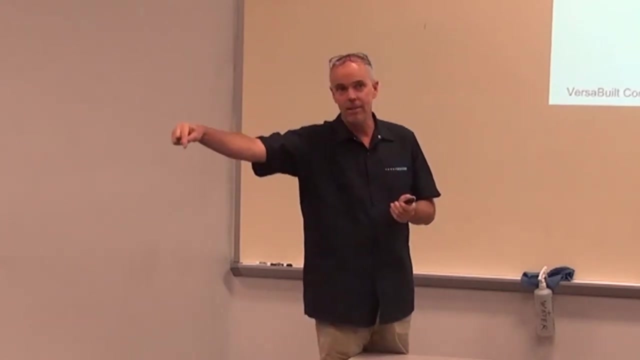 the exact length of each joint. to get that right, I also need to know about gravity and payload. Robots are not infinitely rigid And you'd be amazed. you know, when a robot hangs out like this, a robot like that is probably sagging on its own weight. under its own weight maybe as much as a quarter. 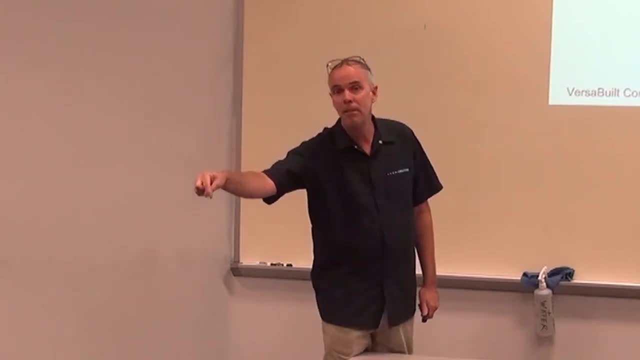 of an inch. If it's carrying five pounds, it might be sagging a half inch, So it's got to compensate for that. So there's a lot of data and it's kinematics to understand. you know how gravity affects. 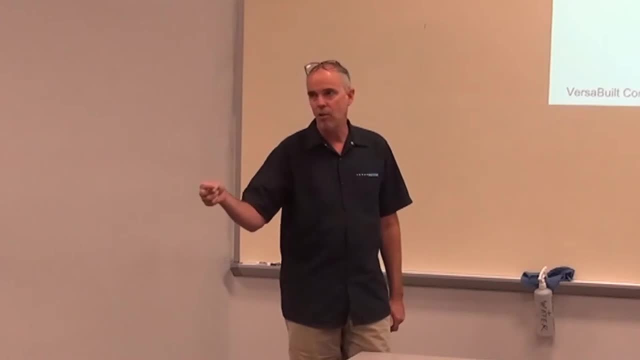 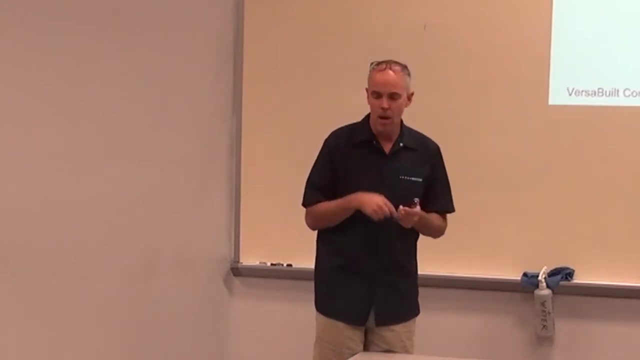 that. But to really get this really high accuracy, what the robot really needs to know is its exact length of all its joints, And the way robot vendors do that is they actually measure the robots. They typically use vision or some other way to say: okay, I think I'm here, but where? 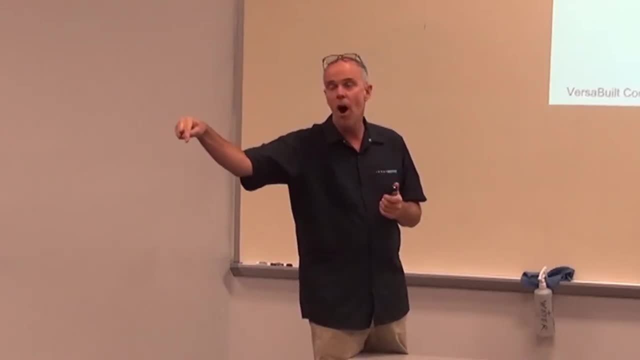 am I actually? Oh, since I'm actually a little bit off and I do that here, then comparing between those two guys, I can maybe assume: oh, I've got this joint. I assumed it was this long. It's probably actually this long. 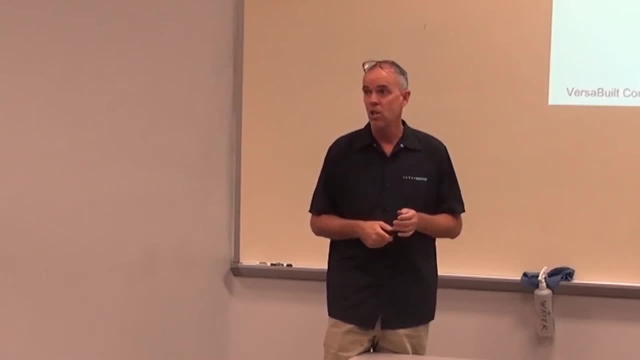 And that's how it gets to it. Does that kind of answer your question? Actually, I was about to take it on a different track. Sure, Because I'm basically wondering if they have some sort of like the adult dead reckoning systems or something. 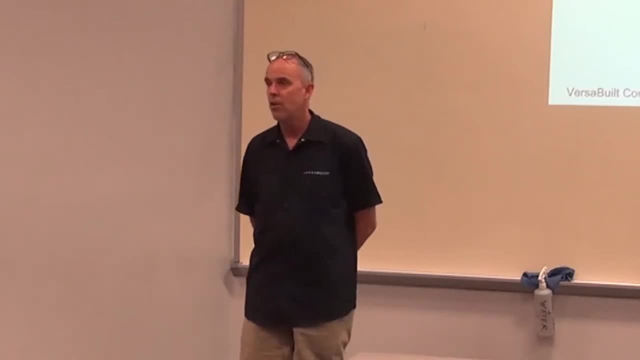 They can with vision, So robots can do a lot with vision. Vision systems have really come a long ways, In fact. FANUC robots: if you have a robot that can do a lot with vision, it can do a lot with vision. 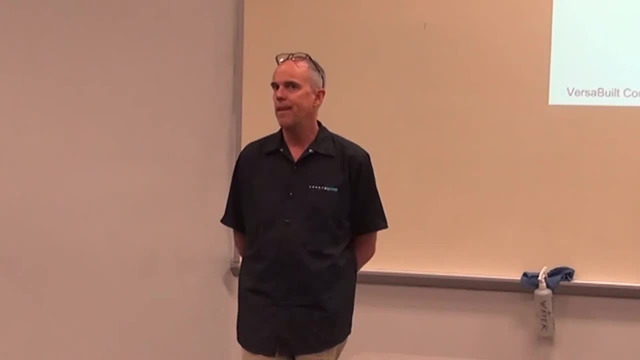 So if you have a robot that can do a lot with vision, it can do a lot with vision. So when you order a FANUC robot, there's no stated accuracy. but you can buy an option or have the factory do an option where they mount a camera on the robot and they actually 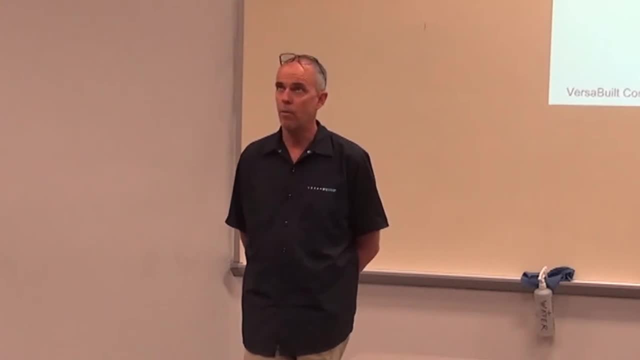 do their calibration for accuracy with vision. They mount something on the end of the robot arm to do that, whereas ABB- the last time I visited their factory, they had physical things. They had physical things that the robot touched to determine and adjust for accuracy. 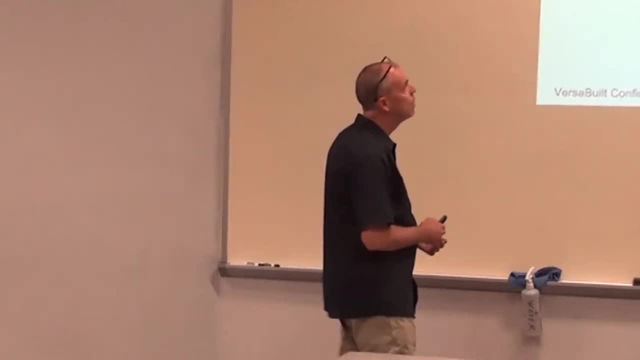 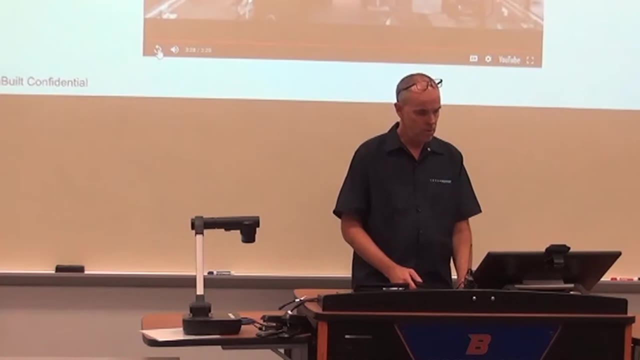 Okay, any other questions? Actually, I got You asked us to kind of think what it costs or what the scale would be If we were to just go excuse me two fold on the size, or? Yeah, that's right. 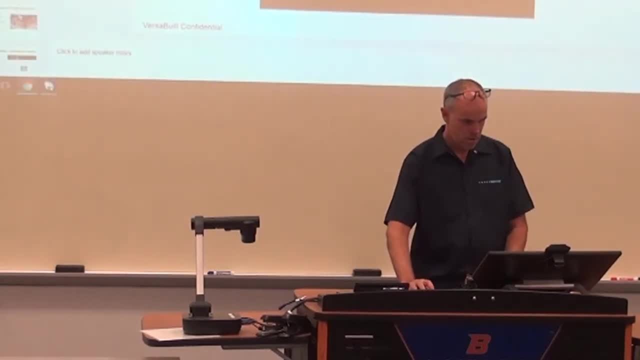 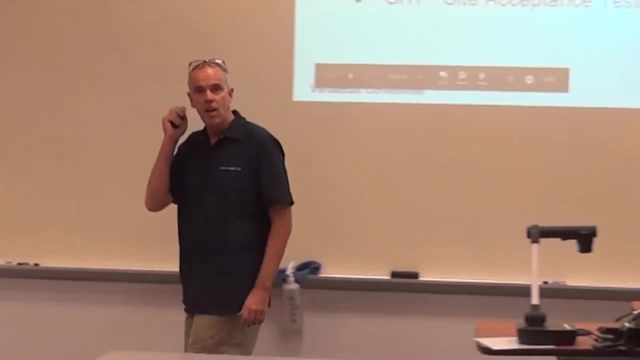 Yeah, of the product and everything else like that. Hold on just a second. I'm trying to get this going again. Start your question over again. Yes, you asked us to kind of think about what it would take to scale that project up Now, if you were looking at one on one. 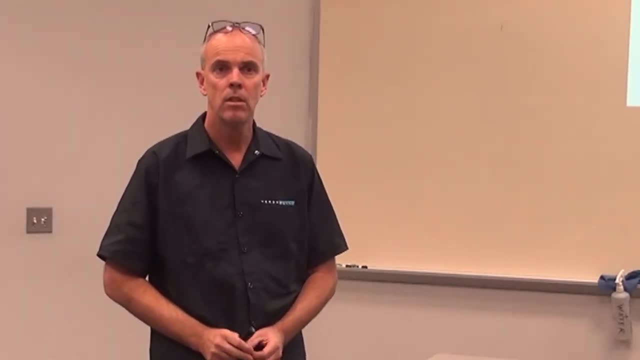 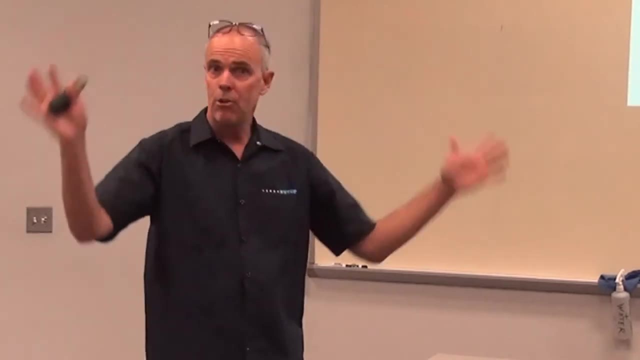 you said the cost of that robot alone was $150,000 plus another. The two robots are $30,000 each, so there's probably about $60,000 there and then $90,000 for all the stuff around there. That's just one setup. That's one setup and you can see that. those little designs for that particular shape part. everything around it was designed for the shape of that particular part. So now if we want to scale up, that's just compounded on itself. but now if we want to change that actual part, like change the way it's going to be assembled- 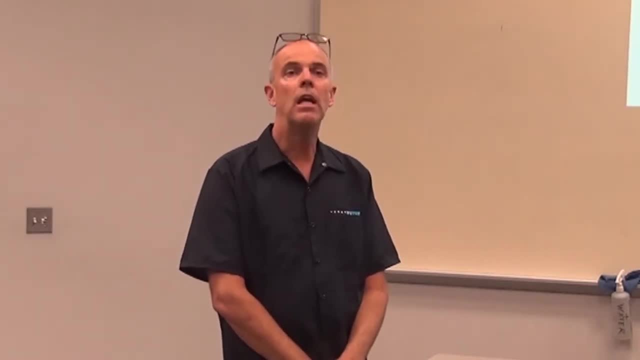 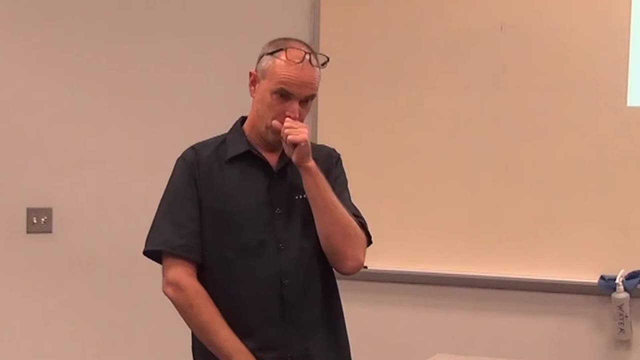 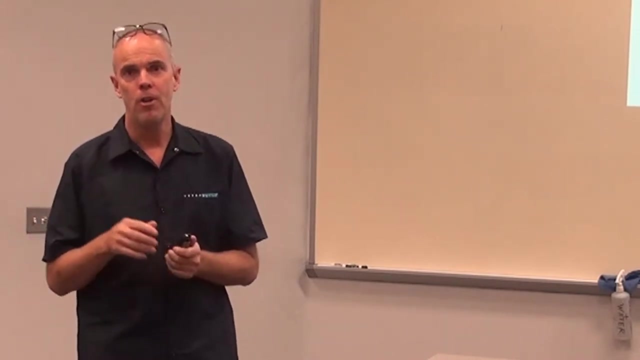 then the engineers have to go back and reassess everything. Yeah, so scaling in terms of volume: add another one, add another one, add another one. Scaling in terms of making one that's instead of a quarter inch diameter by three quarters inch tall to one inch diameter. 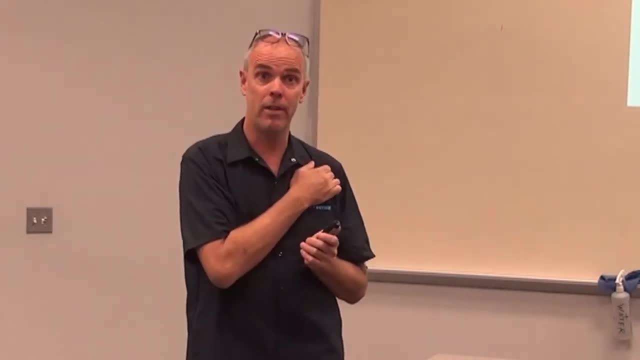 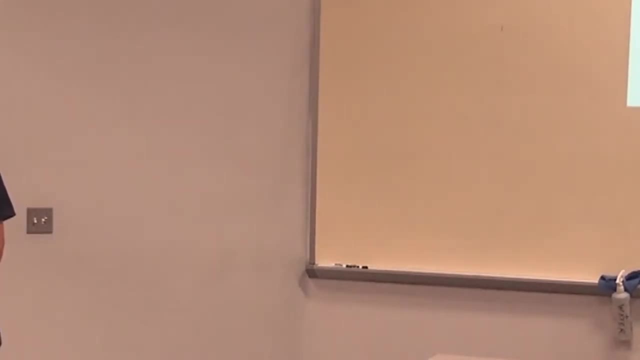 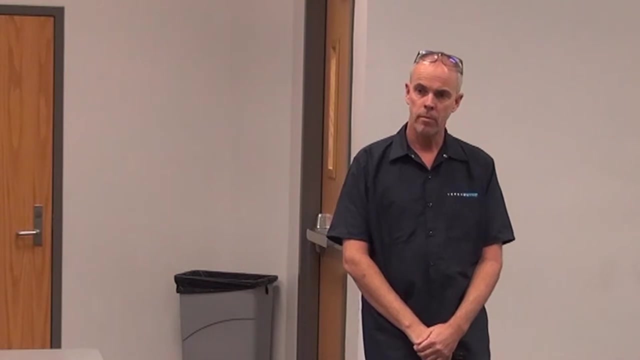 two inches tall. that would be a pretty significant redesign in that type of thing. So that's high volume, no bass. So I'm thinking, if you're a company to, let's say, renovate and start using robots over human workers. 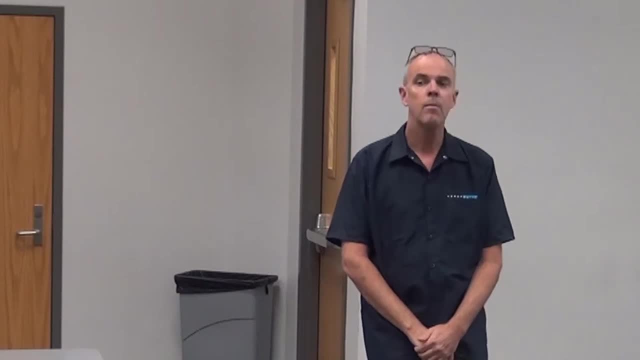 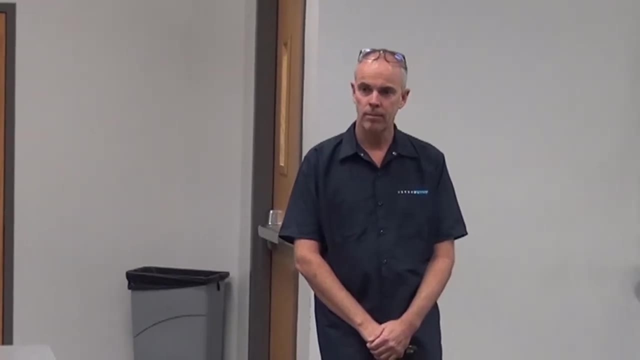 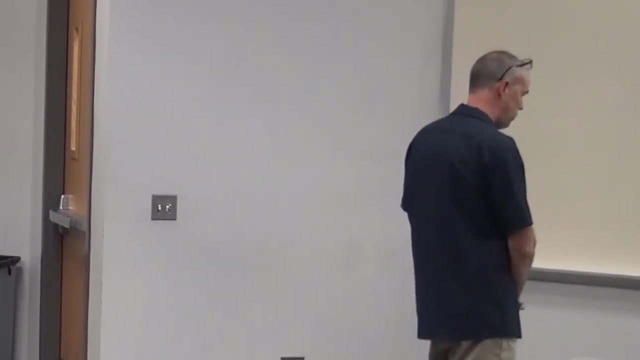 it seems like it's pretty expensive to start that. How, I mean? obviously it would probably depend on what you're making in the market, but how quickly would it basically pay back? That's a great question, So, and it's one I struggle. 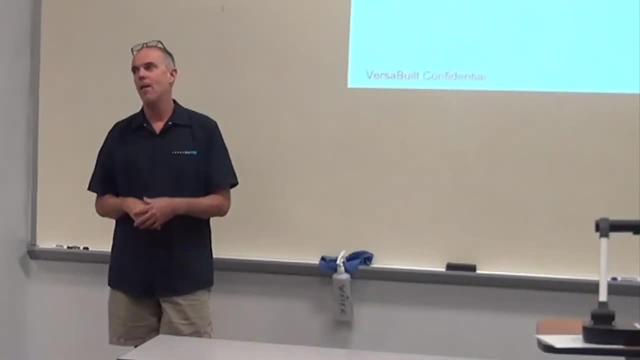 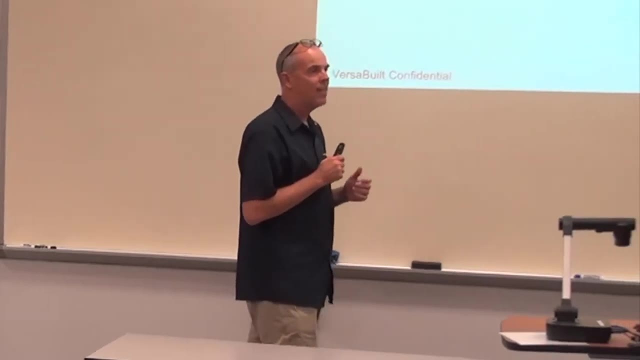 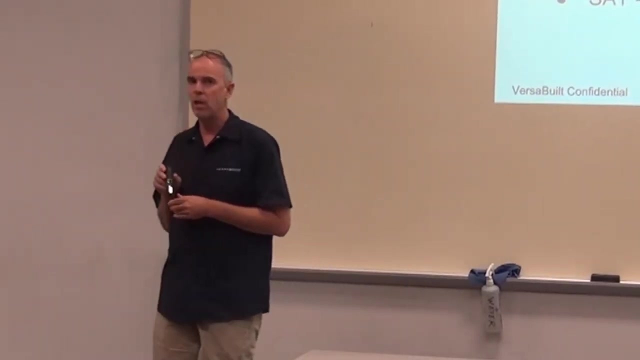 with teaching potential buyers of our equipment all the time. So you have a typical laborer. in the United States there's about a million people that are employed loading, unloading or setting up CNC machines. Does everybody know what a CNC machine is? The average loaded cost of that labor is $22 an hour. A typical CNC machine is $100,000 to purchase. So what do you think is more expensive, The guy loading it or the CNC machine? It is So how much. Like 20% more, 50% more, twice as much. Okay so typical CNC machine in the United States the average age of a CNC machine is 15 years. There's 87,868 hours in 10 years, So let's say 120,000. hours or so At the end of that machine's life. it still has some residual value, maybe 5 or 10%. But if you look at the total cost of that machine over that lifetime it's probably on the order of 60 to 70 cents. 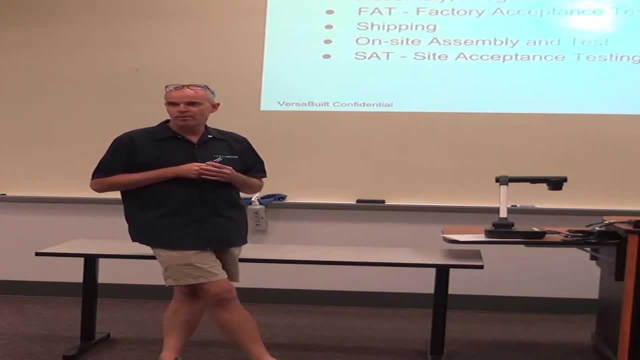 per hour. The operator's $22 an hour. It's significant. Most people- and I'm talking about you- know I'm working with a company that acquired my last company for Cruise Motorsports. You talk to those guys the way they have their current production. you would think for sure that 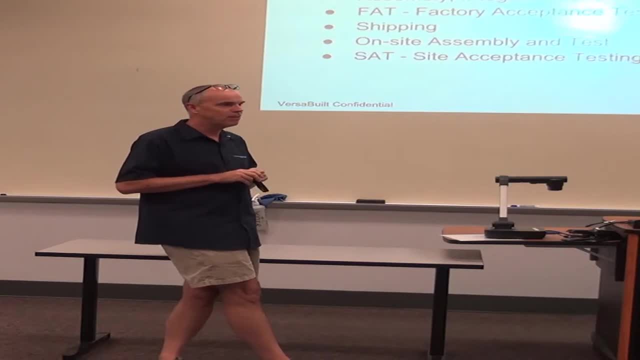 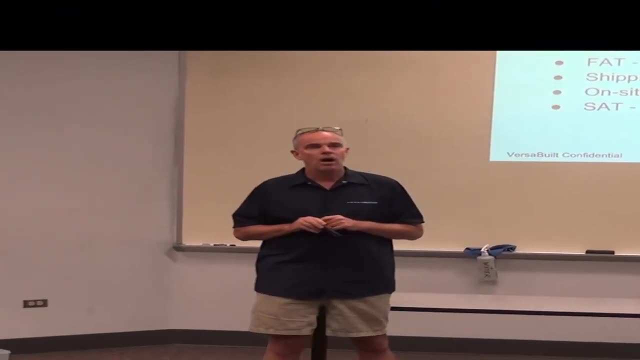 they think that their machines are worth 5 times as much as their people. They don't get it And their machines- their average age of a machine in their shop is probably 20 years old. So people are pretty expensive Equipment's pretty. 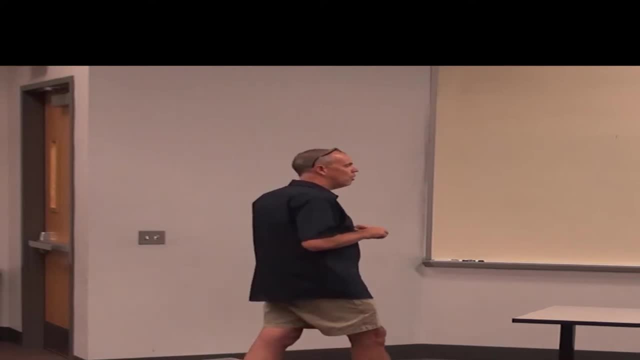 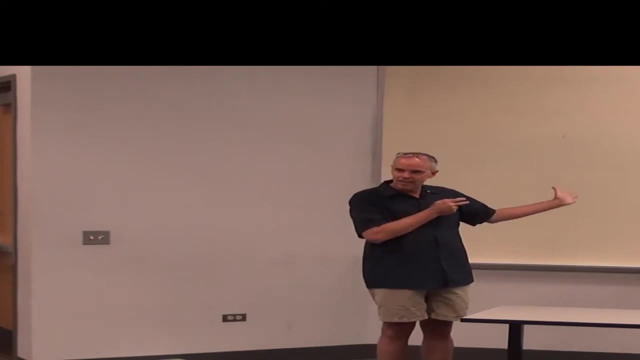 inexpensive. So that's one of the key drivers, but it's also one of the. I'll kind of get to this as the presentation goes on. but today, if you looked at that system that we just looked at there, let's say you actually had 10 different part numbers you needed to run. 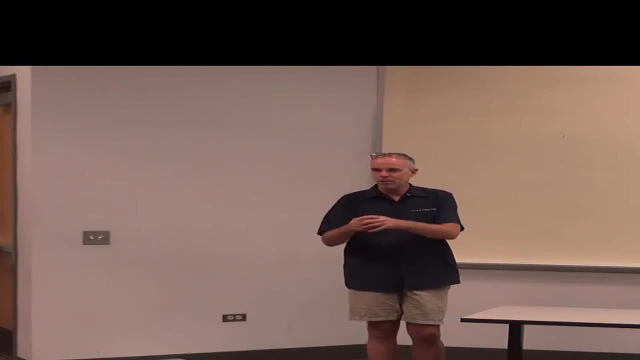 You know, from a quarter inch up to 3 inch, to this to that. You can imagine, even if you engineered it right from the start, knowing how to do all those things, if you needed to run, go from the quarter inch part to the 3 inch part, it may take 2,, 3,. 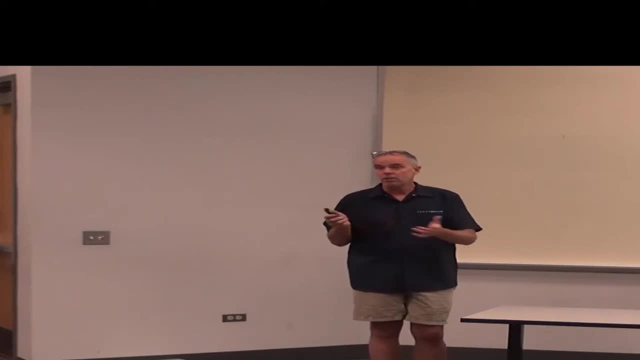 4 hours of setup. Maybe it might take 2 days of setup to transition from making it a one part to the next part. And again, as we talk about high mix manufacturing with lower volumes, that's unacceptable. People are cheaper. People are really good. 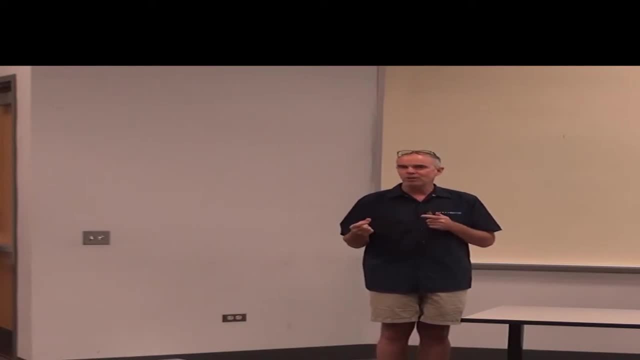 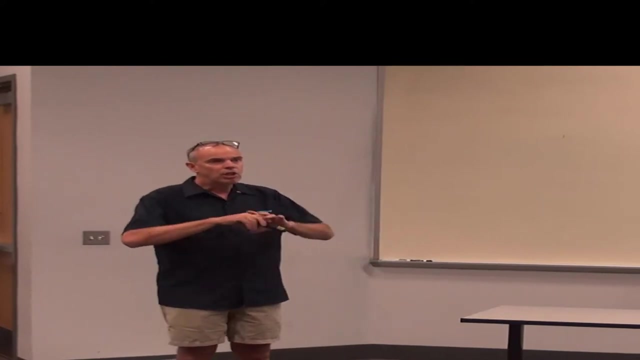 at quickly changing over things. They're not really good at doing things repeatedly like machines are, but they're really good at being flexible and adaptable And that's been a big inhibitor in the widespread adoption of industrial robotics. If you look at all manufacturing, if you look at all 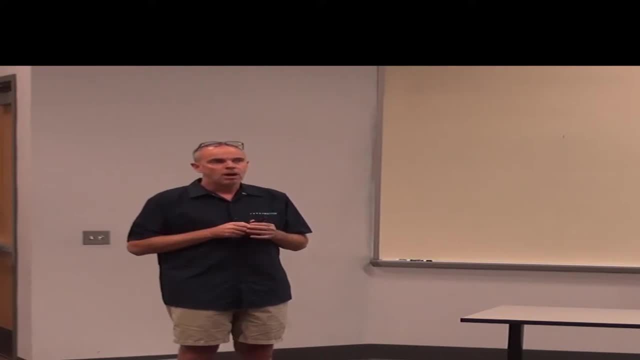 manufacturing machines and CNC's in particular. I was really shocked at this. I thought that if you looked at all parts made in the world and all CNC machines that are in manufacturing in the world, I thought at least 50% of them would be involved in high volume. 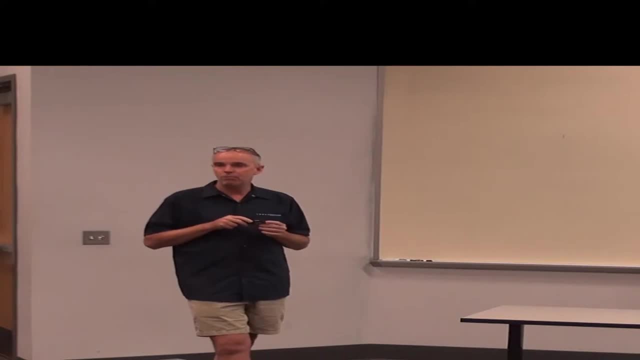 no mix manufacturing. The actual number is less than 10%. The vast majority of CNC machines are making in the United States. the average batch size for a set of parts that goes through a CNC machine is 50 pieces, And that's why 95% of them are still loaded by people. There's more than 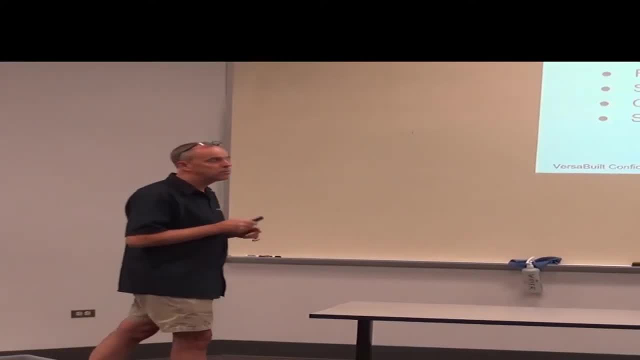 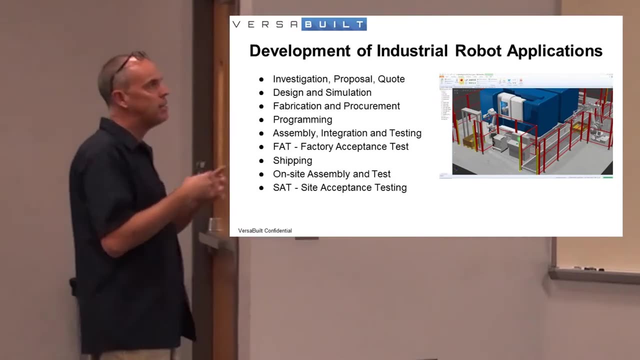 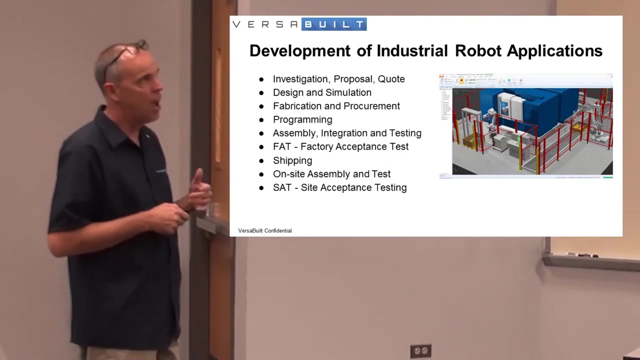 a million people employed running CNC machines than the rest. So real quick going back to the traditional system integrator model. how does it work? How do these things get deployed? There are some pretty good software tools out. Each, every single major robot vendor has. 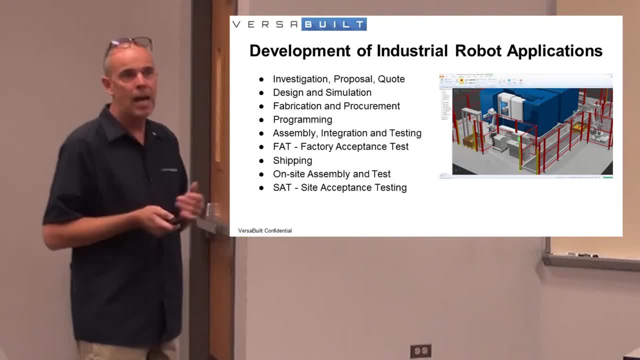 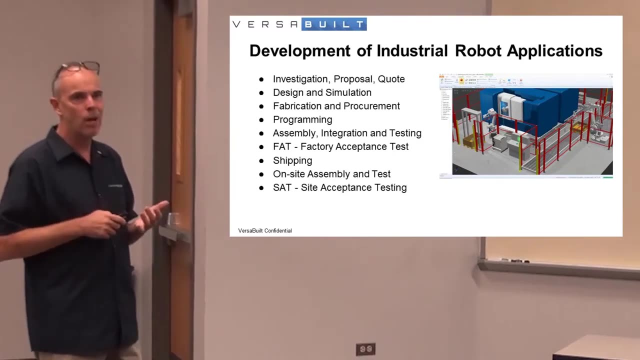 a piece of software like this. It's a pretty advanced CAD kind of package that allows you to simulate and program the robot, And they keep getting better and better. They're still all closed architecture, all proprietary, So they're not moving as fast as, say, Microsoft Visual Studio or some of these. 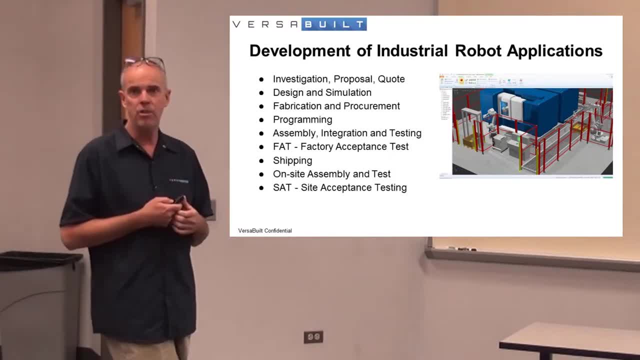 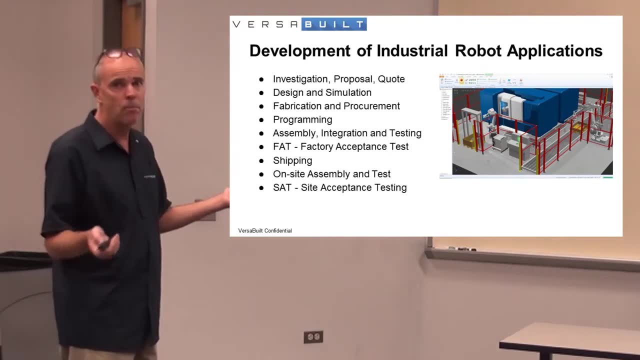 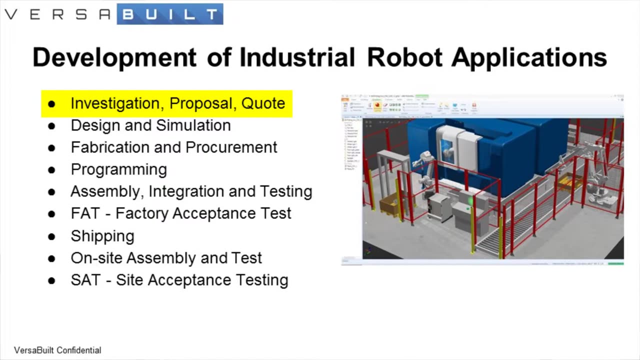 open source development applications and frameworks that you've seen in the general software world. But generally the way these things get deployed is: customer has a problem, calls up an integrator and you have these kind of phases of the project. First is investigation, proposal, quote, Then design and simulation. 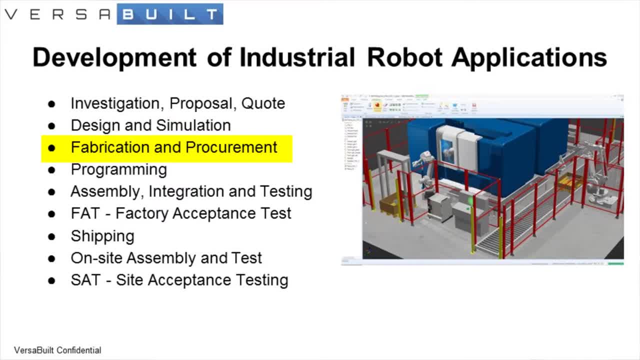 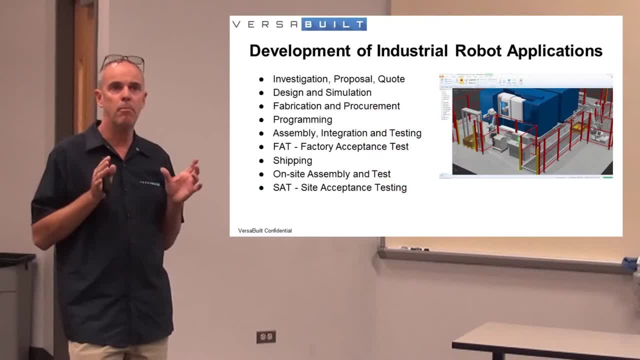 make sure everything's going to work. Then fabrication and procurement. If you look at the way these things are deployed, they are primarily assembled from off-the-shelf components that have little tiny tweaks to them. What robot system integrators have learned is that 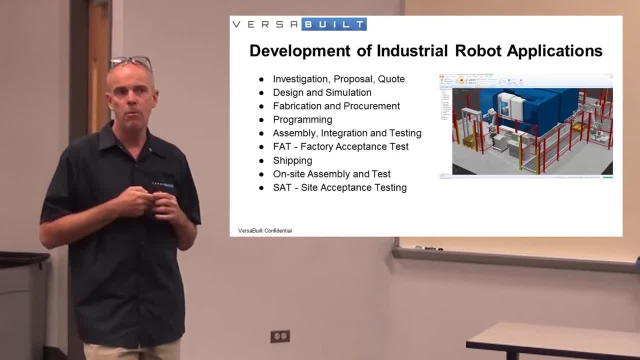 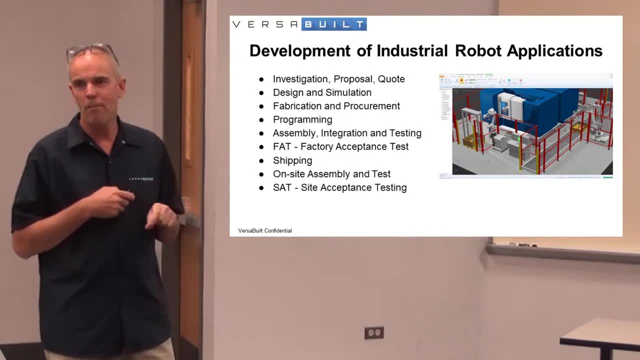 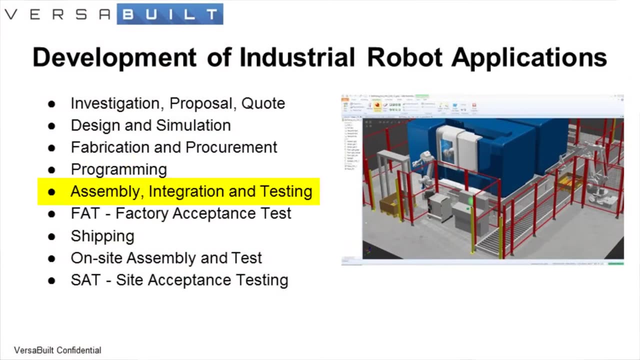 if they try to invent things, they usually fail. So understanding where to find and procure the right solution for the problem is a really important part of that job- Programming, assembly, integration and testing- And that's typically done at the system integrator's site, not at the customer's factory. 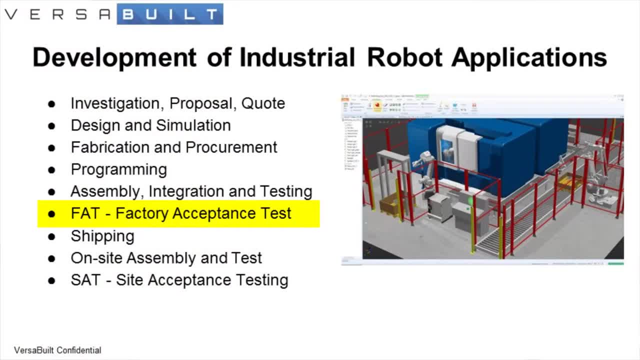 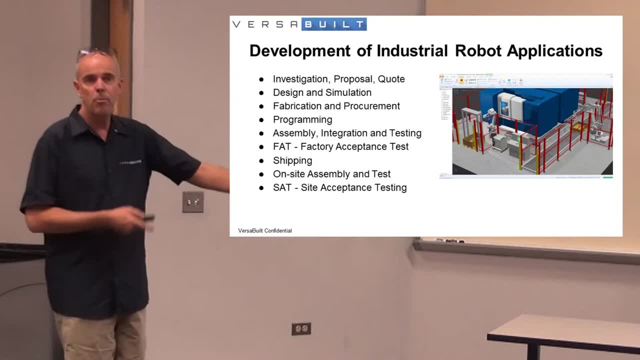 site. And then they have what's called a factory acceptance test where, after the system integrator's pooled everything together, maybe got some raw material and able to run some parts, they bring out the purchasers of the equipment and say here's the specification. 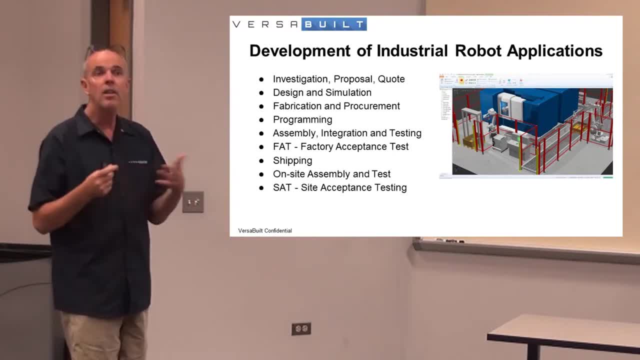 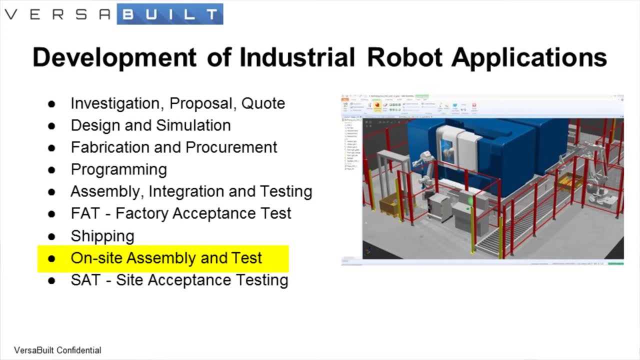 see we're meeting it, it's working reliably And they sign off on it and usually get some significant progress payment. Then it's got to all be packed up and shipped. Then there's on-site assembly and test And then they'll do some. 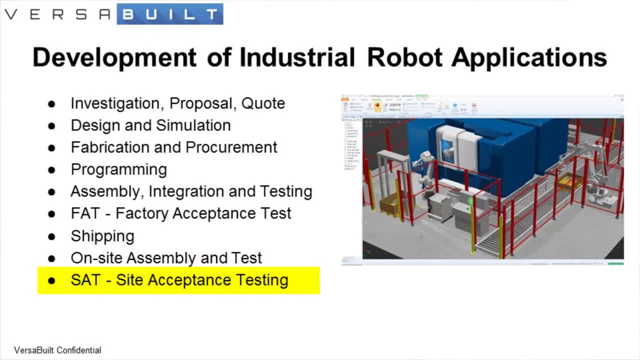 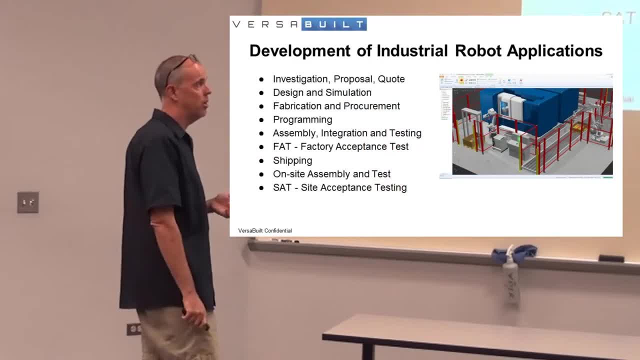 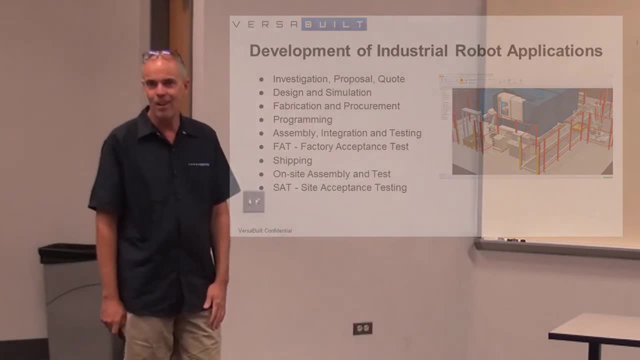 run-offs there until they get to what's called a site acceptance test, And once that site acceptance test is complete, that's usually when the remaining balance of the purchase order is paid for. But from my perspective this is a really inefficient system. You do all this work, you build it up. 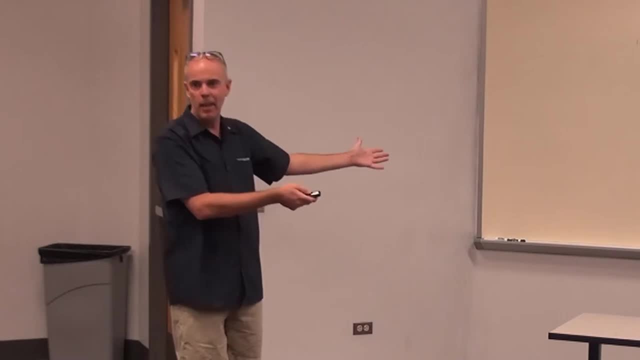 and you tear it all down and you ship it over and things break and you build it all up and try and make it all work. That's part of the reason why, if you look at this market also, system integrators are very regionally. based. There's not these giant system integrators that are in one location and they do things all over the country. It's partly because you need to have things on the ground, very near the customer's equipment, So when there's problems you can respond very quickly If you've built a several million. 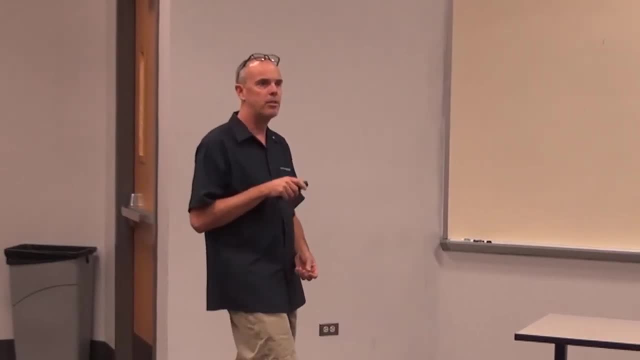 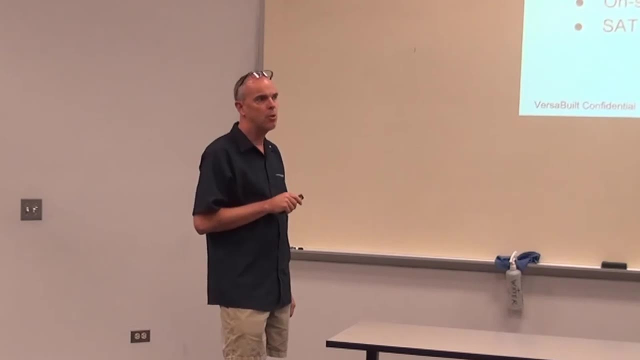 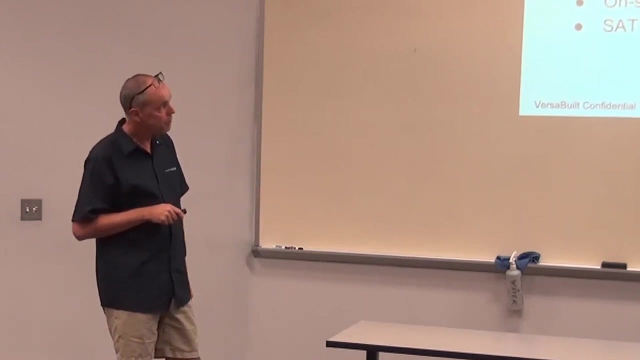 dollar robotic system that's running production and it goes down. the cost of being down can be extraordinarily high. It's also why the liabilities of robots are so important, Which brings up another thing about the robotics market: When a robot does break, these things are pretty reliable. Published meantime. between failures of about ten years. My experience is more like two or three in the first year and then after that. they tend to be pretty reliable, But when they do go down, you can generally get service within 12 to 24 hours. The cost to repair that robot is typically very near the cost of the actual robot. But people are willing to pay for it because they need it now. They need it right now If the cost of that line being down is $10,000 an hour. 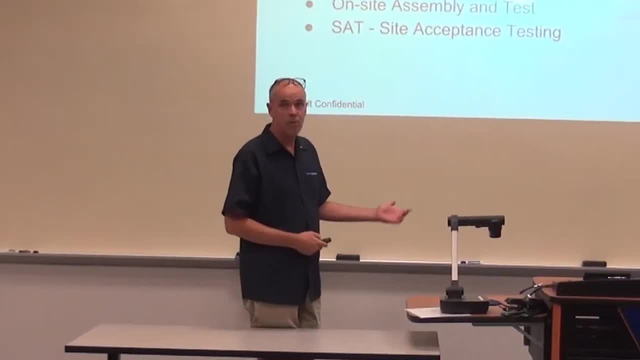 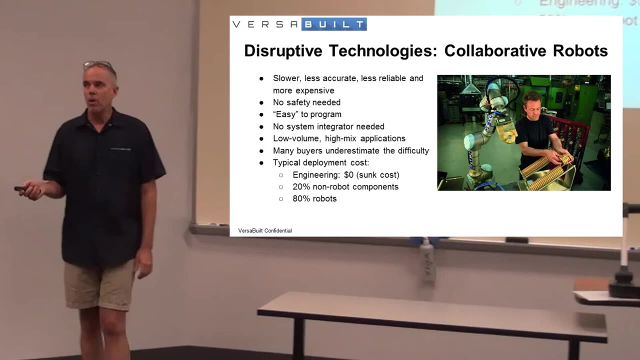 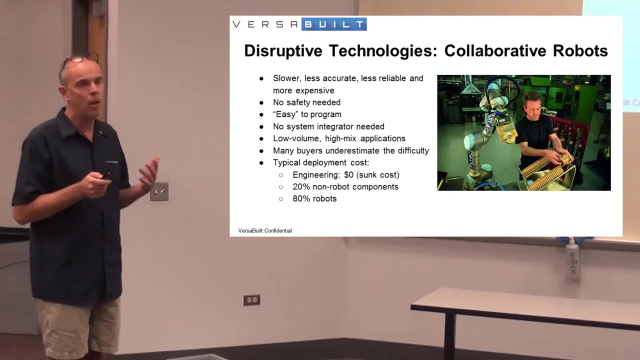 people aren't going to whine very much about paying a $30,000 to $40,000 bill to repair it. So what are some of the things that are happening in the robotics market? Again, I'm limiting this to industrial robots that are really changing the market and will have. 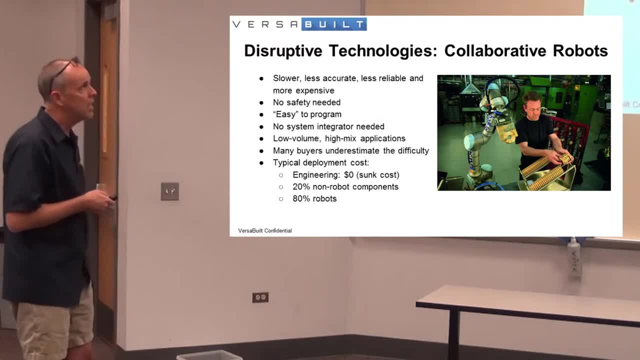 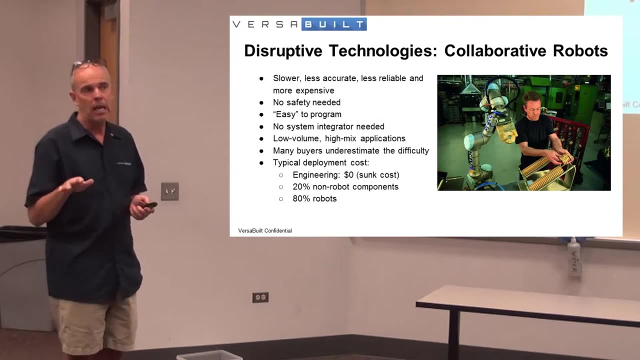 a significant impact. So the first thing is collaborative robots, or co-lots, And collaborative robots, by definition, are robots that don't require safety systems to be operated in an industrial environment. What that means is a person can operate right next to them. 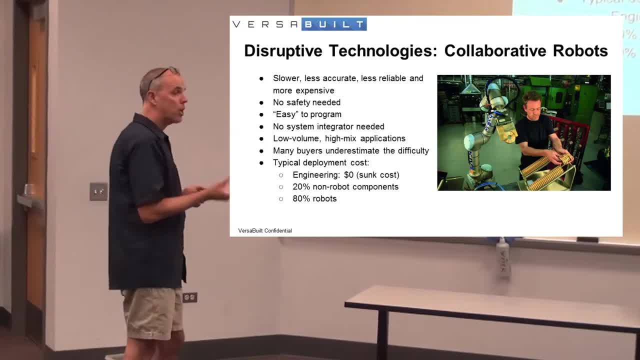 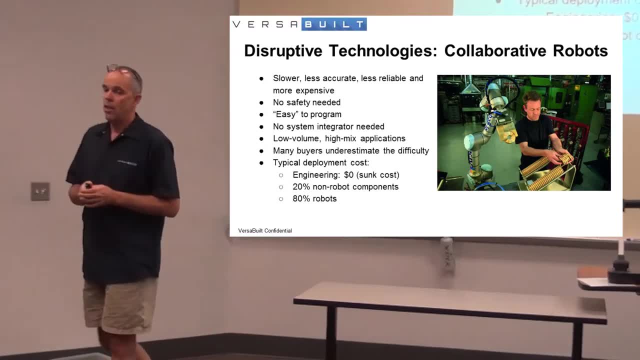 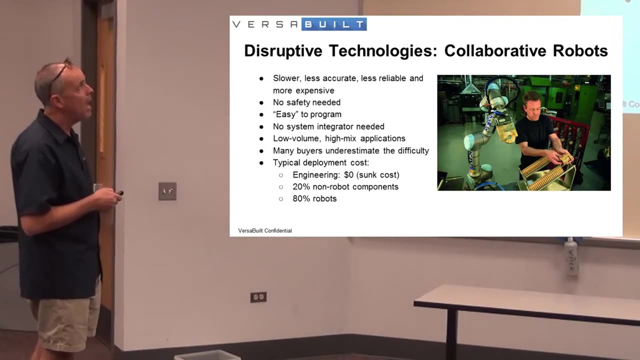 These robots have very sophisticated torque sensors in them so they can recognize if they've bumped into someone. or if they've bumped into a person, They generally are much slower, much less accurate, much less reliable and more expensive than industrial robots. That sounds like a losing proposition. 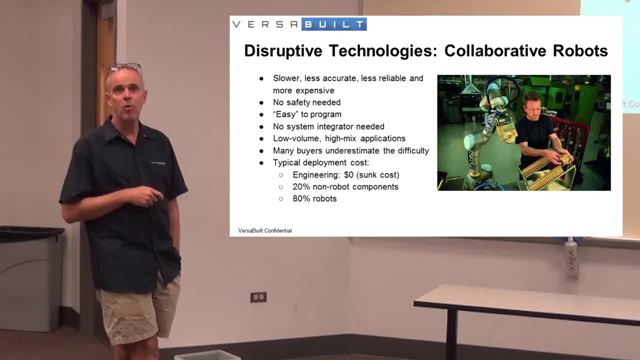 doesn't it? It's by far the fastest growing segment of robotics. I think my perception- and we're actually going out and doing some market research- is that the success of collaborative robots has about 20% to do with that. people can work around them and you don't have to build a safety system around them. 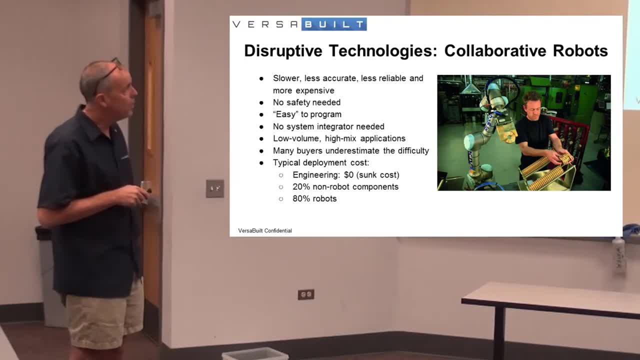 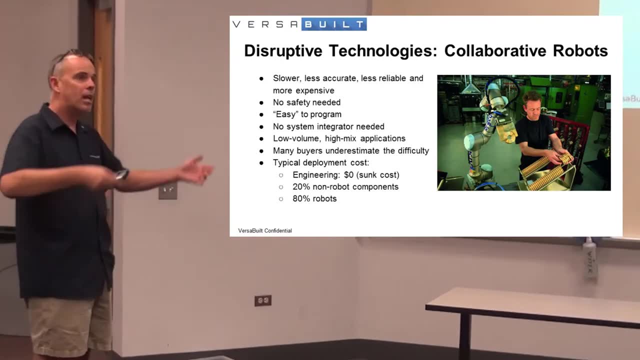 It has 80% to do with the perception that they're easy to program and I don't need a system integrator. I don't have some guy coming in waving his arms in front of a whiteboard proposal talking about hundreds and hundreds and hundreds. 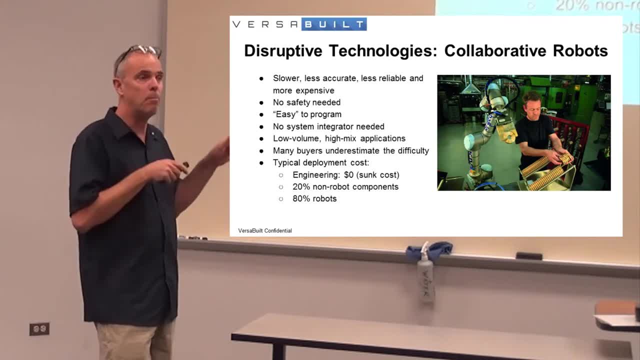 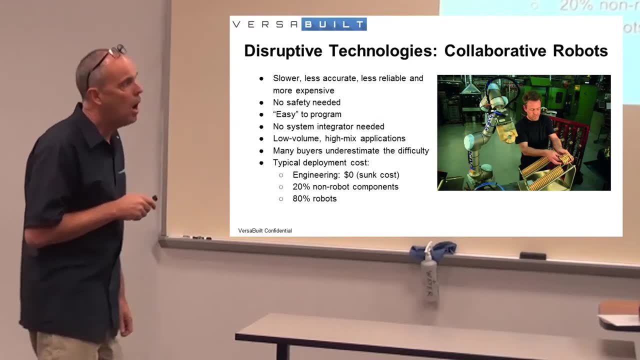 of thousands of dollars or having my entire business be dependent on this system integrator. If it goes down and I can't ship product, I could be out of business. That, I believe, is what is the primary driver for these types of robots: Universal robots. 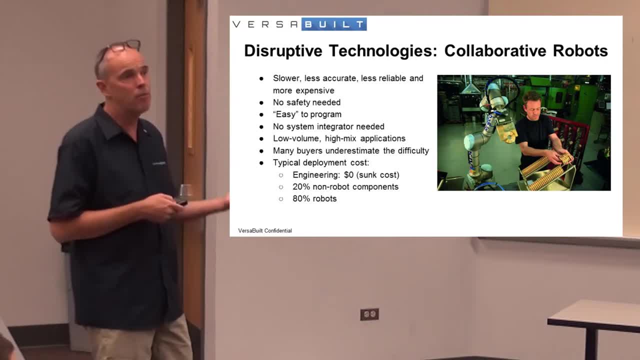 is really the leader in this market. You've probably maybe heard of Baxter. It's a little bit more of a toy That works around industrial robots. This is a toy to me, But they're very, very important in the market. Really, if you look at where. 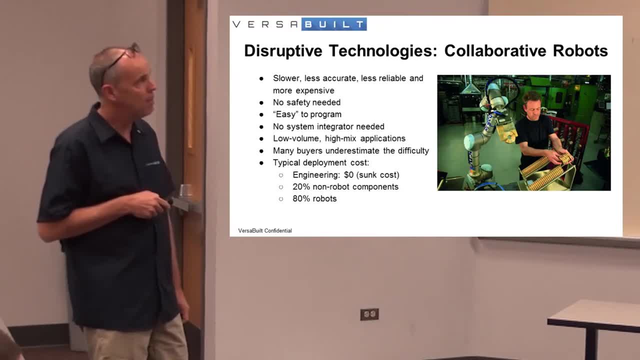 they're being deployed. they're starting to be deployed in low-volume, high-mix applications. You can see this guy's got a little infeed system that he probably built himself here. He's got a little gripper that works for that. But if he needed, 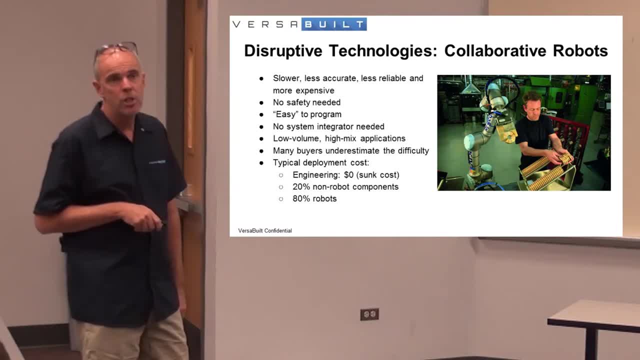 to change from making that maybe three-inch round part to a four-inch square part. he could probably figure it out in two or three days' time and do it himself. He wouldn't have to wait six months to have it done Or call in the system and go: oh, we need a change. 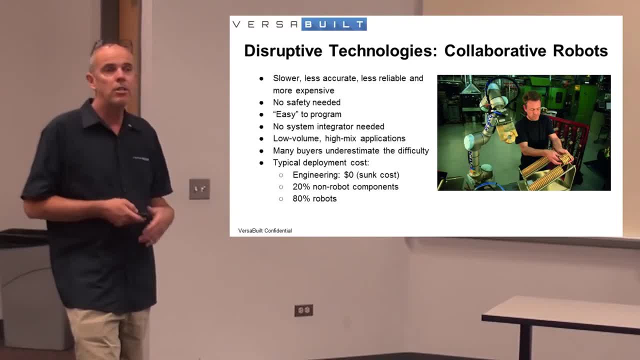 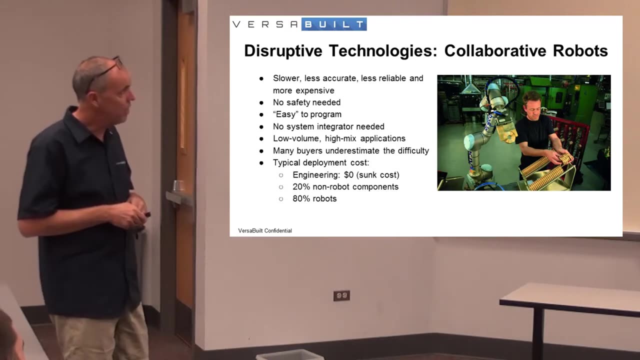 We'll start with a change order That starts with $10,000.. These are going to be some of the key drivers that start to push robots to broader applications outside of those traditional high-volume no-mix applications. I would say that I've talked to a lot of buyers that underestimate 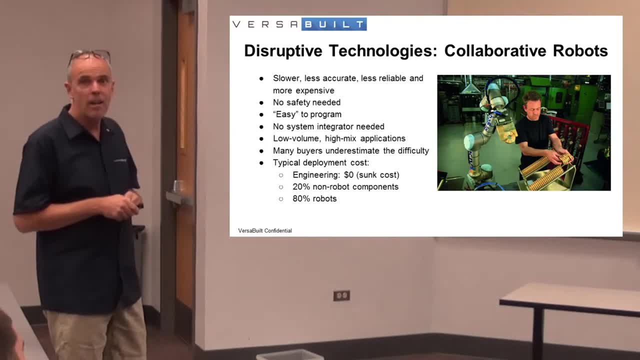 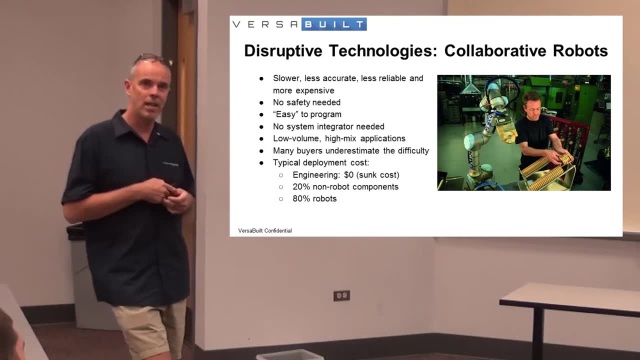 the difficulty, They finally figure out how to make it work, but it's usually a smaller scope below their expectations and it took a lot more work than they expected. Have any of you taken any process engineering classes yet? You should. Process engineering is important. 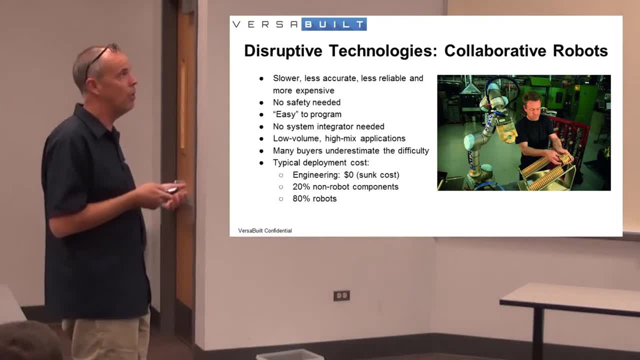 It's a great kind of education in general, But this guy probably has never had a process engineering course and so he will learn it the hard way. Go ahead. What kind of companies are using this type of robot? All types of companies. 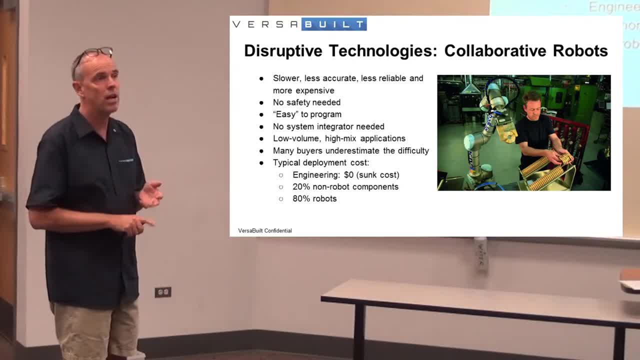 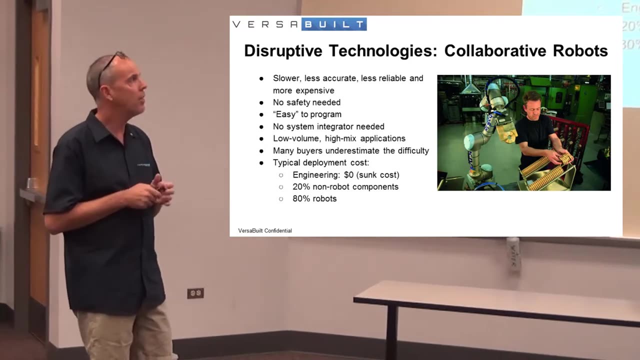 Aerospace contractors, medical device contractors- you see them in kind of smaller volume electronics assembly type of applications, Mostly pick and place. I don't think I've ever seen a universal robot deployed in a welding application. I'm not sure it could actually work in a welding application. 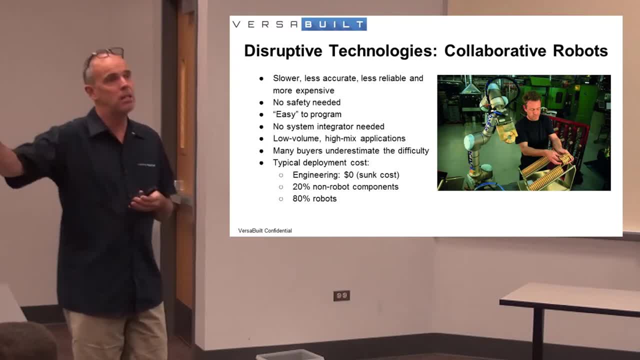 They're not real accurate. so dispensing applications like glue or caulking or something like that, they're probably not going to perform as well. They're mostly targeted at the pick and place market, So engineering costs most buyers are going to consider. 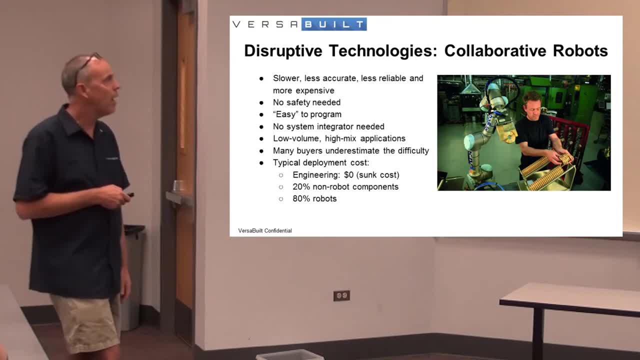 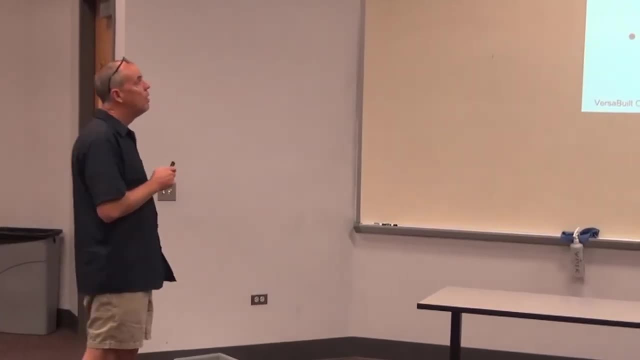 it to be zero. Just have Tom, He'll figure it out. Maybe 20% of the total cost of the system, or even 10%, will be non-robot components And most of the cost will be the robot itself. So this is kind of a. 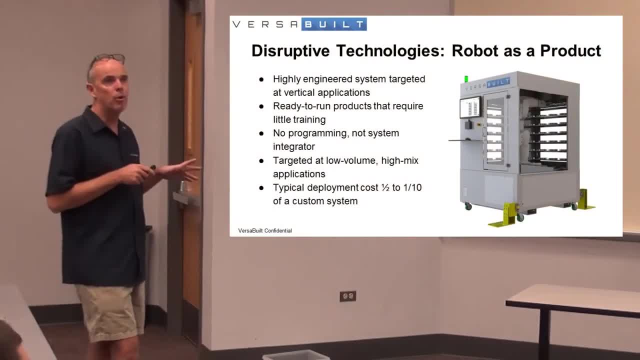 I'm not trying to pitch you guys my product, but this is the space that we're in. I think it's another space that is finally starting to see some traction and, I think, will be a very big driver of growth, And that is a robot. 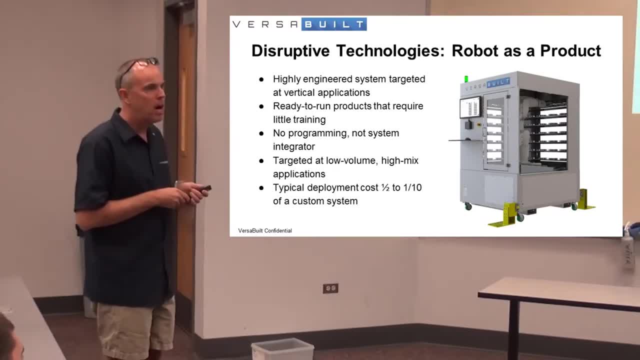 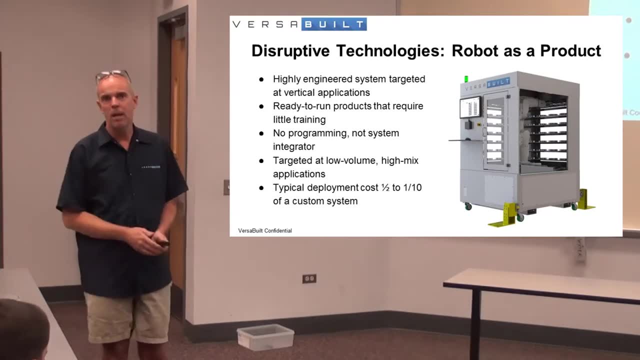 as a product. And what I mean by this is, instead of looking at every application as a new opportunity for something custom and highly optimized for a particular part and making that part as quickly as possible, coming up with a generalized solution to a vertical problem. So when I say vertical problem, the vertical 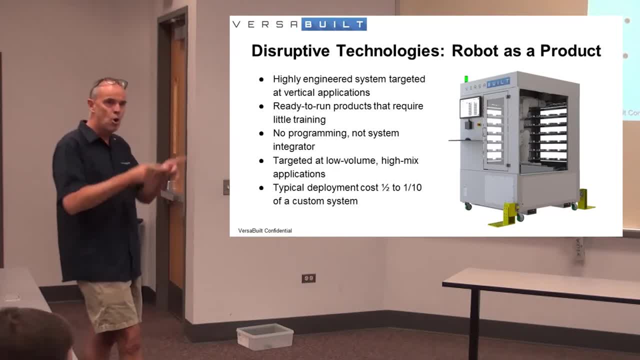 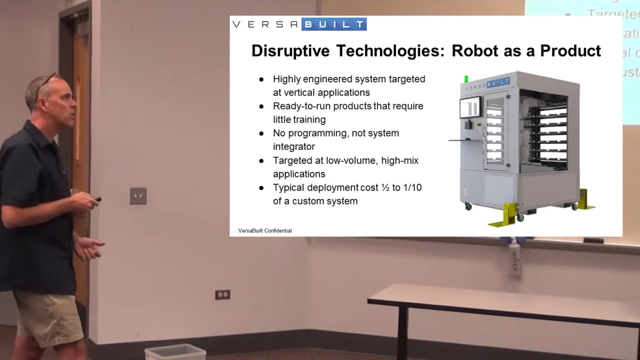 problem that we're trying to address is CNC manufacturing. We're not trying to solve the problem of CNC manufacturing and welding and glue dispensing. We're just focused on CNC manufacturing, And the area of CNC manufacturing that we're focused on is low volume, high mix. 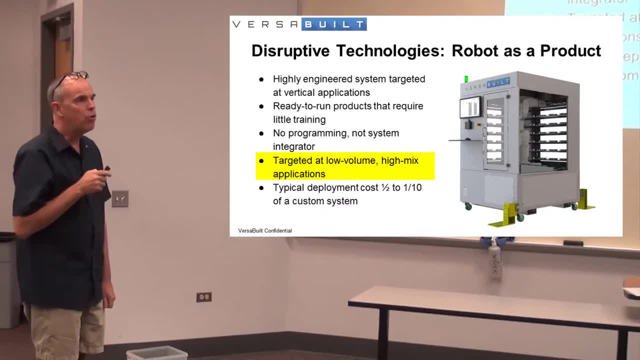 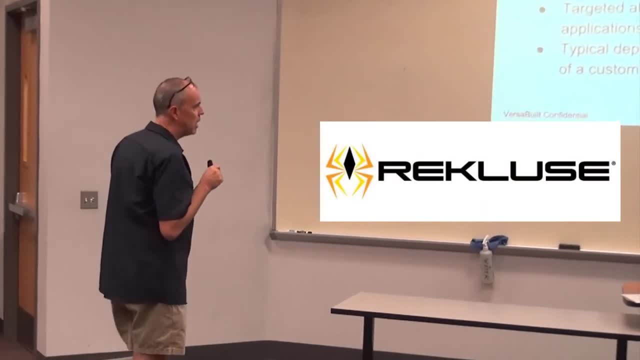 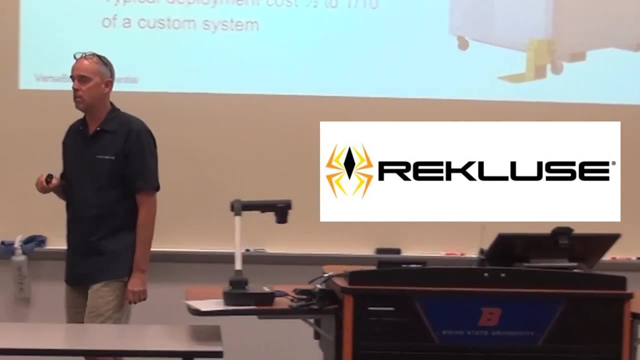 So if you look the way I got into this business is Recluse Motorsports' growth was being constrained by our ability to ramp up, during our busy season, the number of operators we needed to run our business. It doesn't seem like the right thing to do. We brought in a system. 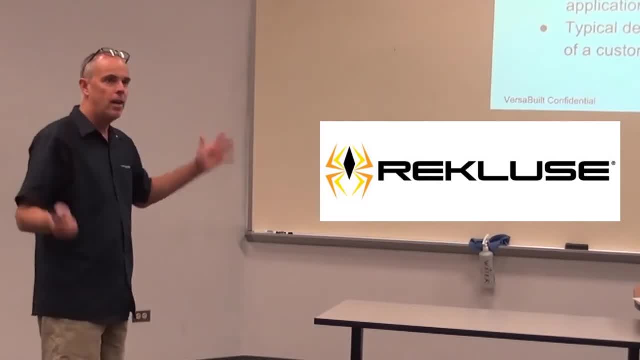 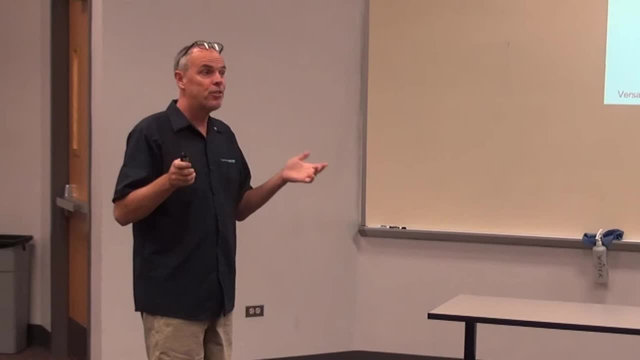 integrator and they waved their arms around a lot and came back a month later with a proposal for well, let me back up for a second. I first said: hey, we have 250 part numbers, Here's the different families. And the guy literally laughed at me. 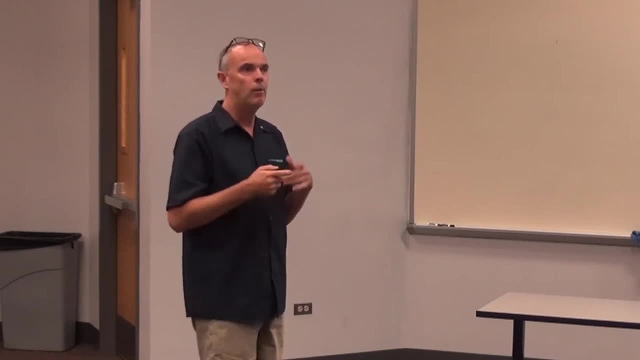 He said: we can't do 250 part numbers, We can do one part number. What's your highest volume part number? So we gave them that. They came back a month later with a proposal. It was about $300,000.. It was going to take nine months to deploy. 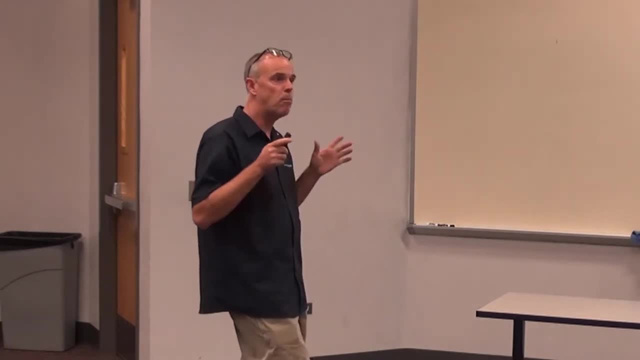 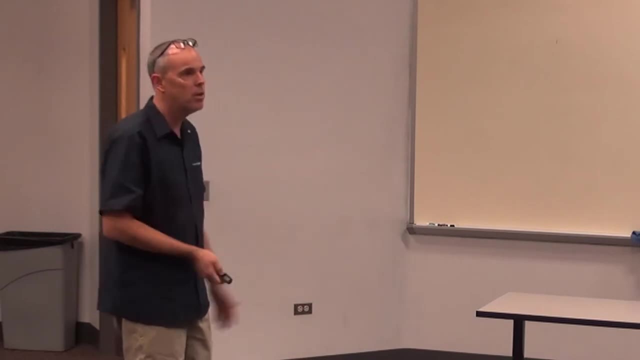 And by the time we had it deployed, we anticipated changing the part by that time in a way that would no longer be compatible with the automation solution that they were proposing. So it made no sense whatsoever. So, like just about anything, I think I can do anything. So we thought: alright, we're going to give this. 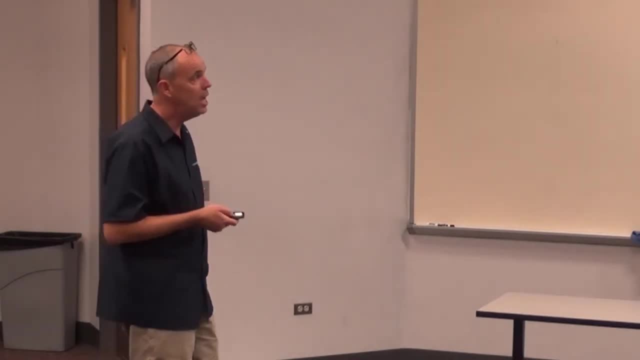 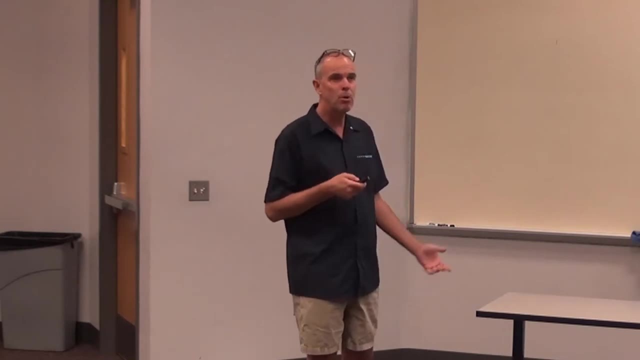 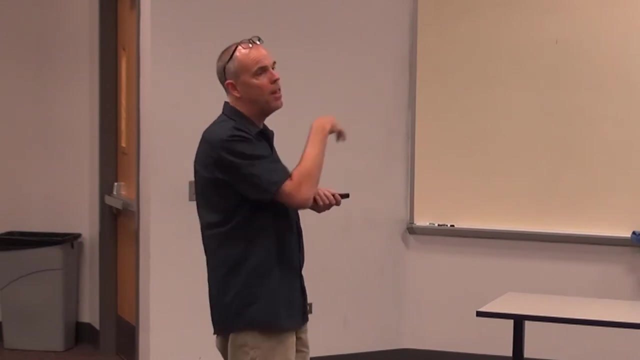 a try And we worked with House of Design And we started developing a solution And we ultimately came up with a technology breakthrough. It's pretty simple. We call it multi-grip. It's how the robot moves the parts in and out of the cell and then also moves the fixturing that holds the part. 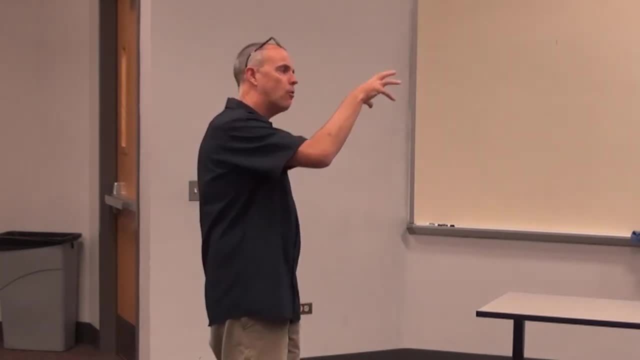 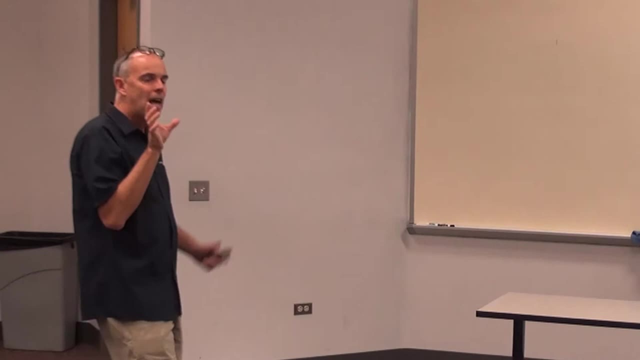 in the CNC Where other applications, the robot has fixturing to pick up the part, The CNC has fixturing to hold the part in the CNC. With our system that fixturing that holds the part is used by the robot and the CNC And that just. 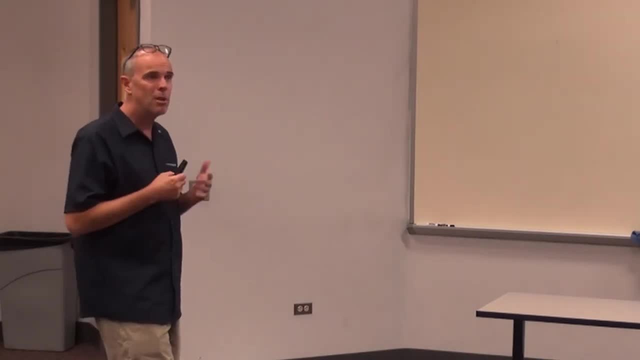 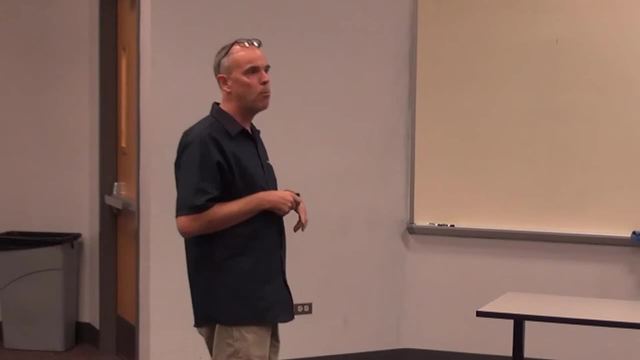 makes everything way easier. It doesn't seem like it would make it that much easier, but it makes it about 10 times easier. If you had a working robot and you wanted to go from making a 3-inch round part to a 4-inch square part, with a typical system integrator it might be $10,000, $20,000, $30,000. 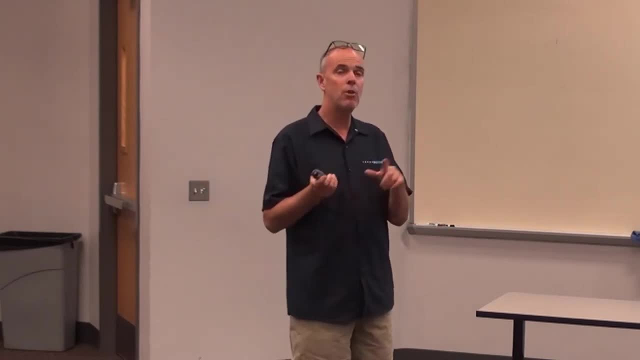 to make that transformation And then to go from making the round part to the rectangular part. for the operator on the floor to do that might take 4 hours, 8 hours, 16 hours to make the changeover to doing those different parts. 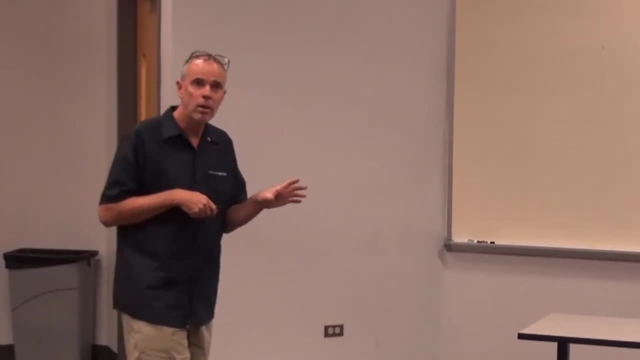 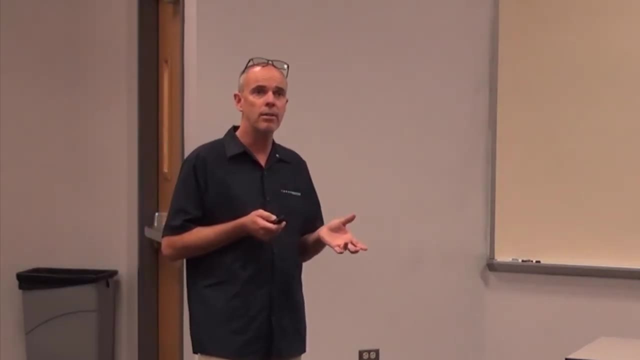 With our equipment it's about a couple hundred dollars to add a new part. It doesn't require any system integrator. It doesn't require any programming. The changeover from making that round part to that rectangular part is about 30 seconds. 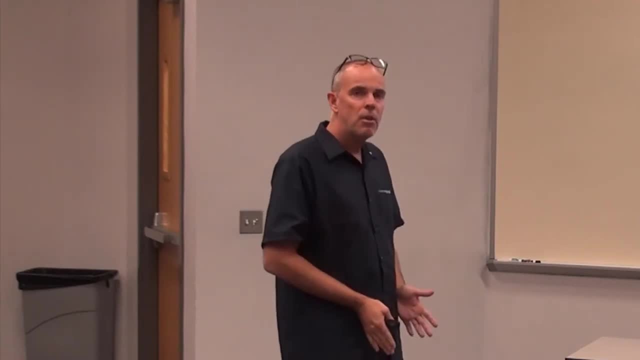 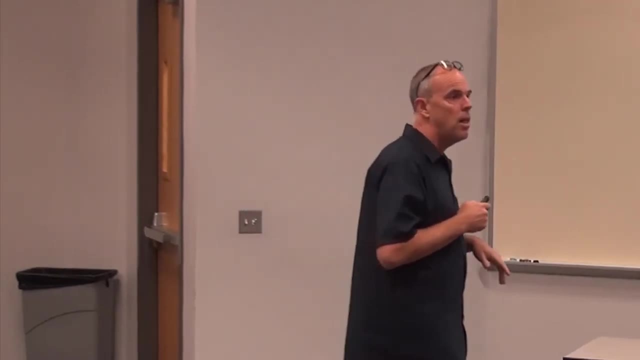 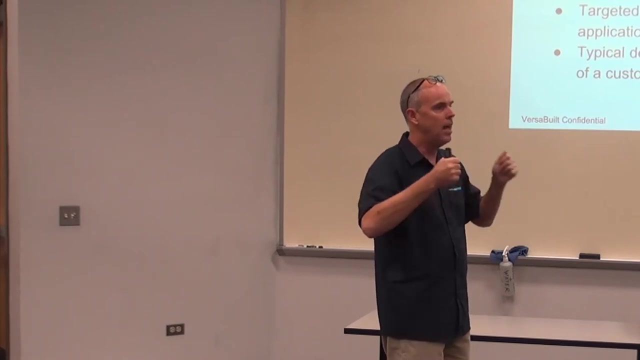 It's looking at some of these opportunities, maybe going into. I met a company that makes a product that fills burlap sacks or dog food sacks And they've got a product that can handle burlap sacks of these standard sizes, plastic bags of these standard sizes. 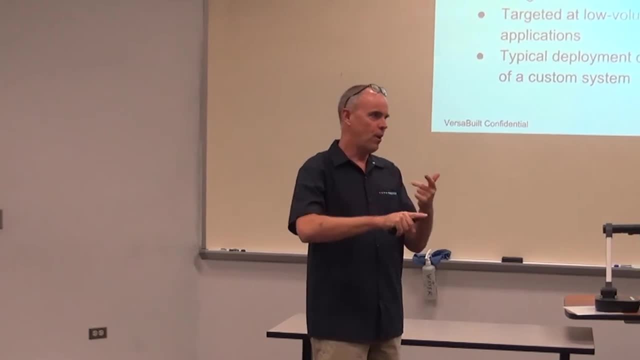 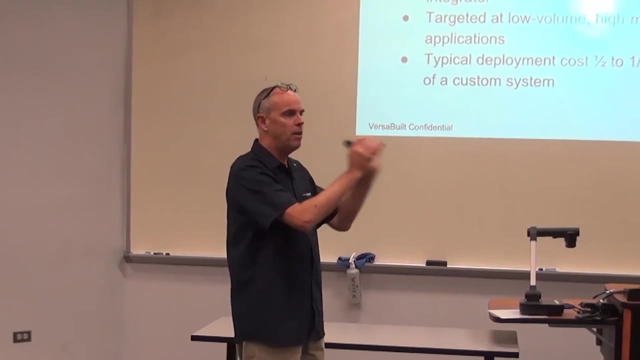 It can handle dog food and grains and various things They've kind of carved out. here's what it can do. Buy our product, You don't need anything custom and you can go from filling dog food one in the morning to filling bird seed. 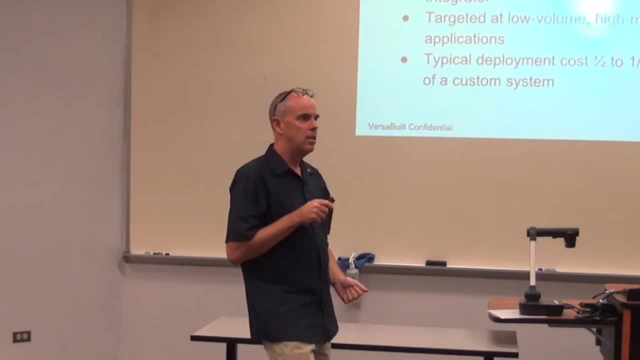 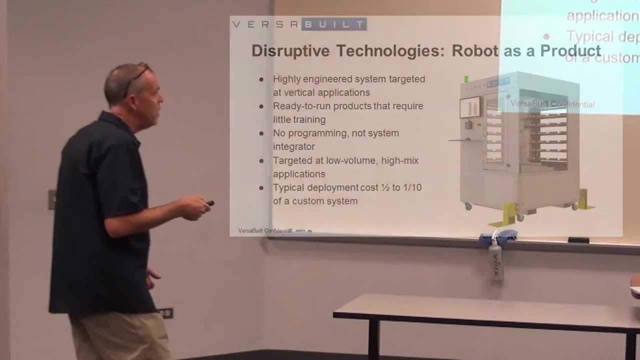 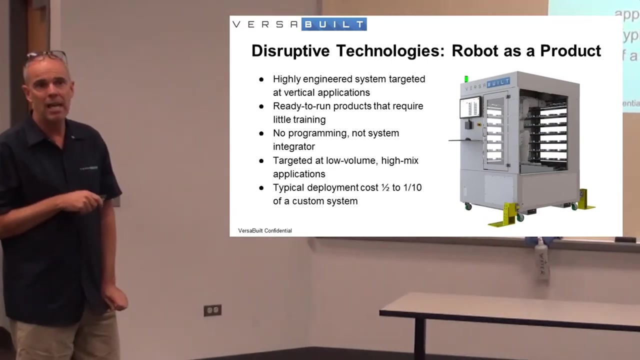 in the afternoon. And those are the type of products that I think are going to really have another big impact on industrial robotics, And this is one of the key things here: That deployment cost and then the cost to actually run it. It's typically one half to one tenth of what it is in a custom system. 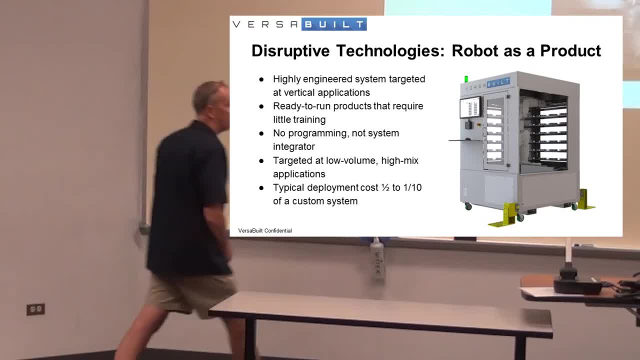 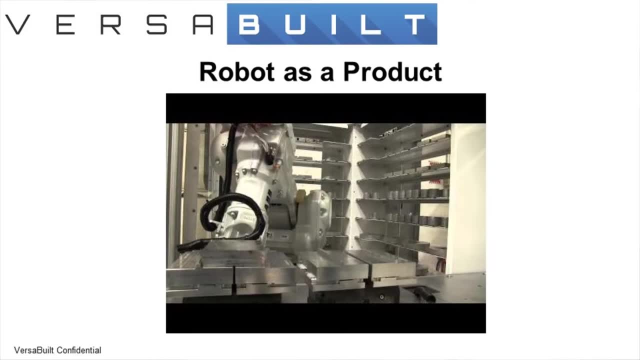 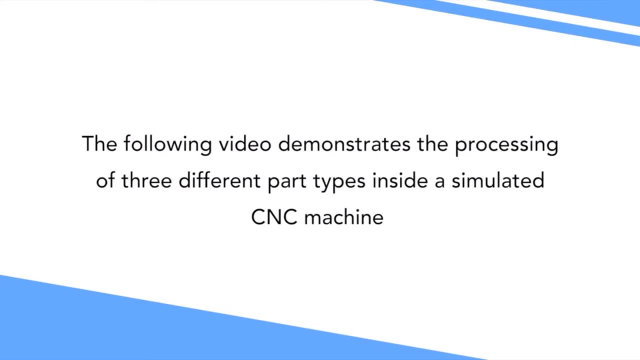 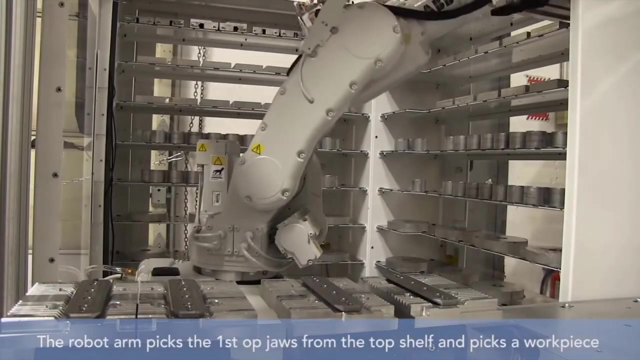 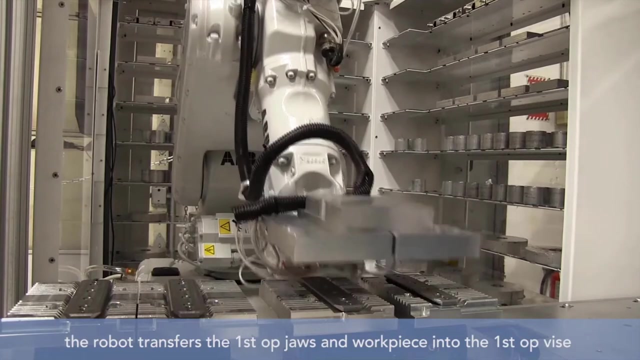 So this is really quickly. This is about a three minute video. It kind of shows our product and what it does. So the robot picked up a set of jaws, Picks up raw material from an in-feed shelf And then it loads it into a vice that would be inside the CNC machine. 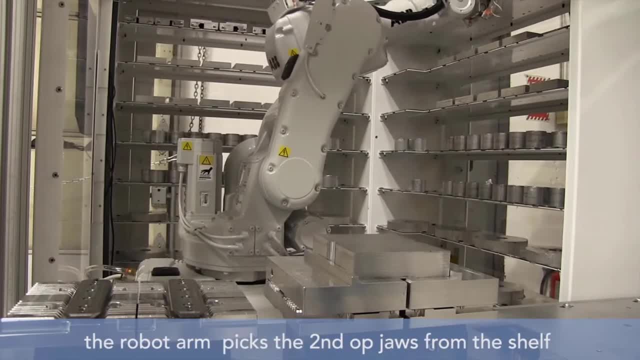 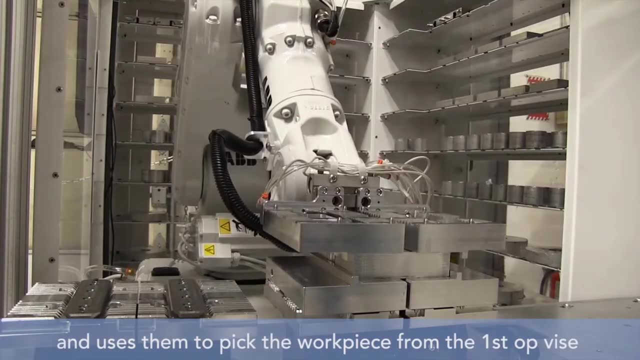 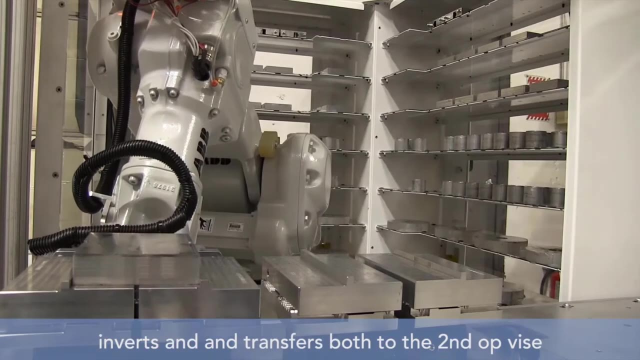 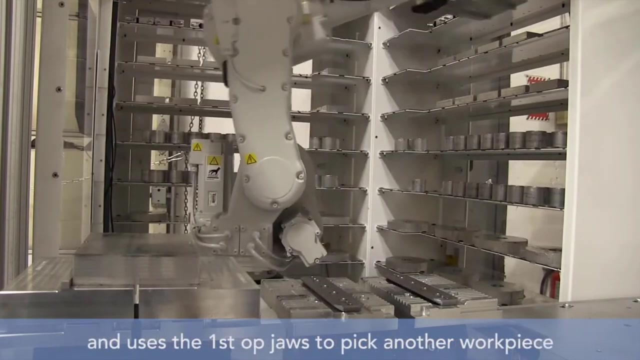 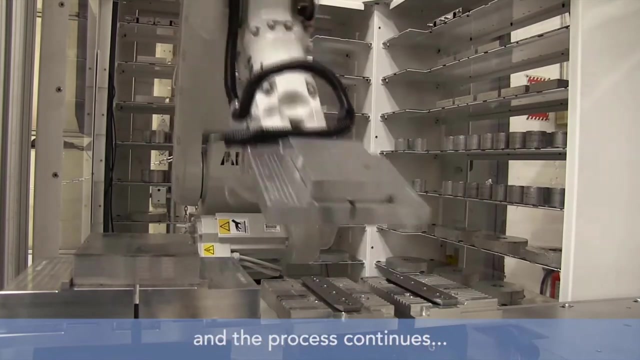 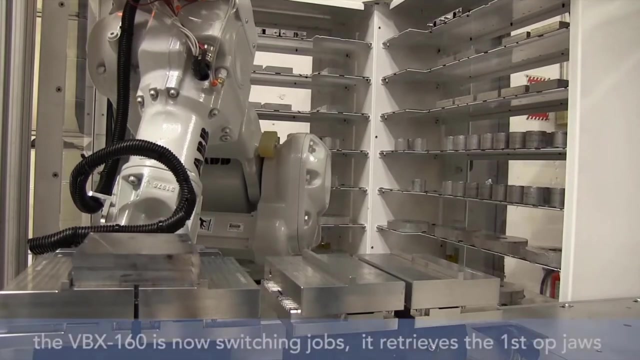 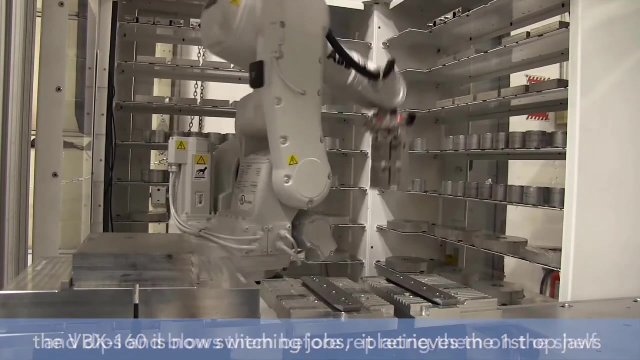 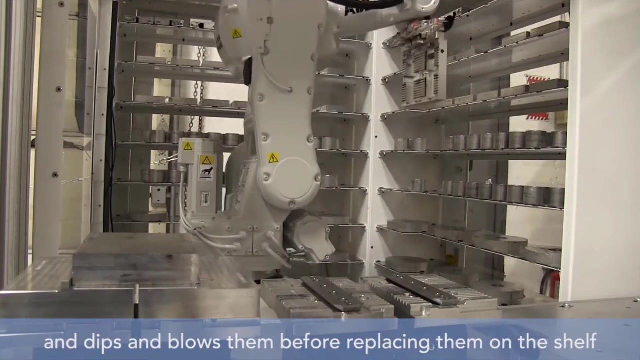 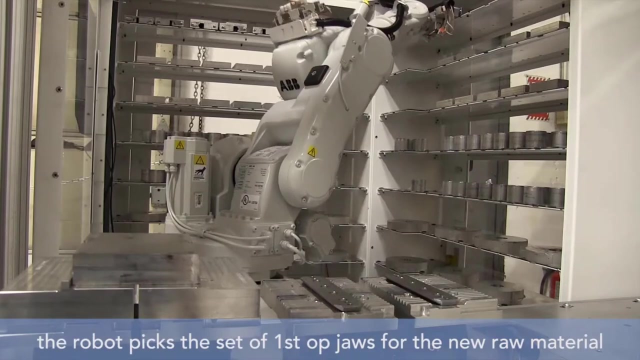 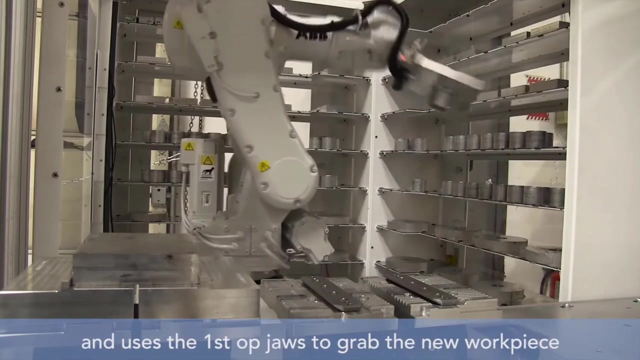 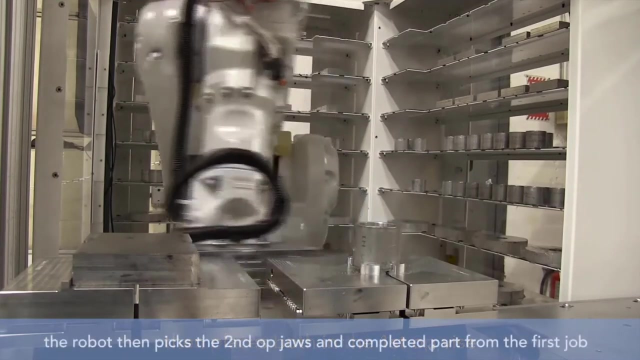 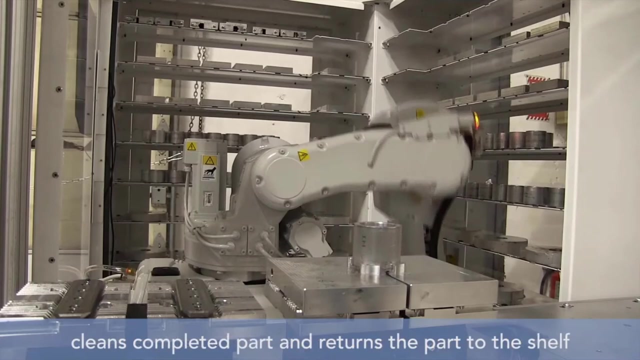 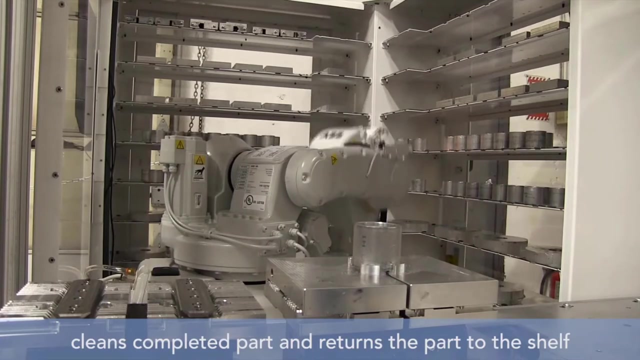 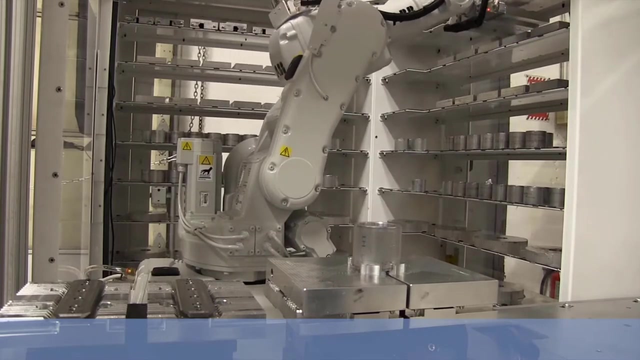 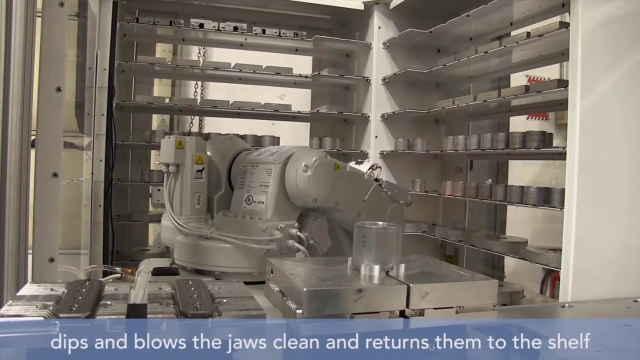 And then the CNC machine would start processing that part. Any questions about this? So how many machines can one CNC machine just typically operate without this? 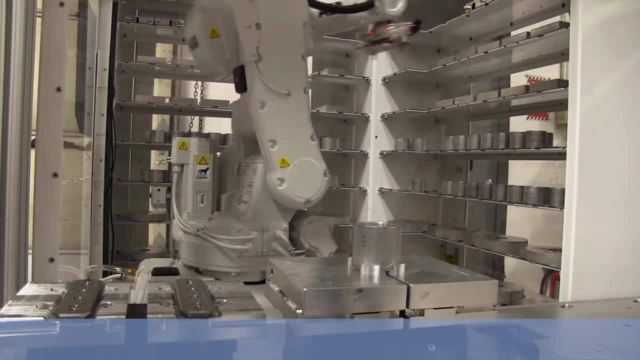 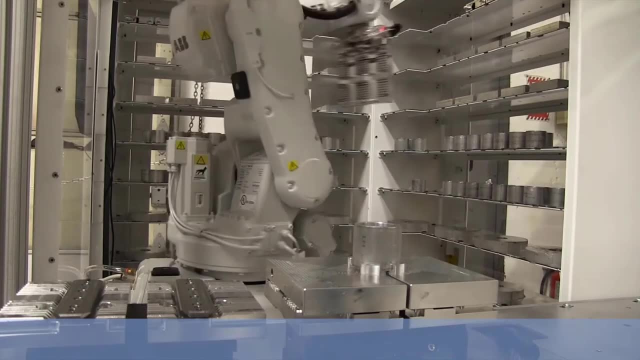 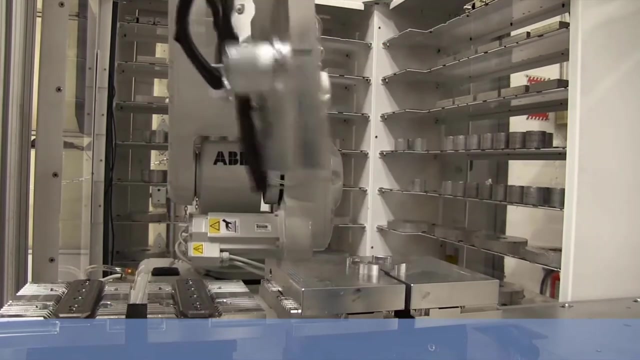 So the average cycle time in the United States per operation is about 15 minutes, between 10 and 15 minutes, And you'd be surprised because you'd think one person, if they've got 10 or 15 minutes, it takes maybe 3 or 4 minutes to open the door, clean it off, swap it over. 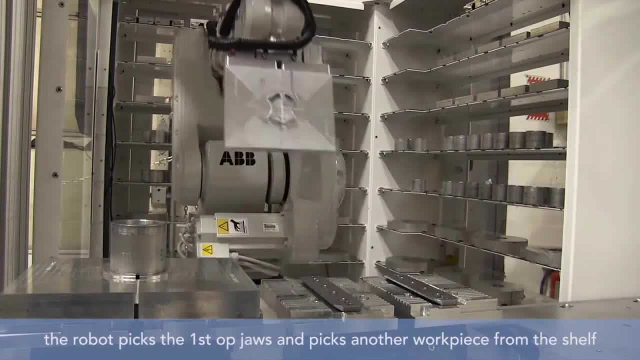 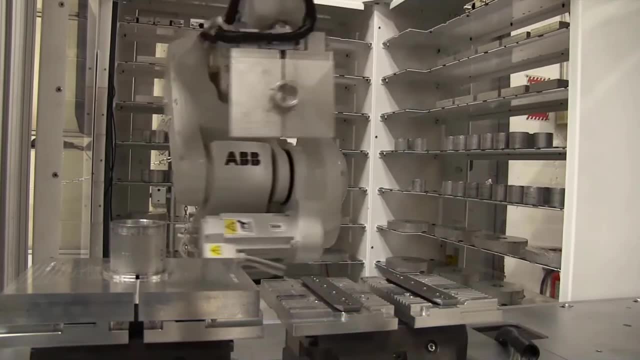 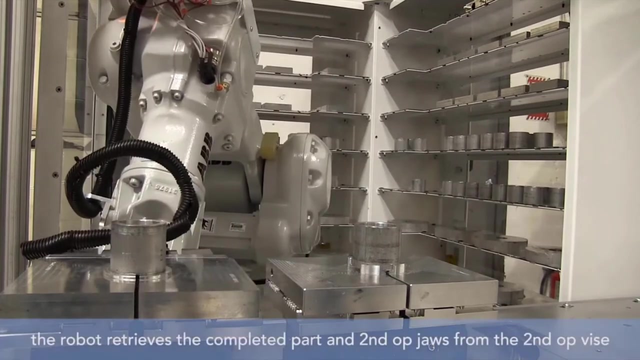 You'd think they could do 3 machines pretty effectively, right? If you have a single operator over the course of an 8 hour day running 2 machines, they'll get about 5 hours out of each machine. If you push them up to 3 machines, they'll get about 3 and a half hours. 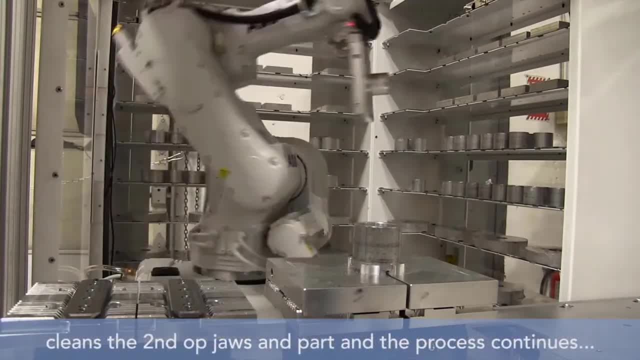 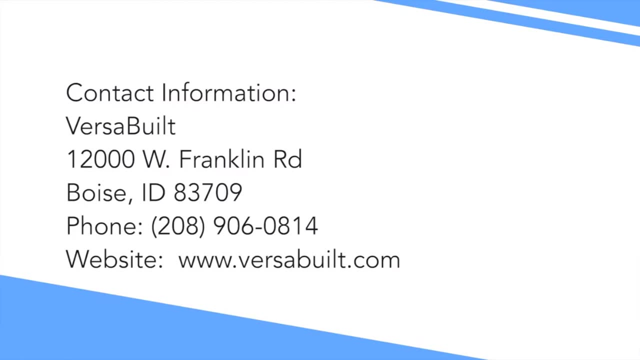 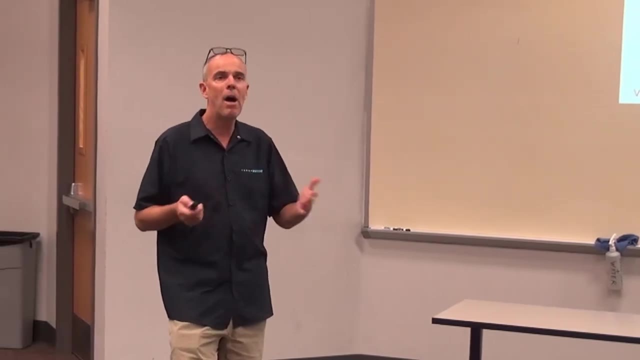 So they'll get a little more output, but not that much. So with our equipment generally, what we say is: one operator can keep 8 machines running for 24 hours in a single shift If they have a reasonable amount of support for other things like the daily maintenance of the machine, the cutting of the material, 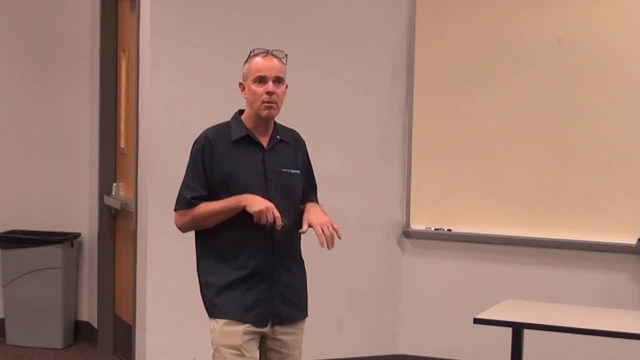 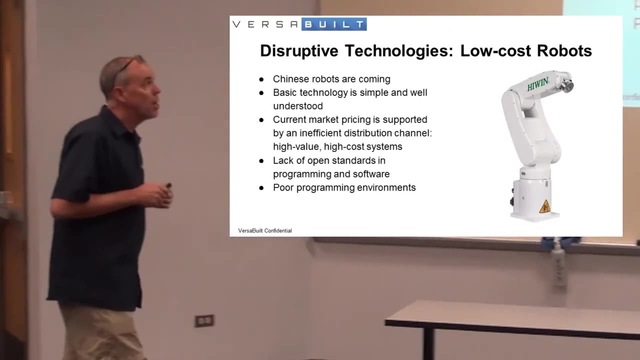 if all they're doing is tending the machine, changing tools, things like that, basic things, Alright. some other disruptive technologies, Low-cost robots, Chinese robots, are coming. This is actually a Taiwanese robot by a company by the name of Highway. 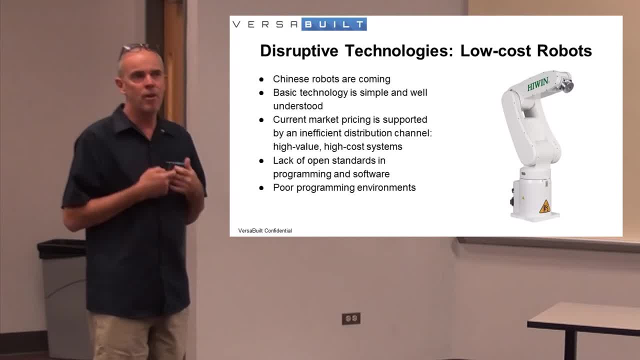 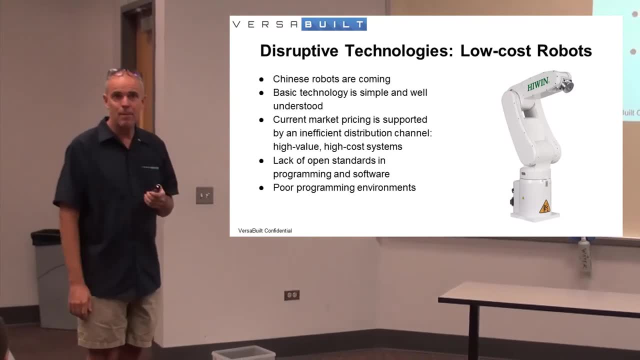 But the basic technology that robots use is very, very simple. It's very well understood. The program behind robots is amazing: the kinematics. I think you guys have a class now that you can take here in kinematics, But it's really well understood. It's not that expensive to develop. So current market pricing is supported by an inefficient distribution channel, the system integrator channel. These robots go into these very, very high-value applications where downtime is really expensive And that robot really isn't even that much of a total cost. 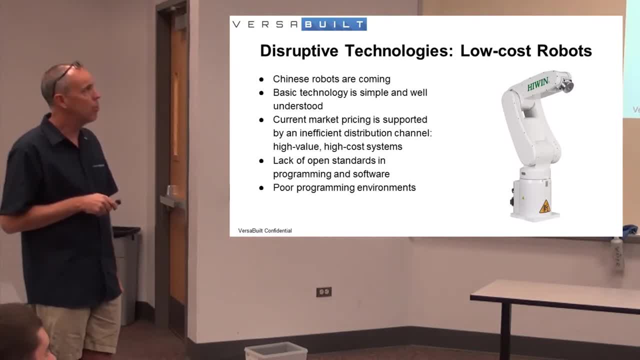 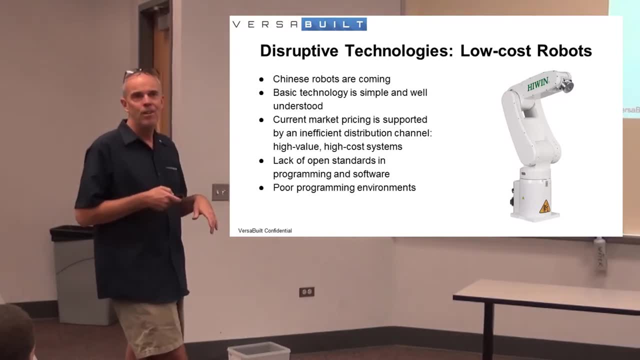 And it's primarily driven by a lack of open standards in programming and software. You need these kind of sophisticated tools to help you develop the applications, But they're coming from the vendor, so you get locked into that vendor. It's really that they can keep their prices high. 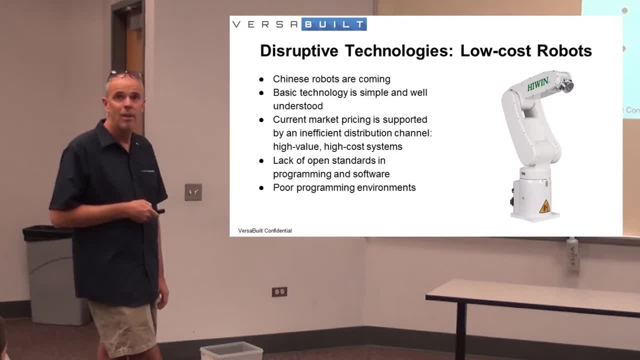 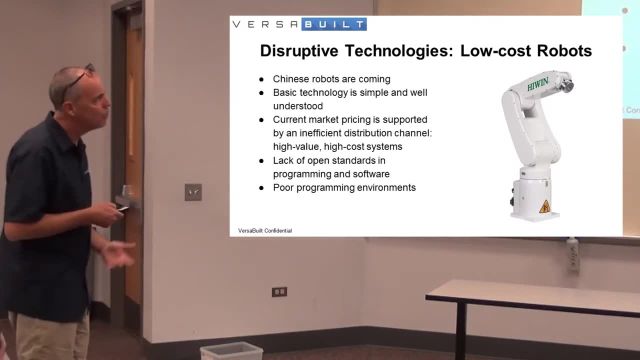 And really these programming environments. although they're pretty cool, they still they suck. As a software guy, they're terrible, They're really behind And primarily because they just have these small teams developing them, They don't have the benefit of the open source community. 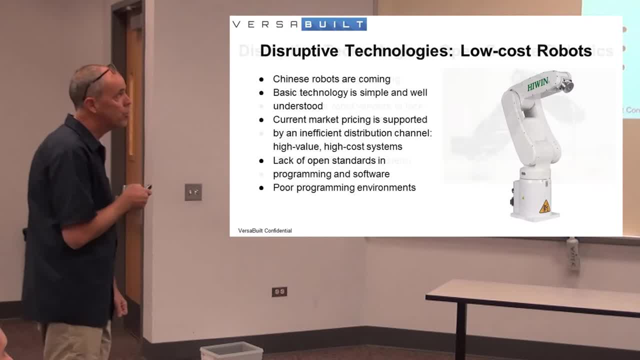 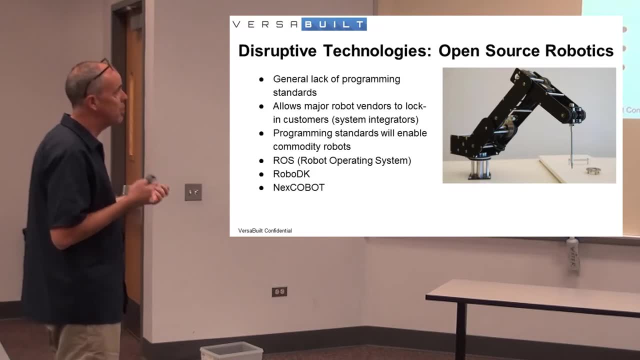 So what are some of the disruptive technologies? Open source robotics. Right now there's a general lack of programming standards. Open source robotics would allow major robot vendors, So they allow the major robot vendors to lock in the customers. Those programming standards will enable commodity robots. 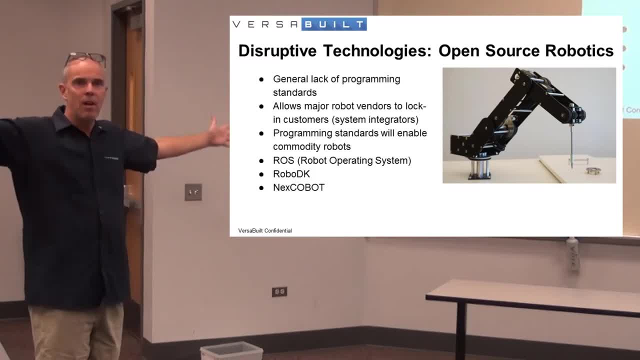 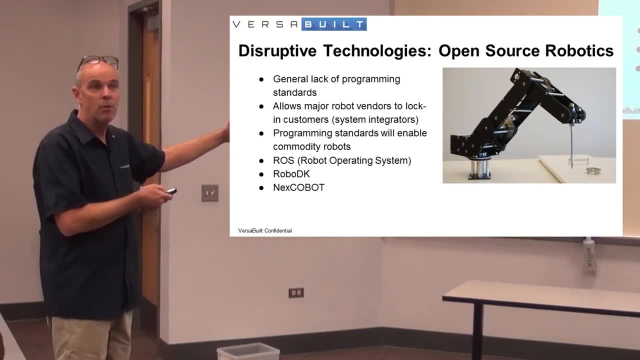 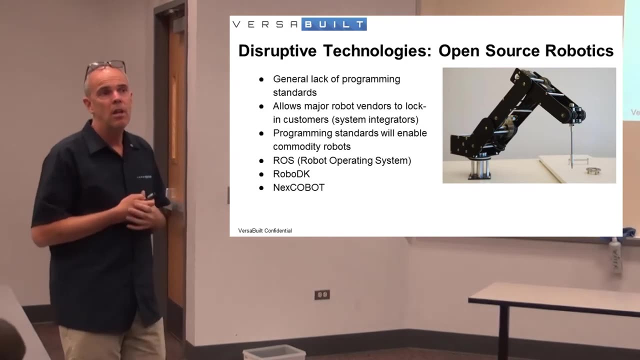 A little vendor from China can't afford to develop this massive application to be competitive in the market. But if a group of open source software developers do it or some company that will license that stuff relatively inexpensively, that will enable these producers of commodity parts. 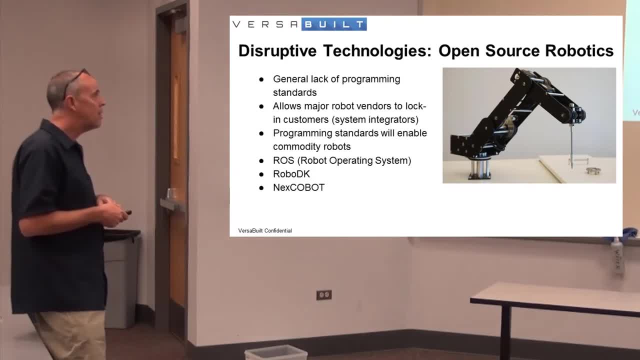 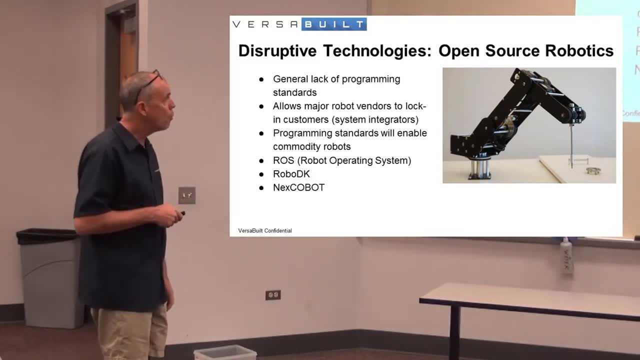 to bring the cost of robotics down. So some of the key things that are happening in there. Ross Robot Operating System has been around 10 years. It still doesn't have a tremendous amount of traction. RoboDK is a little bit newer. 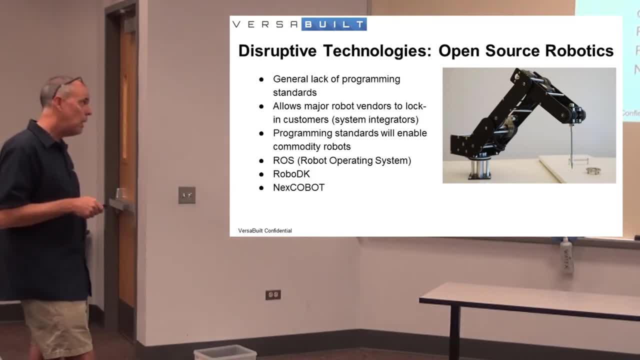 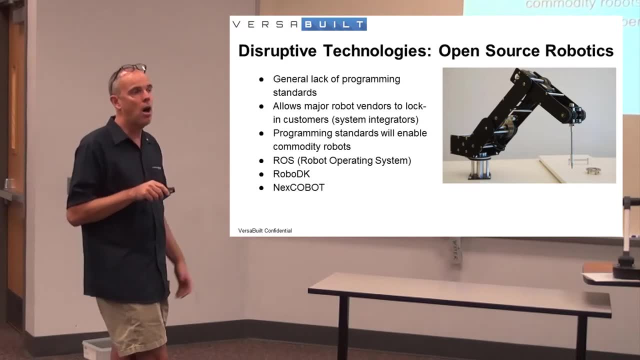 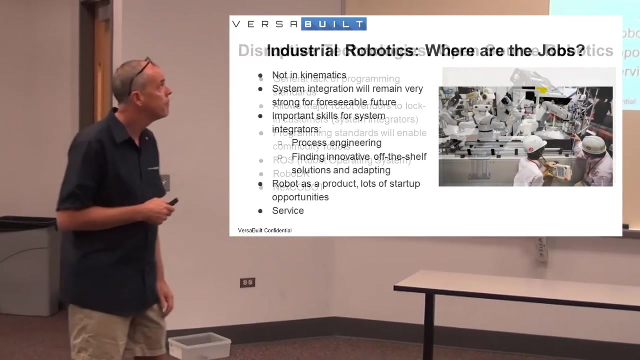 They're doing some really promising stuff And right here, I believe NextCobot is actually the only software company in the world today that is focused on being a software vendor of kinematics And the programming environments to really enable these third-party companies to produce commodity robots. 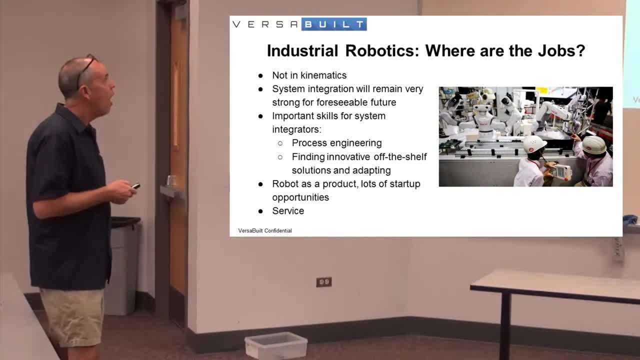 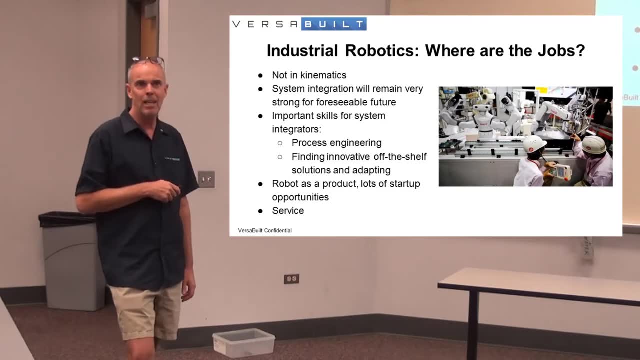 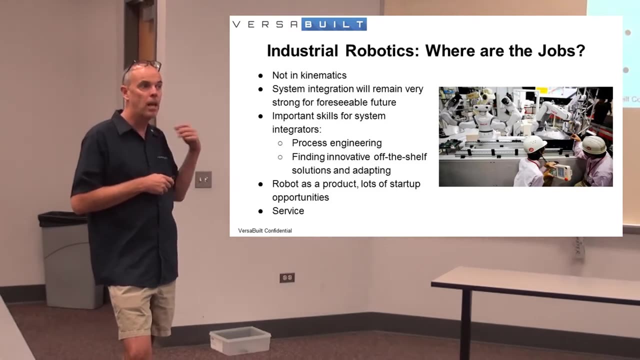 So thinking about Java Robotics, where are they? They are not in kinematics. This world needs maybe a couple hundred people in kinematics. It's been solved. There's not a lot left to do there Again if it goes open source. 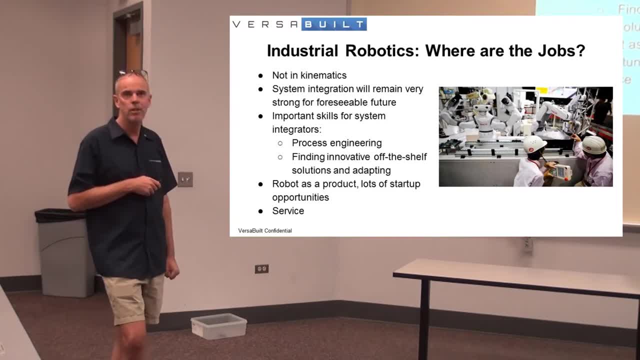 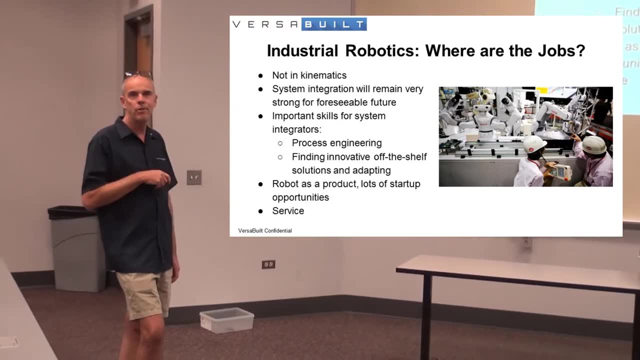 then a team of 10 really good software engineers could, in a couple of years' time, could create state-of-the-art kinematics. If you're developing applications, you don't really learn anything about how to actually control the motion of the robot. 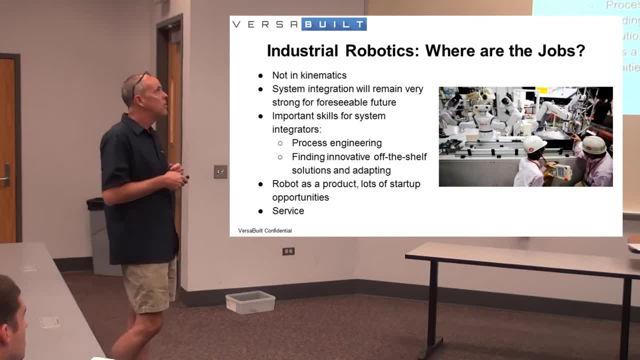 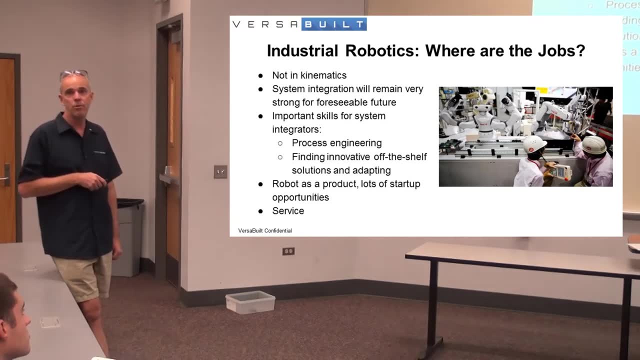 You're just telling the robot what to do. System integration, the kind of house of design work, kind of the traditional model, is going to remain very strong for the foreseeable future. There's still a very, very large market to fill there outside of automotive. 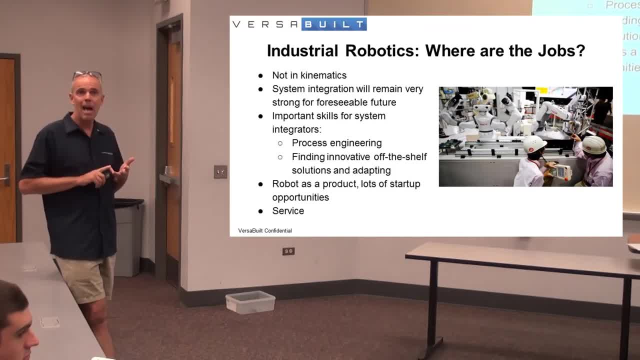 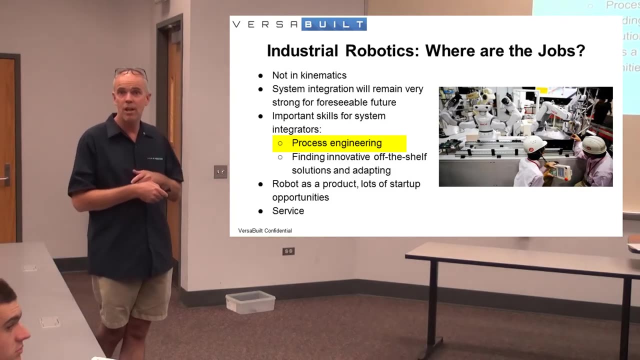 Of these high-volume, low-mix applications that people are currently doing, Some of the most important skills for system integrators are process engineering, Process engineering- Take classes in process engineering. Does BSU offer BSU process engineering classes today? Do a production engineering class? 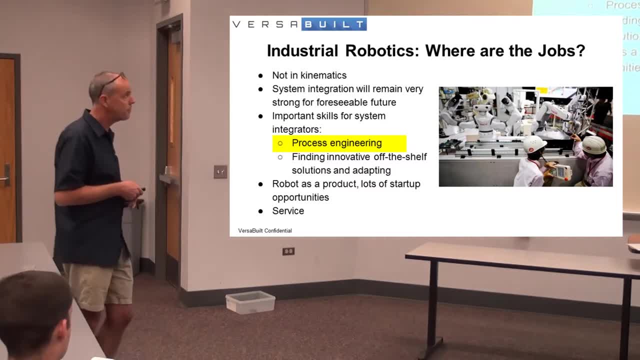 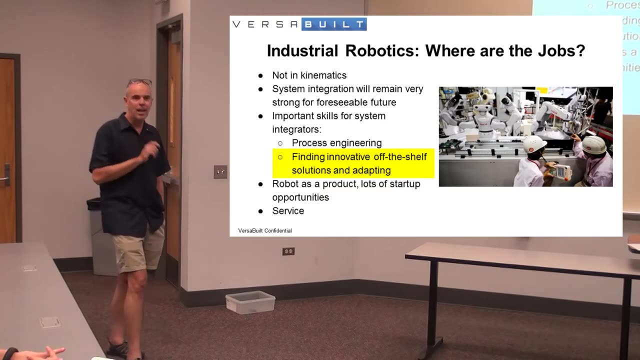 Next semester, Having the ability to go out and find innovative solutions and adapting, So going to trade shows, learning how to search on the internet, connecting with people. Hey, I've got this problem, Man. I don't know how to get this thing done. 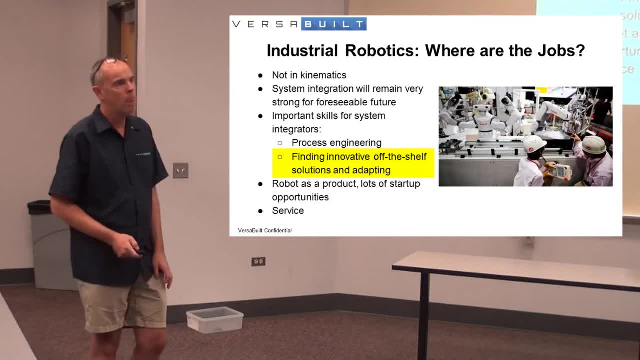 Oh, this guy, he's done that before. Go talk to him. There are thousands and thousands of solutions that are out there around automation, And often the most successful companies are not those that are that come up with the most innovative solution on their own. 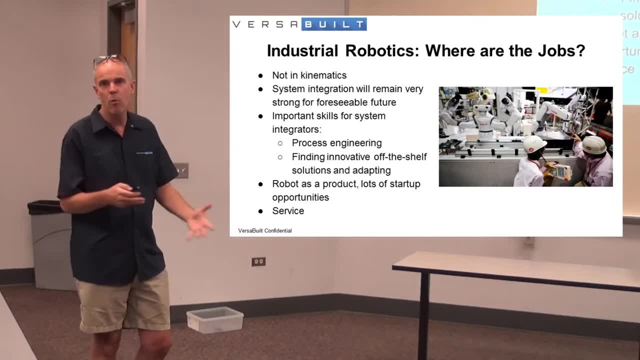 but they assemble other people's innovations into a working product- Robot as a product. Like I said, there are thousands of opportunities there And those are going to be startup companies right Where something like what I've been with RISC built. 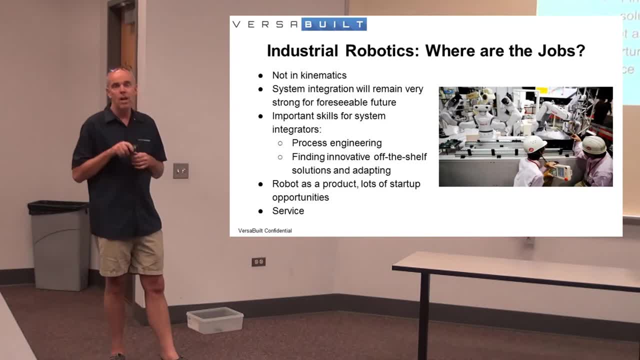 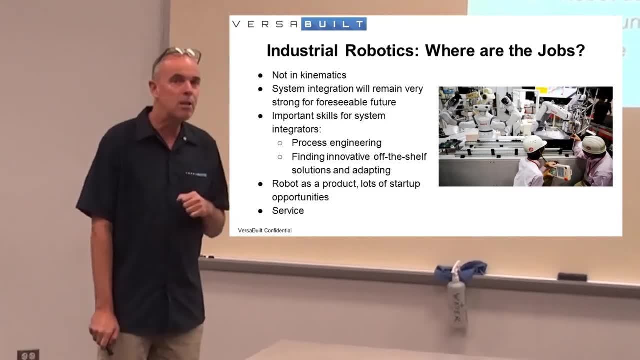 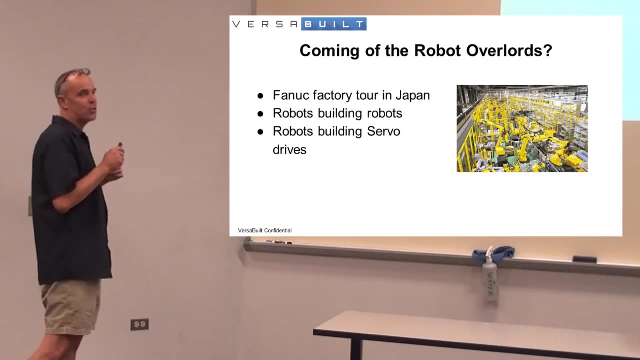 And then service Fixing robots- Right now primarily driven by the robot companies. Great opportunities out there for independent service Coming of the overlords. So I want to tell you just a really quick story. I know I'm running pretty close to my time limit here. 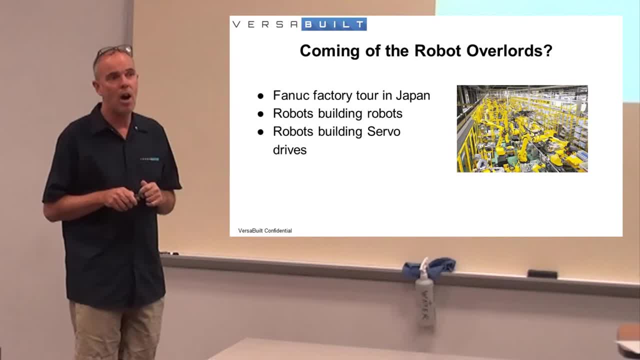 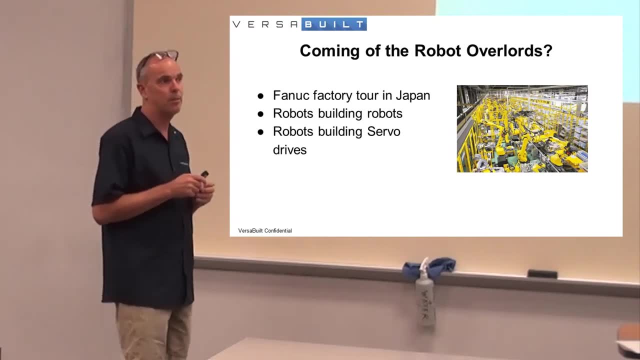 but not last April, but April before. I was very lucky and I got invited to do a factory tour of the FANUC factory FANUC takes about 15 people a year for this tour. They are a very, very secretive company. 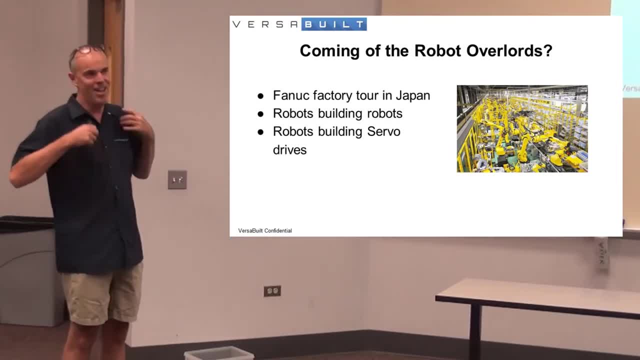 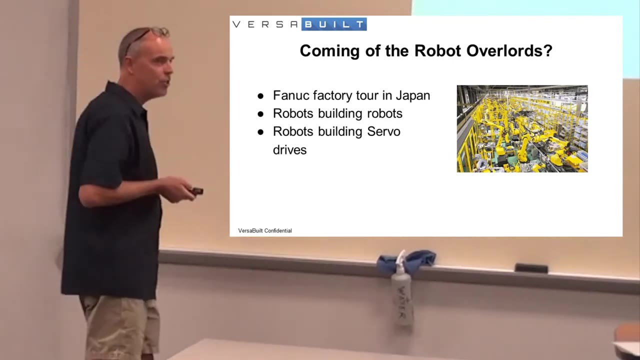 And they take your cell phone and they do a pat down to make sure you have no cameras And then you get to go see their factory Robots building robots. So the first building we go into probably twice as big as this building. 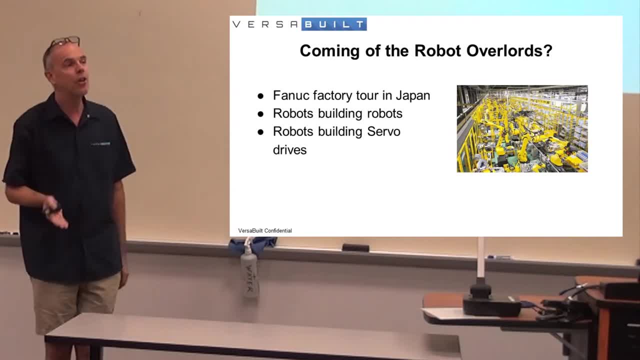 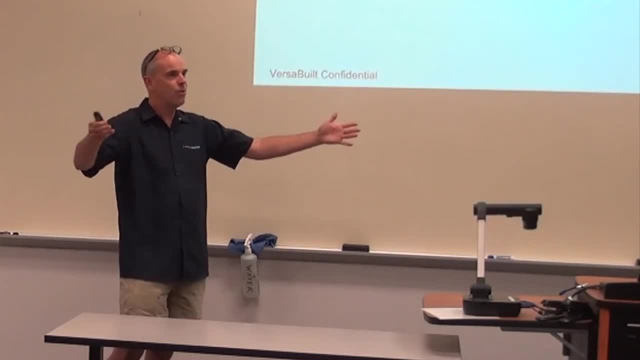 Four or five floors And they take us into the first floor And they turn on the lights. You can hear the noise as you come in. They turn on the lights And they take us over to you know where they have an actual setup. 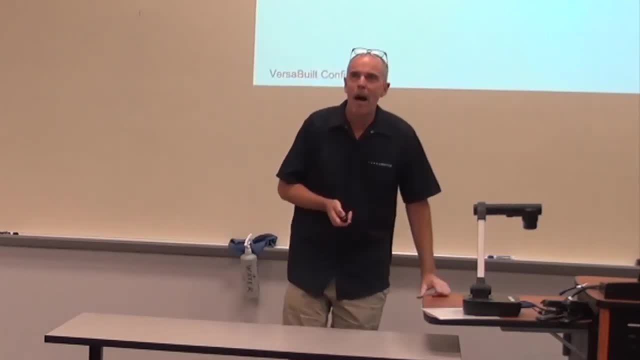 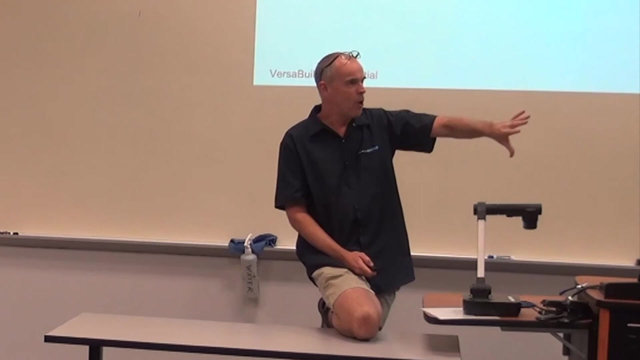 where people can look to see what's going on And there's about probably 15 robots that are building a robot And there's this incredibly large inky coming in And you can see the robots that are completed, that are being moved down through test. 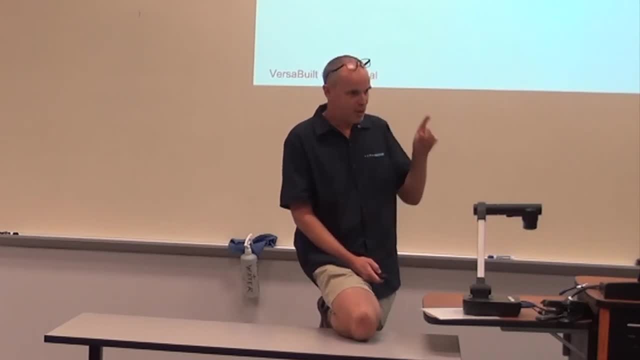 And when we left they turned back on off the lights. I think there was on each floor. there was four production lines. There was five floors. The in-feed for the building was 30 days, meaning that people could come in stock it with raw materials. 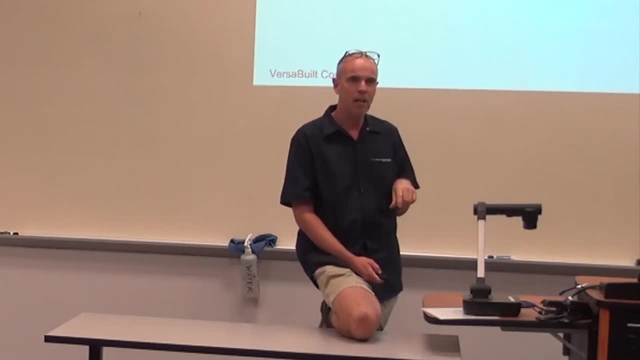 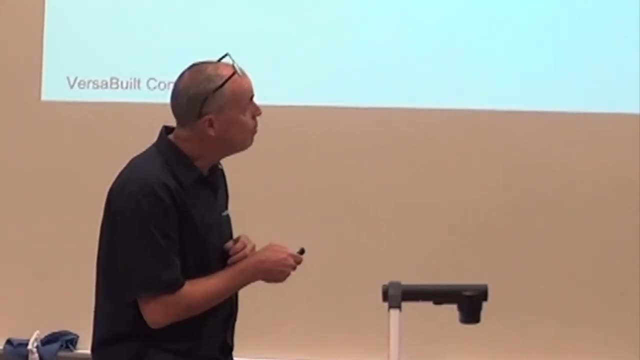 and that factory would run for 30 days making robots without anybody inside of it. The servo motor flying the little motors here. another building you know about twice the size of this building, five floors. They brought us into one little area. 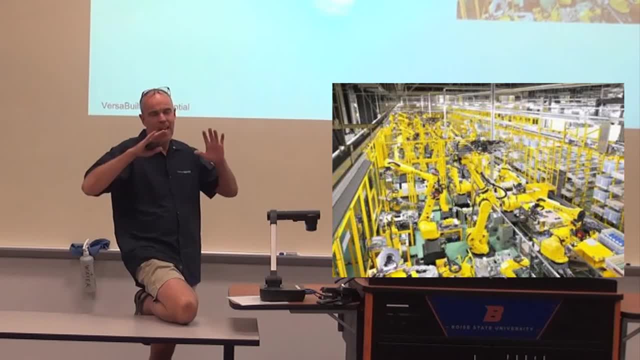 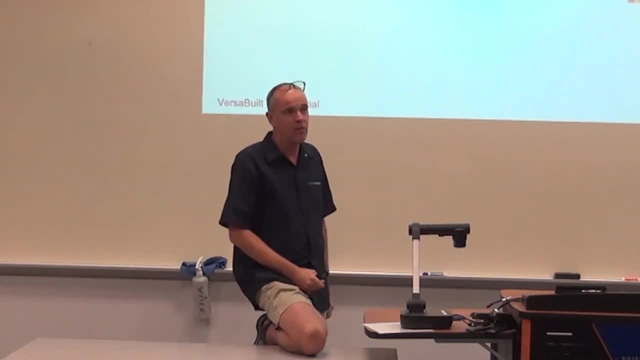 And they turned on the lights And there was a line in front of us. you know about the length of it, That's probably twice the length of this room, or one and a half times the length of the room, And probably 20 robots that were assembling. 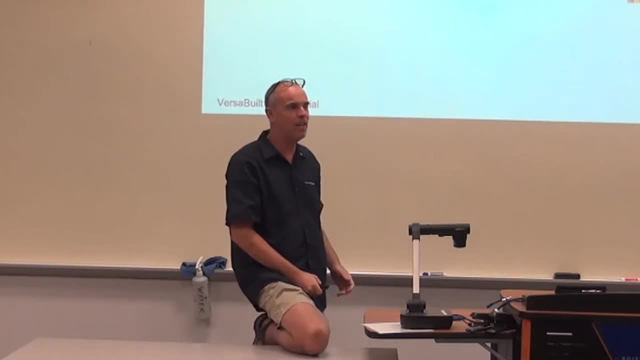 these servo motors together and then sending them out and completing them, And that was really impressive to watch. But the spookiest thing is you know they have glass there that you can see it, And then the room was about the width of this room. 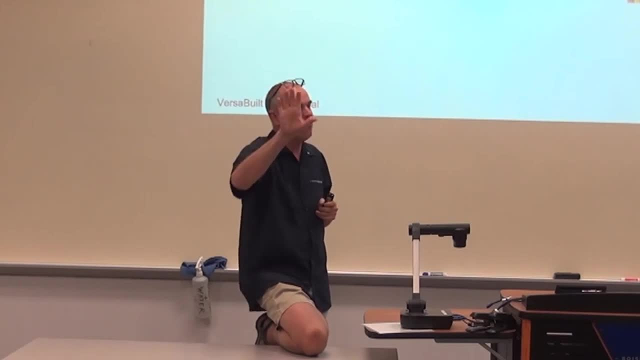 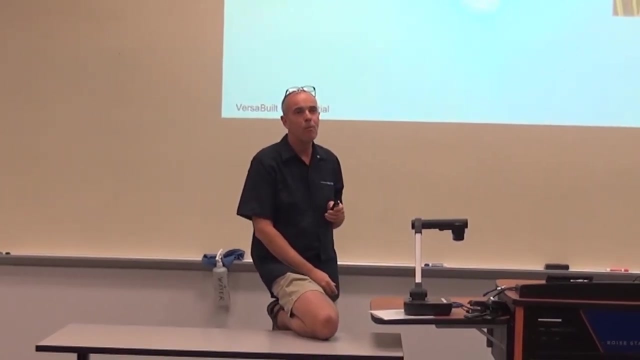 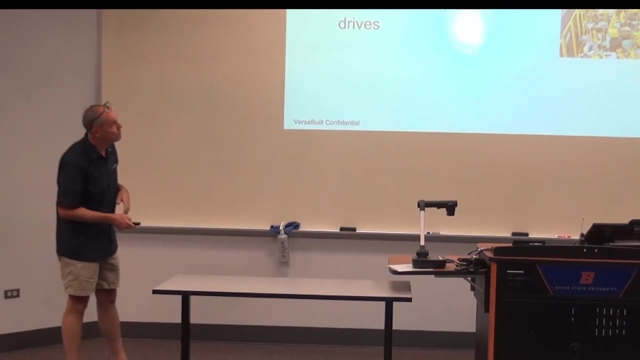 and then there's more glass and behind that you see another line and another line and another line. I think there was five lines deep and five stories of this And again about 30 days of inventory. It was really pretty remarkable And I think that's about it for my presentation. 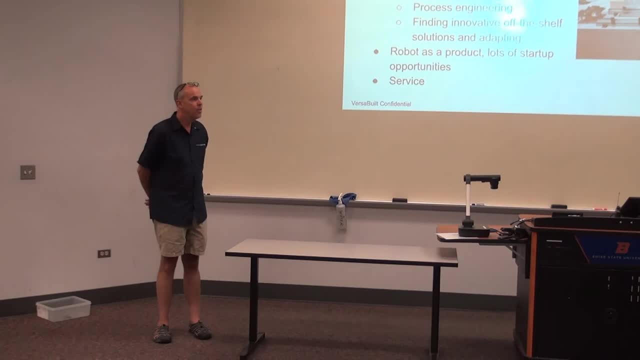 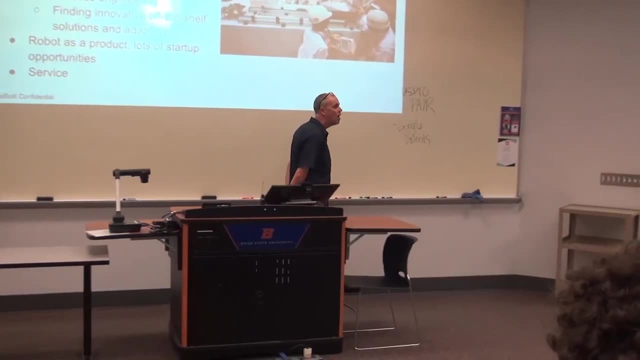 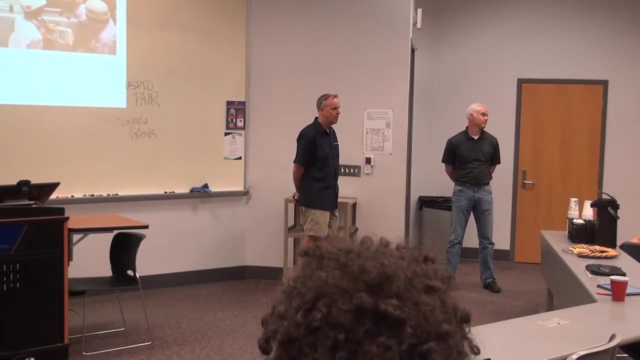 So any other questions? I've got a couple of them. One on the driving side: what does Recluse mean? What does it mean? You know the names, The name, Yeah. And then the other question is the cybersecurity issue of it. 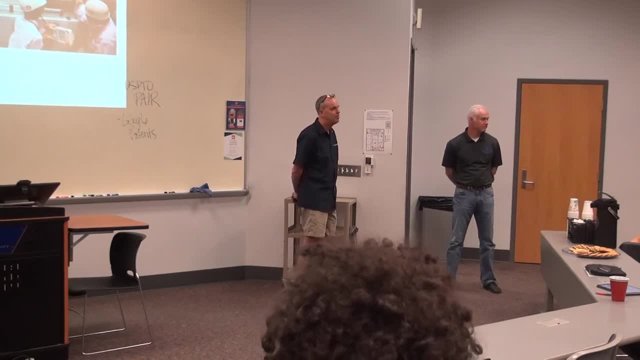 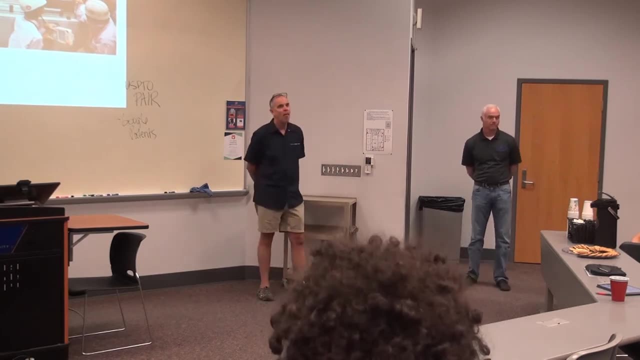 and how are you packing it within your company and then you sell these products elsewhere. Yeah, so great questions. So, Recluse, I was starting a company. I had a friend that was in marketing And I said, hey, figure out the branding for it. 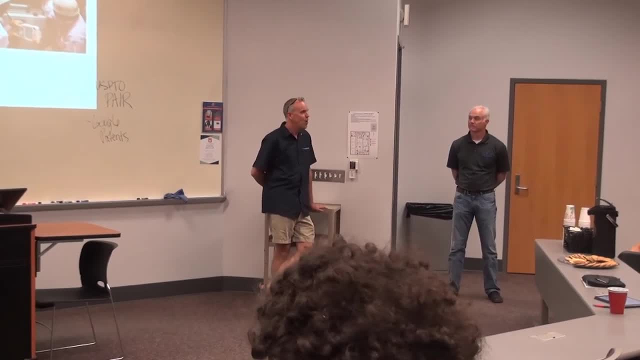 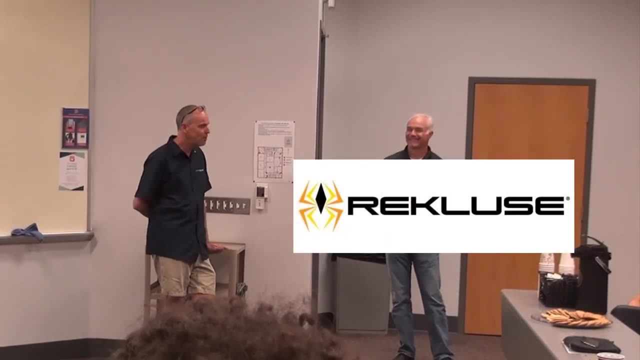 And he came back about a week later And he said: hey, what do you think about Recluse? And I said: huh, You mean like someone that's withdrawn? And he said: no, no, like the poisonous brown spider. 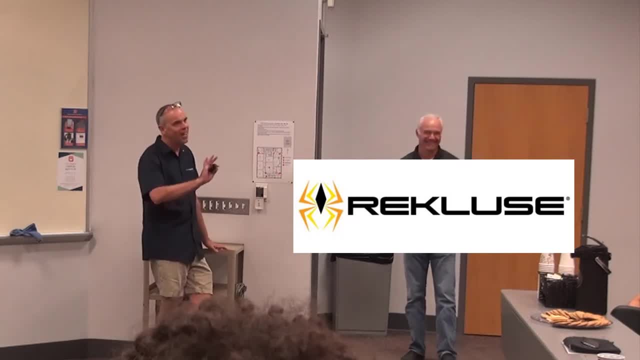 I'm like, oh yeah, that's way better. And I said I don't think so. And he goes: no, no, no, you've got to see the logo. And I came down and saw the logo And I kind of liked it. 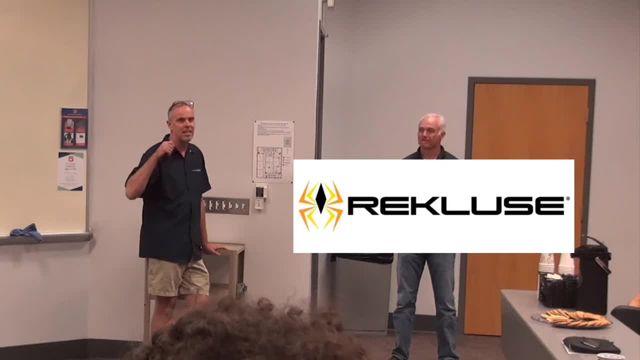 And I think it was a really good choice for us, Because one of the things it did is, when you hear that the first thing you do is stop and go, what the heck, What the heck? So it causes you to stop. 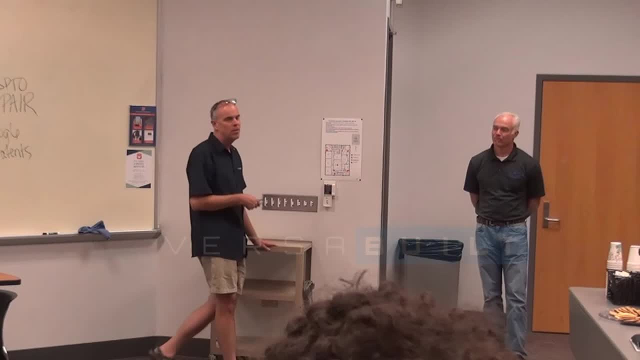 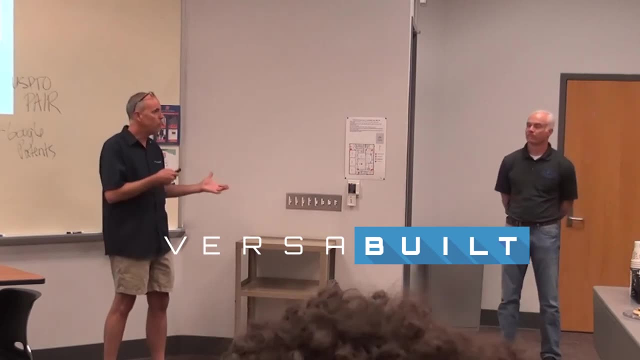 And then it builds a deeper impression. And then VersaBuilt kind of went through the same kind of thing. We had come up internally with VersaBuilt, You know versatile building of stuff. Didn't love it But got the same marketing guy. 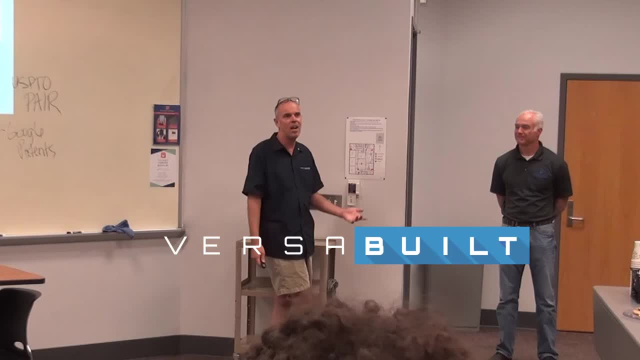 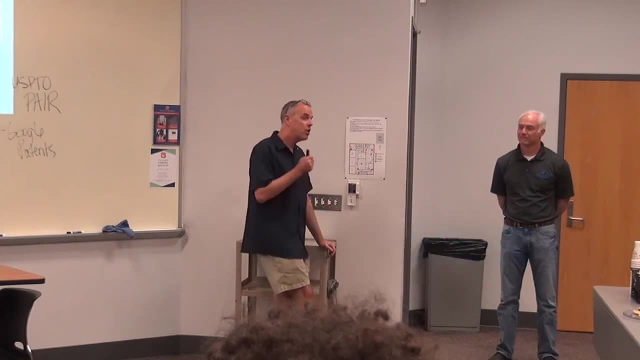 And he went through and his team went through And they came up with all kinds of different things And we all came back in the end and said, yeah, no, VersaBuilt's really the best thing. Cybersecurity- There's been some really good articles recently about this. 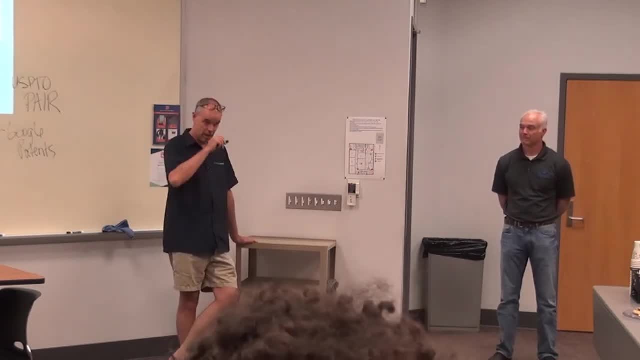 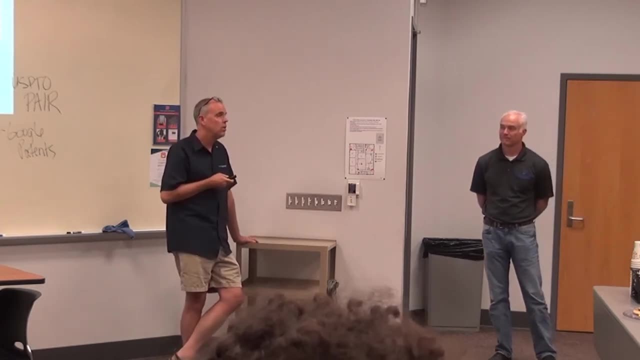 And if you're looking up a really good one. you can connect a robot to an internet connection. You can take control of it and do some pretty nasty things. We do connect our robots to the internet through Cradlepoint VPN, which is a local company. 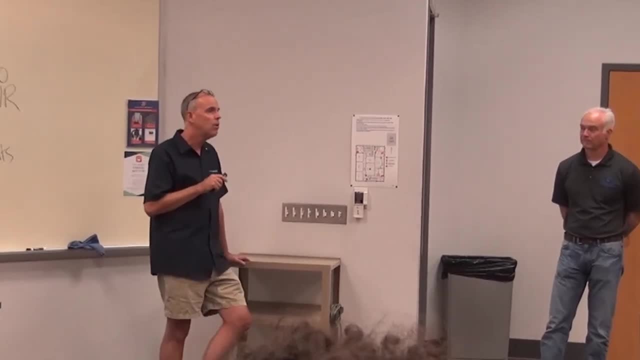 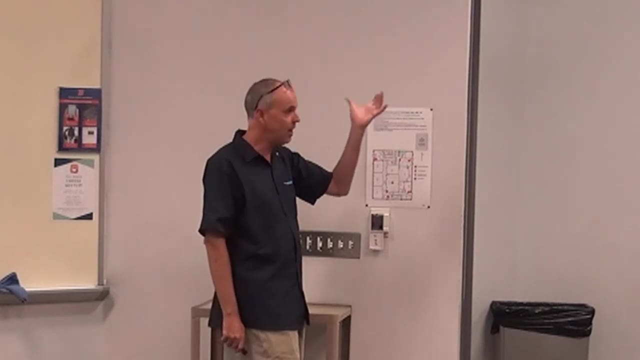 Because being able to connect to that robot remotely is incredibly valuable. We include a cheap $59 camera that we say to people: if this is going to look at anything that sensitive, tear it down. Hey, we're just going to point it at your machine. 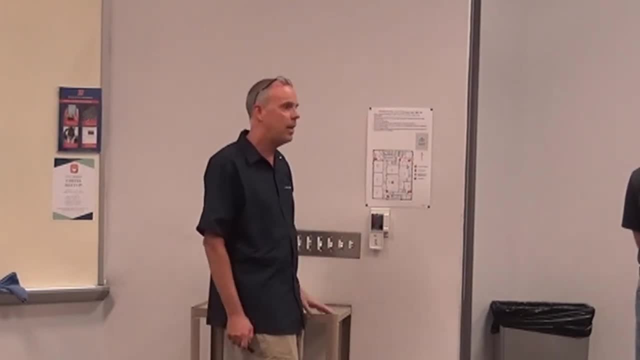 But these things are somewhat easily hackable And it is straight up not going to do that. But there's not a lot that malicious hackers are going to do with a camera. Again, most robots have safety systems, So probably the worst kind of damage. 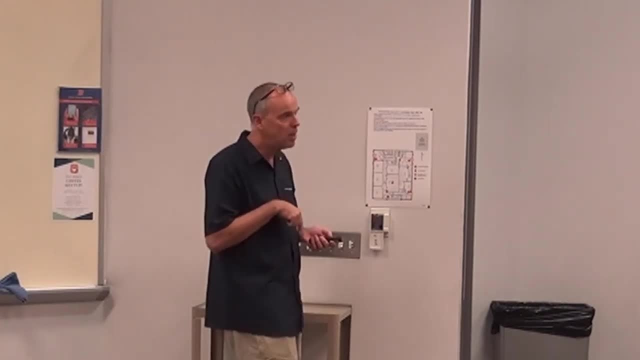 they're typically going to be able to do is not kill something, but maybe damage equipment, Even if you are operating a robot with a teach pen and it has what's called a dead man's switch where you can't have it all the way open. 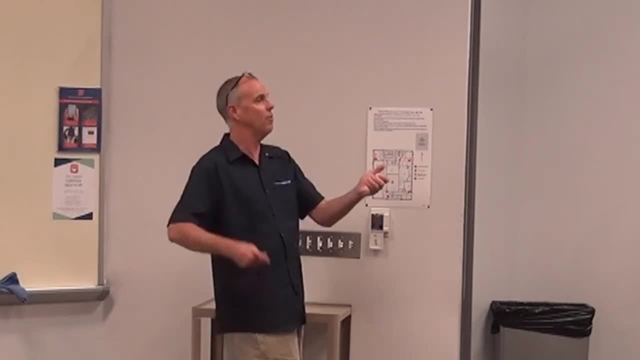 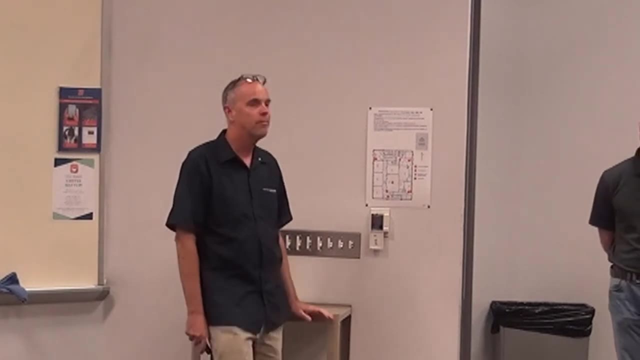 You can't have it all the way closed. You have to have it in the middle position. so if the robot does hit you and it's hurting you, you would squeeze harder and that would also shut it off. Any other questions? How long until you think robots are completely universal? 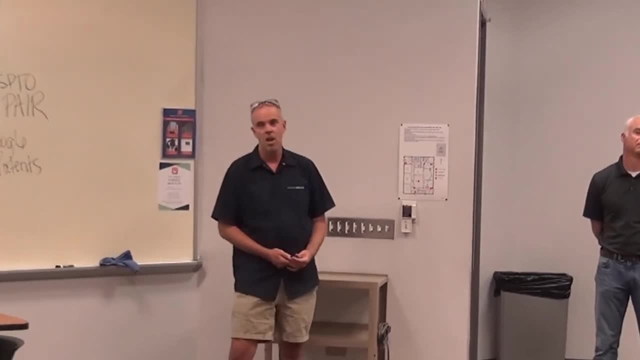 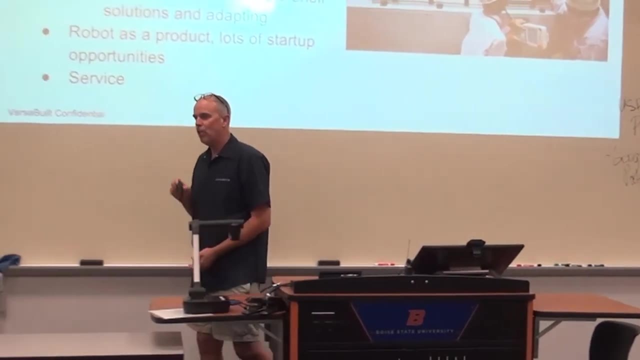 and human work is inexistent. You know that's a great question. There's a really good economist. I'm not sure where he's from, but he's kind of spoke at. I've seen him speak at BSU at least twice. 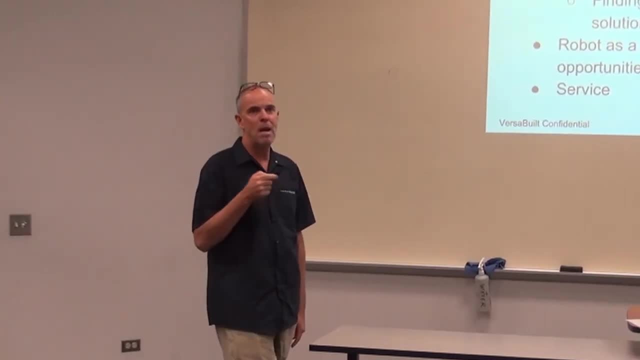 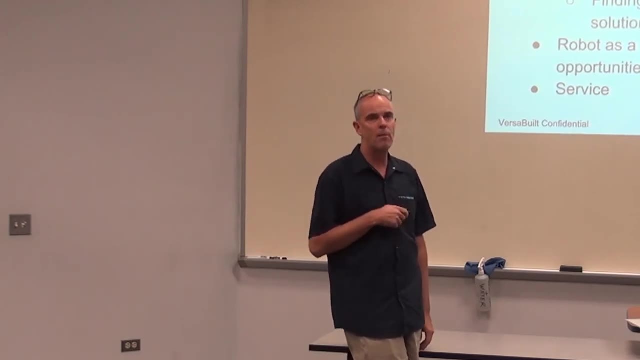 And a big part of this thing is one of the major economic trends right now is lack of enough skilled workforce, which people are not coming to us right now and saying, hey, we need to make our parts cheaper. They're coming to us saying: 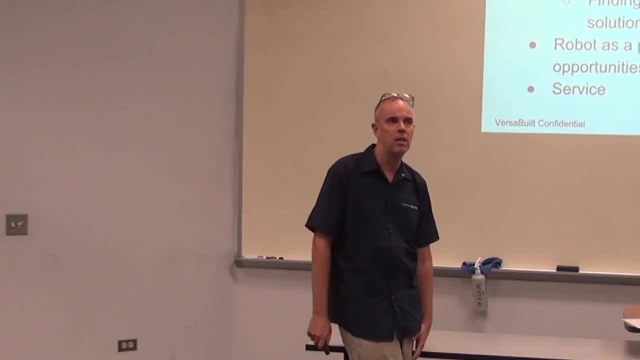 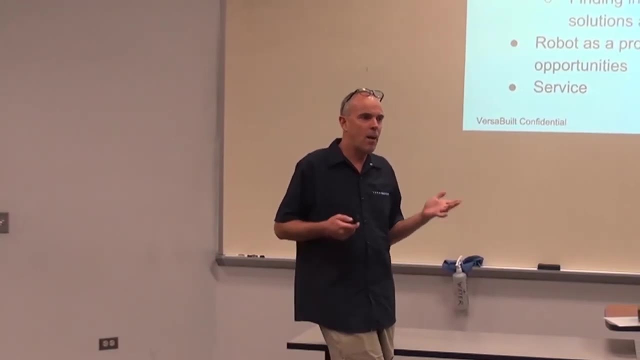 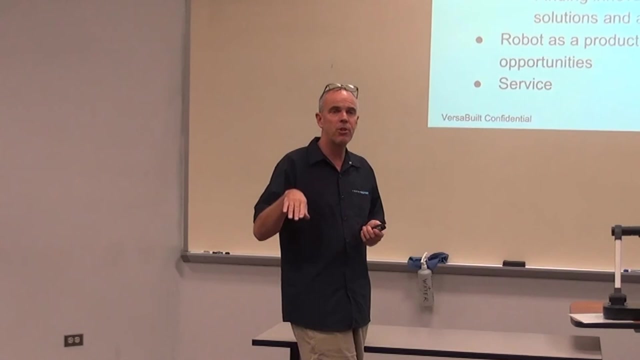 we can't hire enough people to get this done. So a lot of this is more of an economics theory question, I think, than a economics theorists. the pure ones would tell you that the tractor 1880, 50% of all employment in the United States. 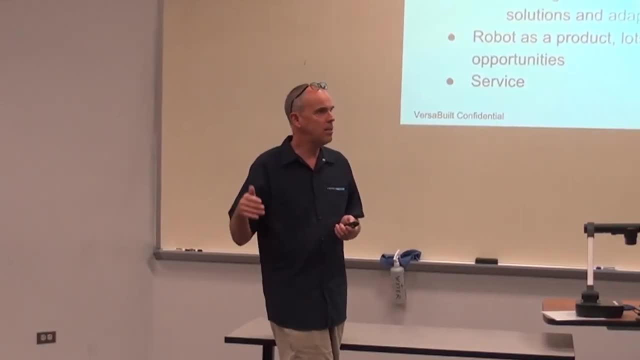 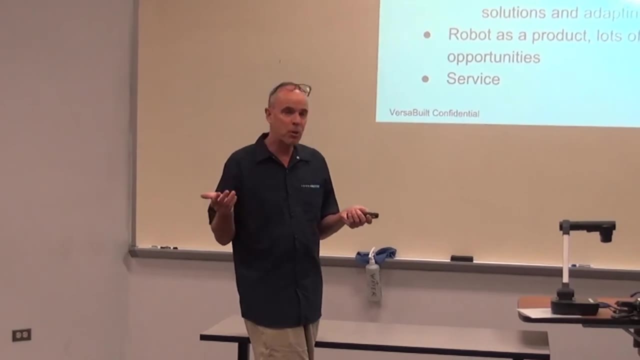 was agriculture. It's 15 years ago. it was about 7%, It's like 2.6%. All that is essentially. people call them tractors, but they're robots. Pivot irrigation is a robot, So do we want to go back to that? Probably not. Are we eventually going to run out of things? How much automation do we need to build before humans decide: ah, that's good enough, right? I don't need to. you know, I've got my Diet Pepsi. I've got my YouTube. 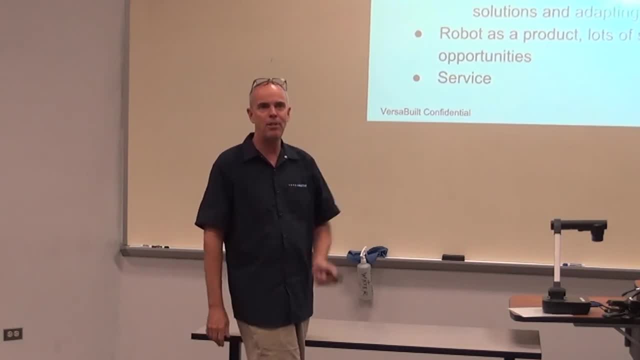 I've got my couch. the food's cheap, I don't need to do anything else. I don't know. I think that's. that's a really difficult question. I think it's way more about less about technology, but I think it's. 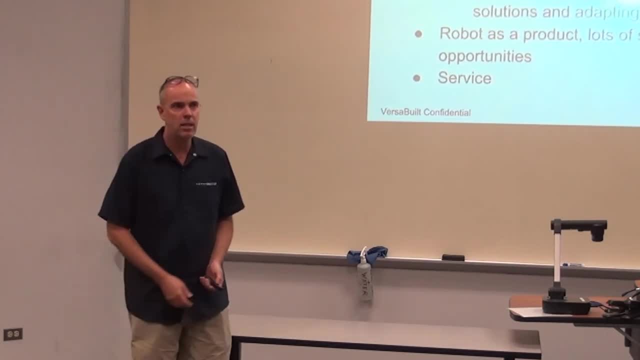 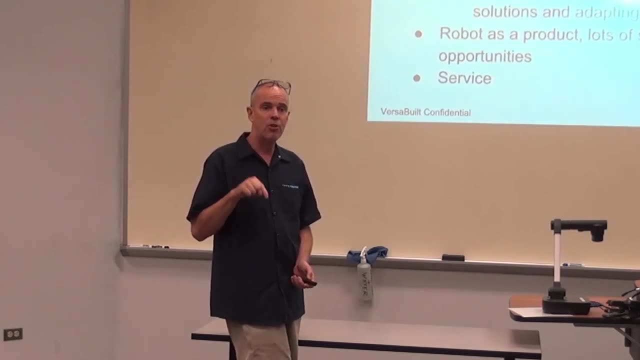